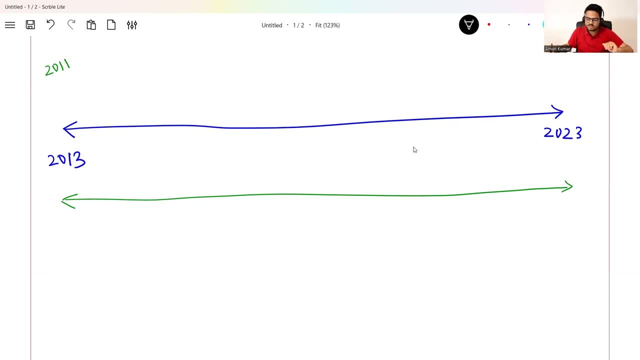 Things Okay. So in 2013, the time was so I will write here what the time was Okay, the time was off. I will write here some kind of n grams, Okay, n grams. All these are different, different techniques in the world of NLP. 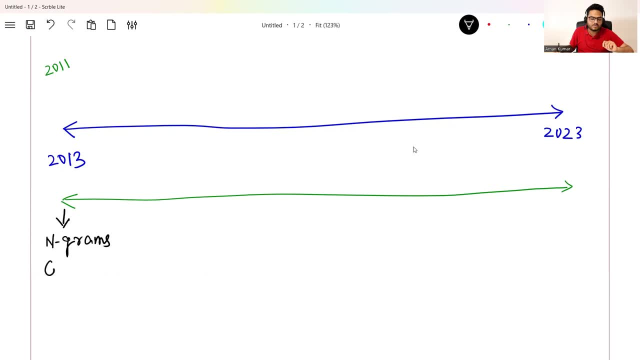 Okay, n grams, some kind of count based models- Okay, count based models- And some kind of word embedding also started coming in this era, 2013 and 2014.. Okay, then, I will explain you why these models were not sufficient. 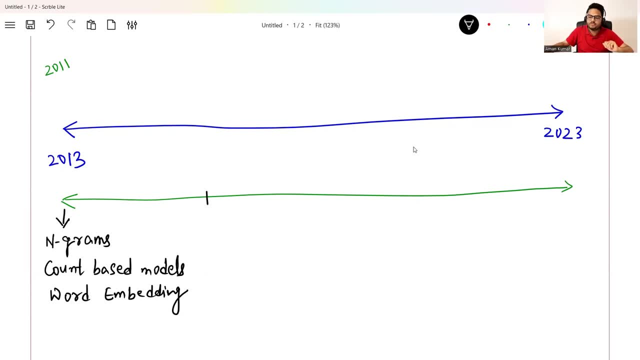 And then if you move around 2014- right, if you move around 2014- then two very, very big things happened in the world of NLP. one is known as recurrent neural network, RNN, and other is known as LSTM. Okay, The other version of you can say RNN or an advanced RNN. these two things brought a very 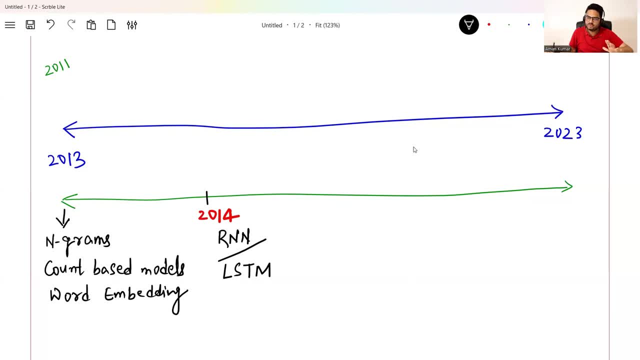 big breakthrough in the world of NLP. why? I will explain you slowly. we will go Okay. then I will explain you. what happened in 2015 is something came. a paper came. the name of that paper was: all you needed need is attention, Okay, and there was introduced something known as attention mechanism. 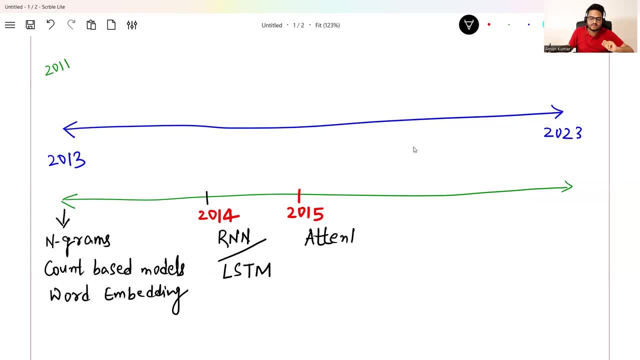 This attention mechanism changed the entire landscape of natural language processing. Okay, so remember these words, guys, which I'm writing here: attention mechanism. the paper came in 2015, if I'm not wrong, and this changed the entire world of a natural language processing. after that, everything took all together: a new route, a new, you know- pathway after 2015. 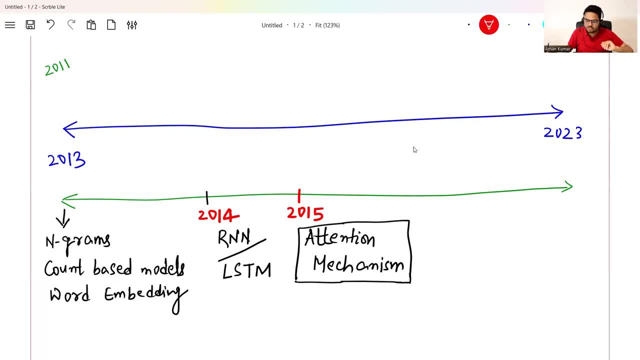 if we move little further right in 2017, two important things happened in the world of NLP. Okay, one is known as transformers. Okay, transformers is one kind of architecture based on which many new things are developed, and other important thing that happened in 2018.. 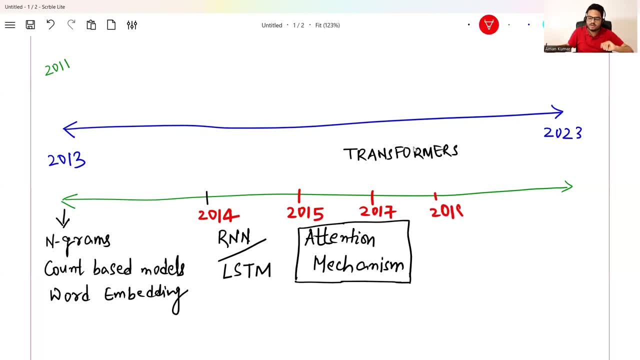 I will just write here: 2018, and this is known as something similar to transformer, but not exactly Transformer, but okay, another kind of model. and as you move to 2020 and 2023- all of you know this is the era of GPT based models and large language models- is the most new. 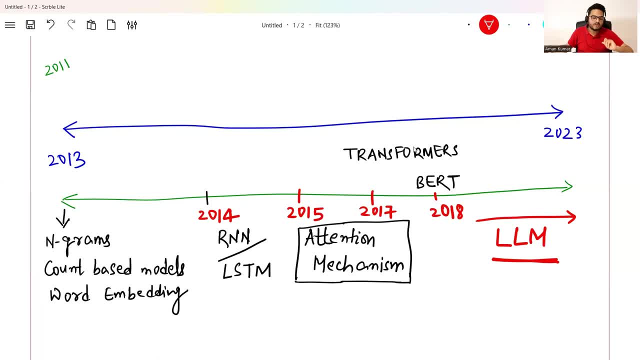 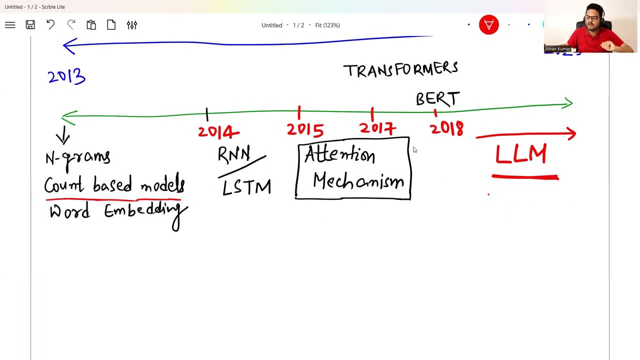 thing that we are seeing in 2023.. So, guys, we started from some count based models, which I will explain you now, and we reach to LLM, large language models, Okay. So I'm going to take one simple, Okay, One simple use case and try to explain you how things have evolved in the world of NLP. 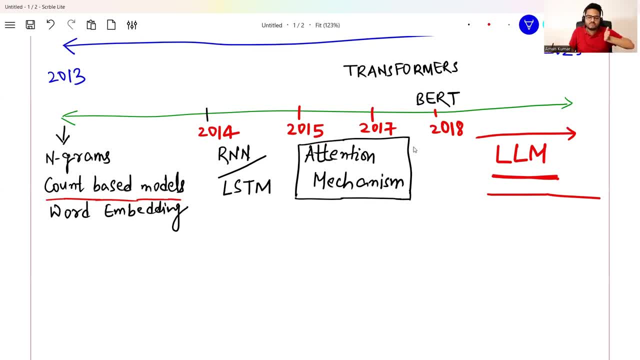 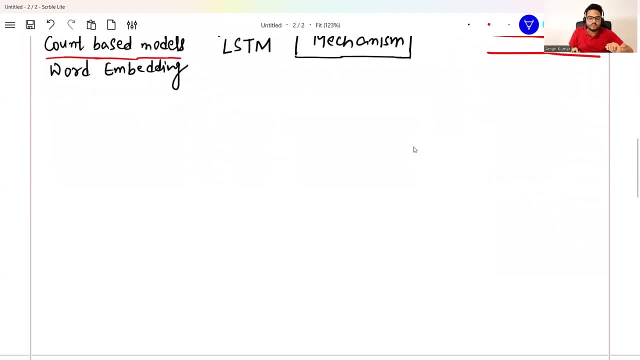 if you understand this right, then it will be very easy for you to digest the advanced concepts and how things have moved. Okay, Now few things here. whenever I say NLP, right, NLP stands for natural language processing. in natural language processing There can be text data. 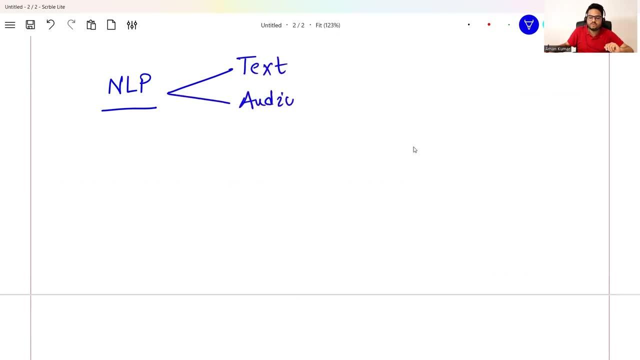 There can be audio data, There can be video data, There can be image data. Okay, audio video image. These kind of data can be there and you know, different kinds of use cases can be there. So, needless to mention some of the use cases which you can see of NLP in day-to-day practices, 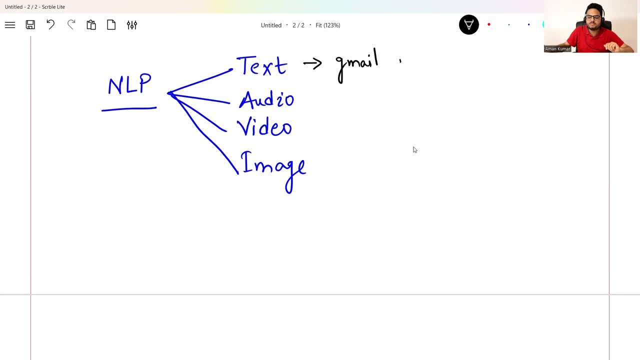 For example, Gmail autocomplete feature. I'm sure all of you would be using this. So when you start writing any email in Gmail, it will automatically autocomplete. right, That is one feature. then you will see some kind of audio to text or text to audio kind. 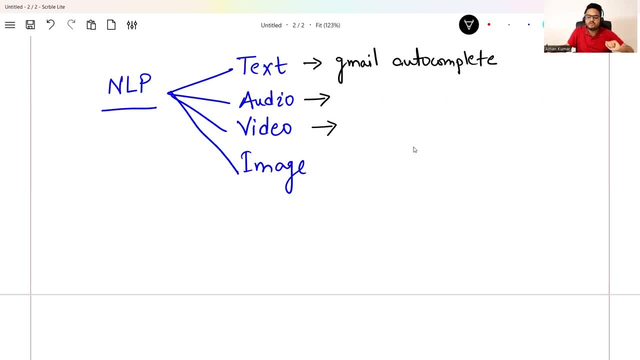 of AWS gives you those kind of devices. in video, You can see many applications of video analytics right. So many of these things fall under the category of NLP. We will focus more on text-based NLP. The reason for that is in market. 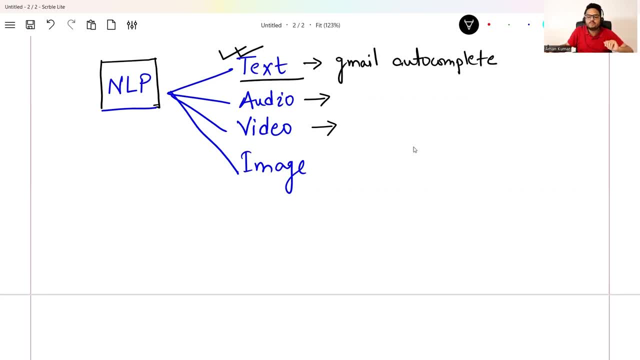 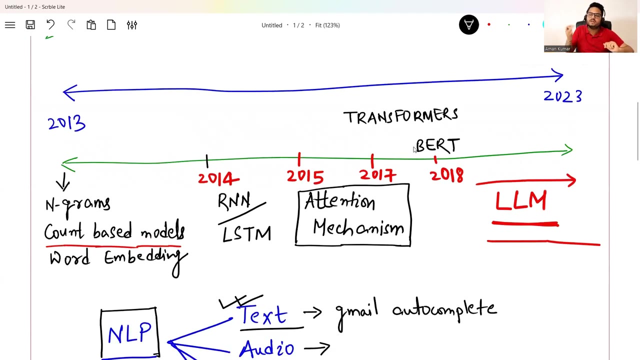 Most of the use cases that we use, and most probably you will be working, will be text-based. fine. Having said that, let's take a simple test Best use case and try to understand how this use case would have been solved using different techniques and how this will be solved using RNN. 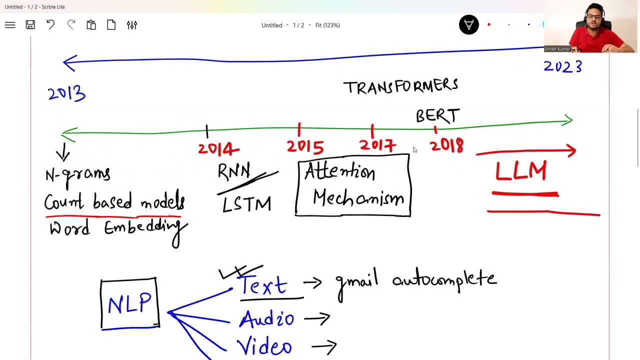 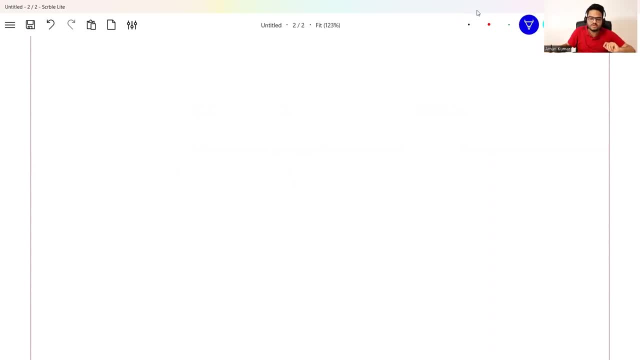 Okay, so I will just explain you how this would have been solved using various techniques before suppose. suppose I try to sentence here. Okay, my first sentence is: I am, I am playing. I am playing cricket. This is my first sentence. My second sentence is: he is playing. 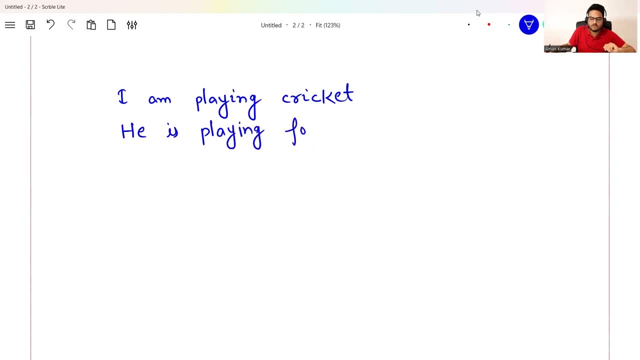 He is playing football. Okay, I take these two sentences Now. suppose these two sentence is my entire training data. Suppose this is my entire training data And what I want to do is I have a level against this. Okay, so I have a target variable. 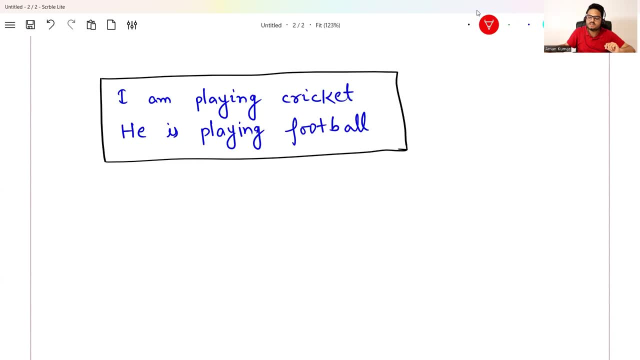 This is a supervised problem. So if this sentence is a sentence related to cricket, then class should be one. otherwise class should be zero. So this is my problem statement. Okay, this is my problem statement. So tomorrow, if I write a new sentence here, for example, I write here: cricket is good. 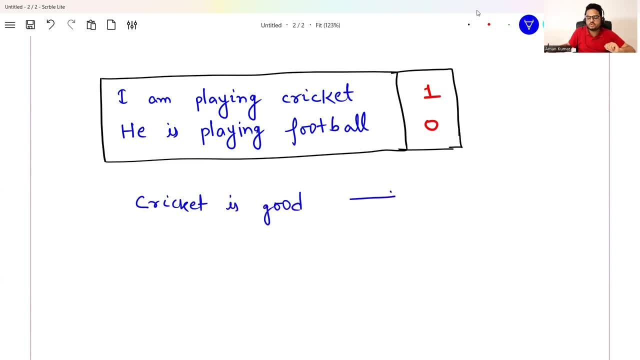 Just an example I'm giving. then my model should be able to predict this falls in the category of one or zero. So this is a classification problem simple. to make it simple, You can think of sentiment classification or any other model which tells whether this 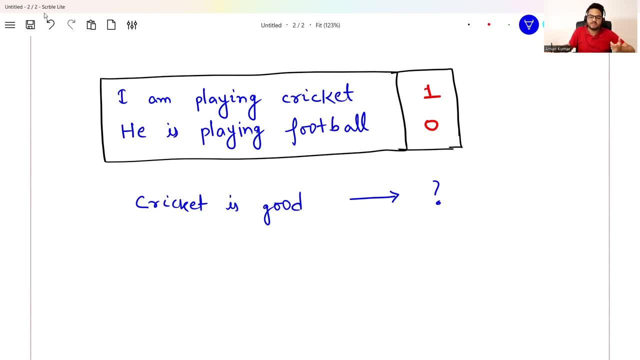 is a positive sentiment or negative sentiment. I am taking these two because people are very easily able to relate with games. Okay, so these are two sentences in front of you and you have to use to train your model. Now let's understand how people used to do this. 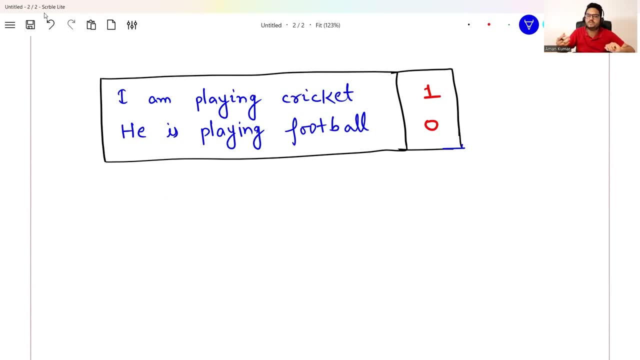 Back in 2013 and 14.. Okay, before that, let's understand few basic stuff about NLP or text data. So I will be using some term known as document, document and another term I will use known as corpus. So don't confuse between these two words, guys: document and corpus. in this scenario, each 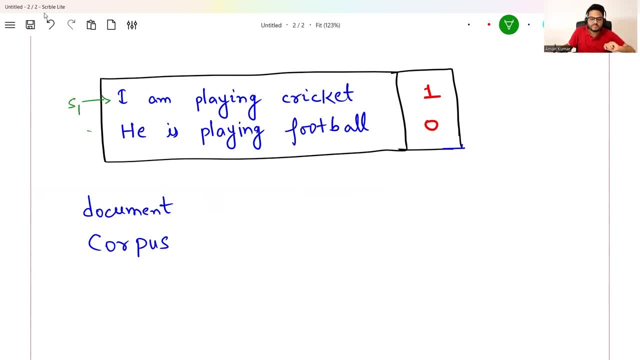 of these sentences, for example sentence one and sentence, So both these sentences are one word, One document: Okay, in this particular use case. suppose tomorrow you are working on a use case where there are 100 PDF files, for example PDF one, Okay, so on and so forth. 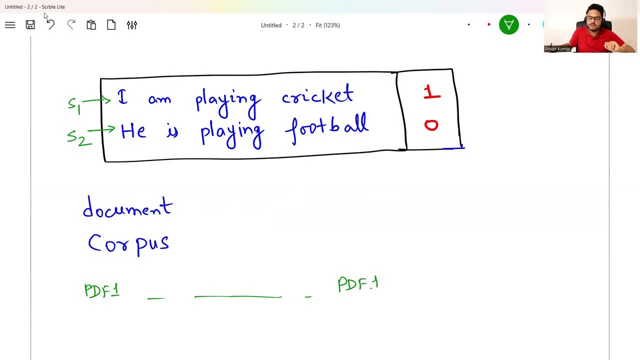 Let's say you have 100 PDF files. So all these PDF files is one, one document for you. This is first document, PDF to each second document and this is your hundredth document. So every time somebody tells a document, you should understand that this person is talking. 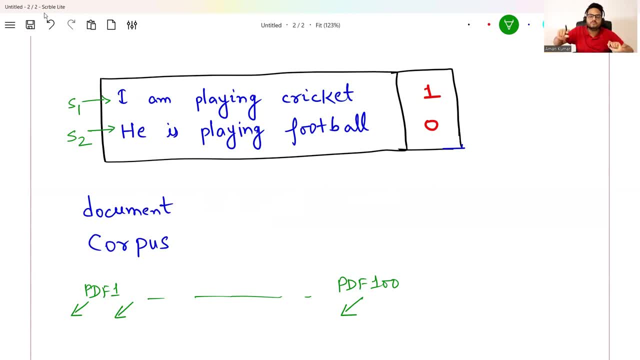 about one particular record Or one particular observation. Okay, so understand document like that And somebody talks about corpus corpus is a combination of all your documents. So in my case, what will be corpus corpus is all these document together. So if you, if you combine these two sentences together, what you get is your corpus corpus. 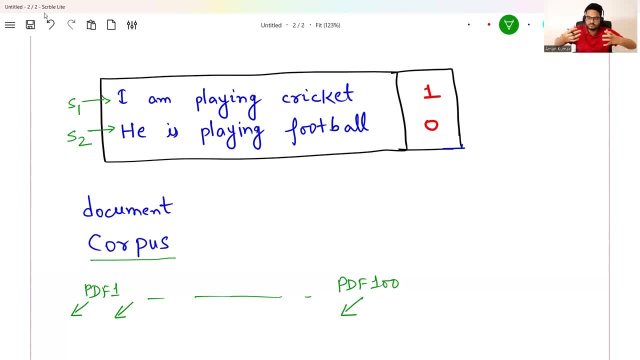 means everything that is there in your use case and here. if you combine all these hundred documents, what you get is your corpus. So please be clear on what is a document And what is a corpus, and keep in mind these two sentences. What is the use case? 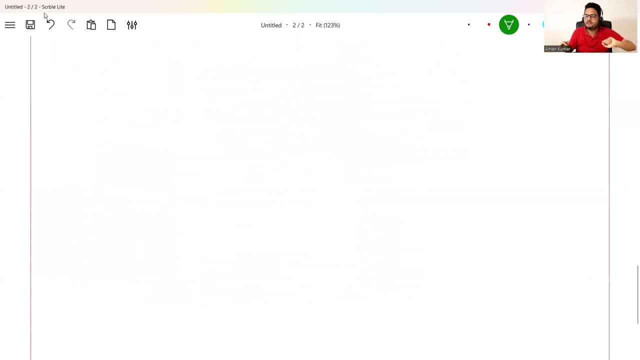 You have to classify a new sentence based on that analysis. Okay, So, as all of you know, I was telling you, NLP will take text data, input date, audio data, video data, image data and many kind of data. but one thing we must understand: all the machine. 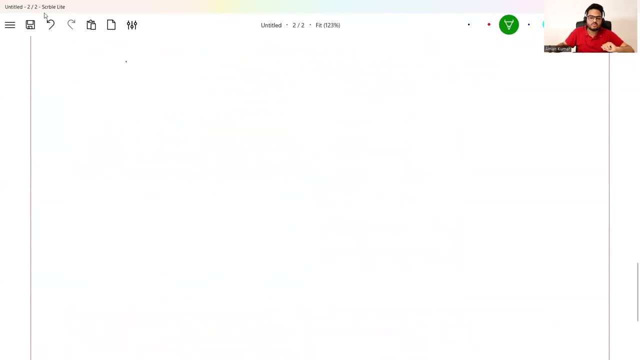 learning models or deep learning models, will expect what numbers? it will not expect any kind of image or text Or video. Okay, it will work on numbers. Okay, so your job, first job, is to somehow convert this training information into numbers. How would you do that? 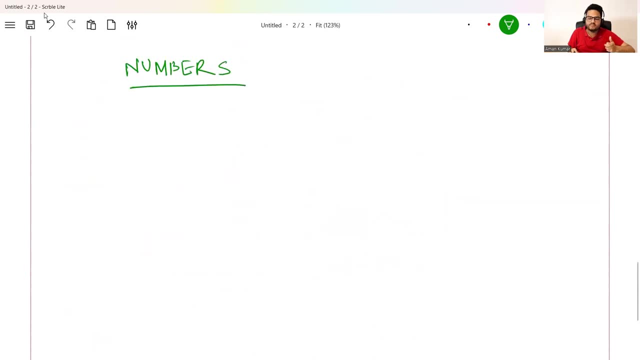 The most basic way of doing that is just see how many words are there in your corpus. Now note: here I am saying corpus, So how many words are there? If I take those two sentences and I start writing here, I is one word. 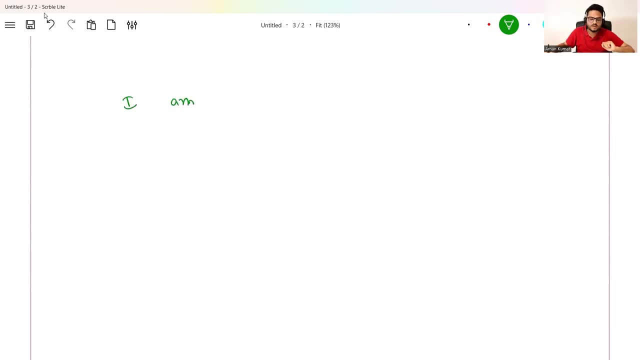 Okay, M is another word. The- all the words that is there in your corpus. I'm writing: Okay, Playing is another word. Cricket is another word. Okay, He is another word. Ignore the. okay, I will write like this: 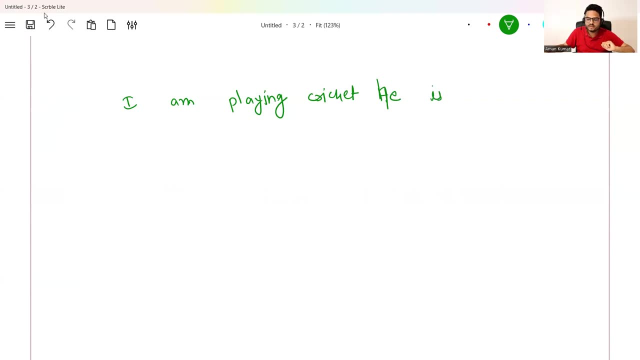 Imagine: everything is lowercase, only He is, and then I will write: football, Okay, Football. So If this is the word, this is the entire corpus in front of you, Right? Then what I'm going to do is I'm going to write as index here: 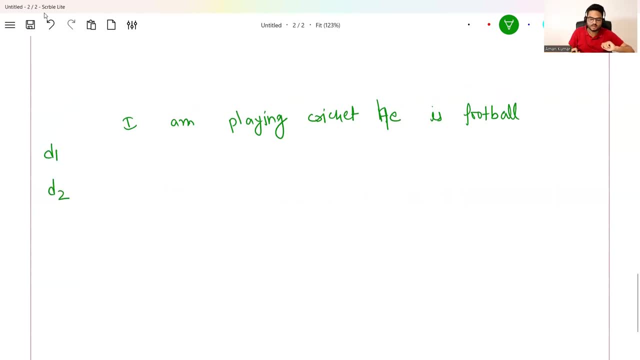 My document one and my document two. Okay, come here and see the word I is present in your first document, or not present? So I will make this one the word M. Let me take it in a different color so that it's easily you can understand. this is present. 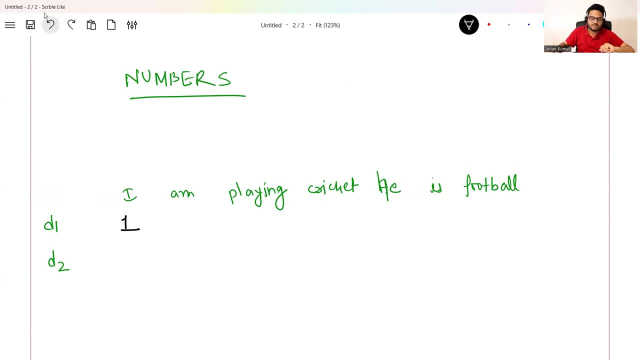 So I will make this one. M is present, I will make. sorry, This will also be one because M is present. Okay, Playing is present. I will make this one. Cricket is present? I'll make this one. He is not present. 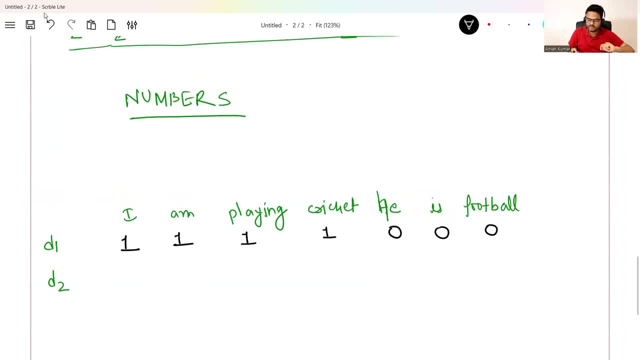 Zero is not present. Zero, football is not present. Zero, Okay, And I will come here and he is playing. football is my second word. So playing will be one, football will be one, He will be one and is will be one. This will be zero. 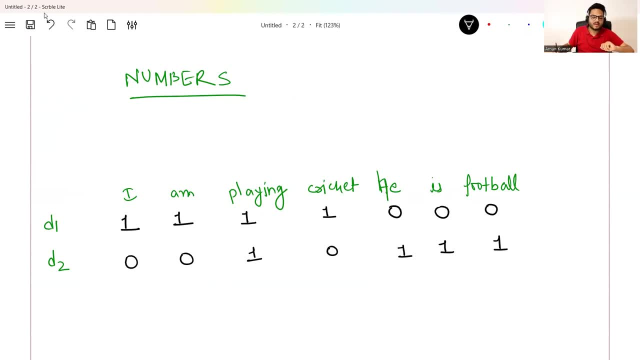 This will be zero and this will be zero Now. Why I am explaining you in this detail is try to understand how people try to convert sentences to numbers back then, 10 years back, and use that in their classification model. Now this becomes your individual feature. 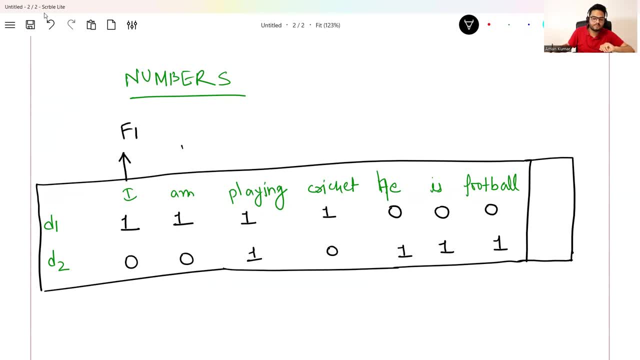 So, for example, this is your feature one, This is your feature two, And so on and so forth. and here becomes your target variable. So first is your cricket, So this will become one. Second is your football, So this will become zero. 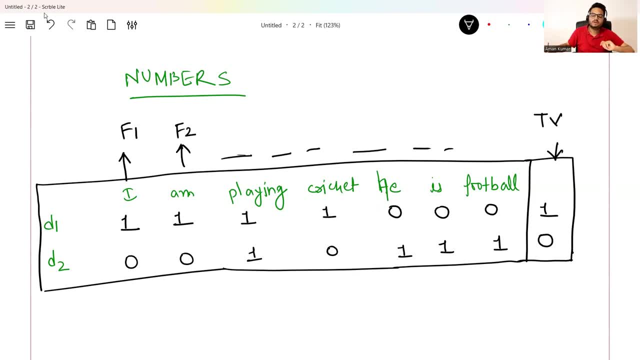 So this is your target variable. Now this becomes your complete classification problem. You can train your data on this most basic approach, most fundamental approach that was used like way back. Okay, just to give you a conceptual understanding of what used to happen back then and this: 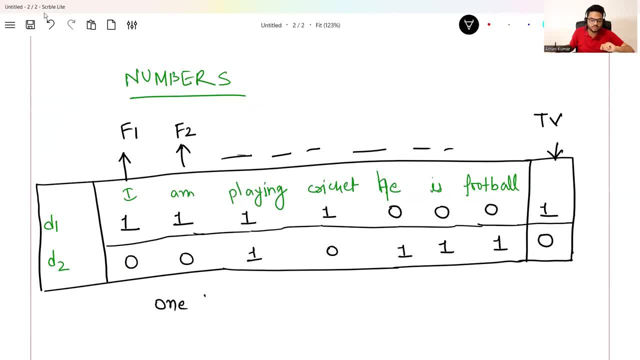 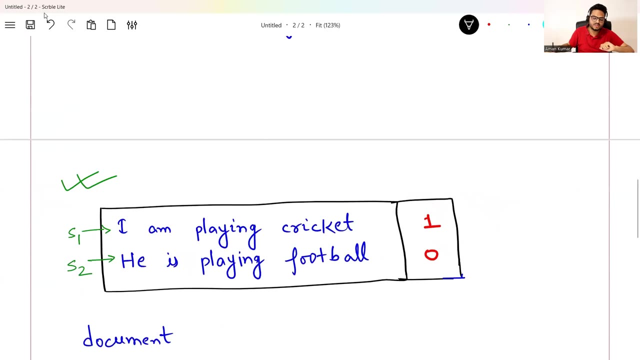 method is called, as most of you know, one hot encoding. Okay, one hot encoding. Now, if you noted down, I just made here small case, but in the sentence he was in, X is in capital letter, right? So if you see, in the sentence I am writing here, I should have written here. 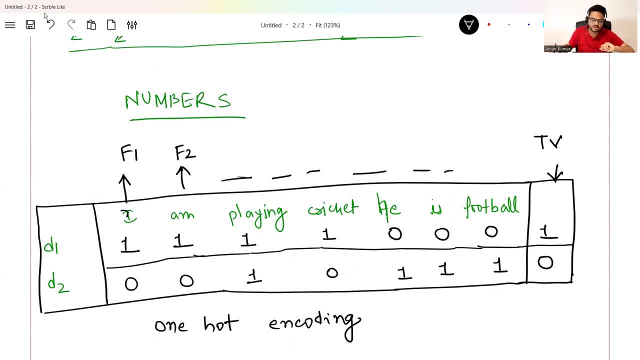 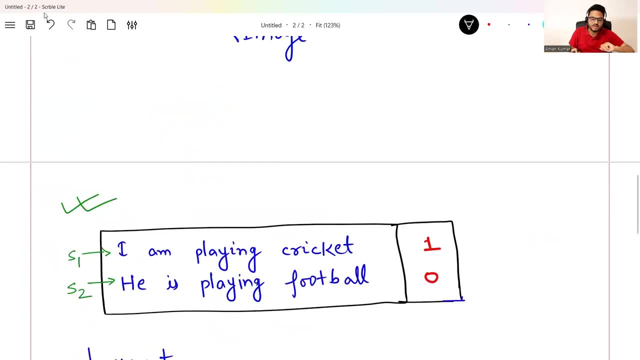 Let me write here in small case only. It should be small case only. understand this as small case. Okay, everything, understand that is a small case. So if you notice here, few things are capital here and few things are small letters here. But in my, in my data preparation, when, when I'm preparing the data, right, 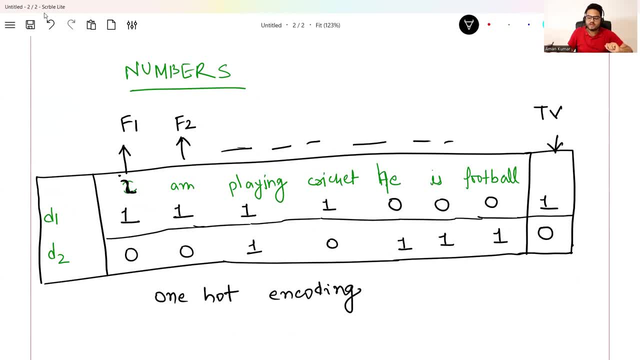 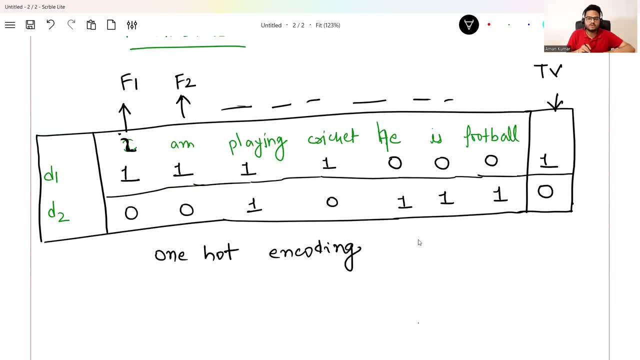 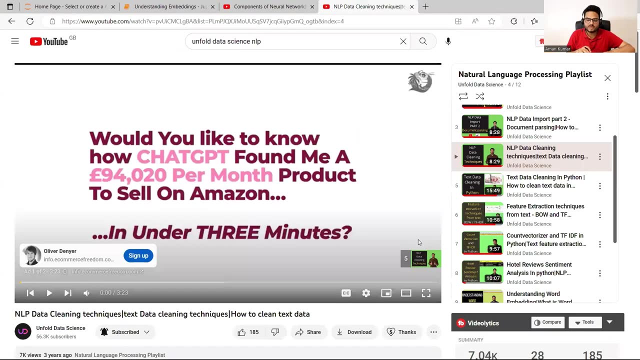 I am making everything at small case, Okay, and this is one kind of text cleaning. This is one kind of cleaning of text data. So if you want to understand more about what are different text cleaning techniques and how it is done, then I want to take your attention to unfold data science NLP playlist on YouTube. 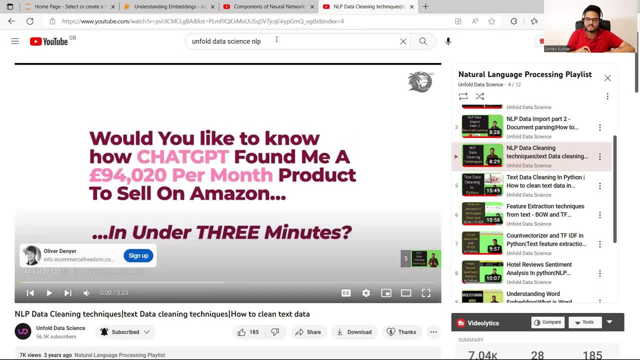 So you have to go and search for unfold data science, NLP. You will find a video playlist on YouTube Of 12 videos. just watch the video called NLP: data cleaning technique. Okay, you will know what are different data cleaning techniques used in the world of NLP. 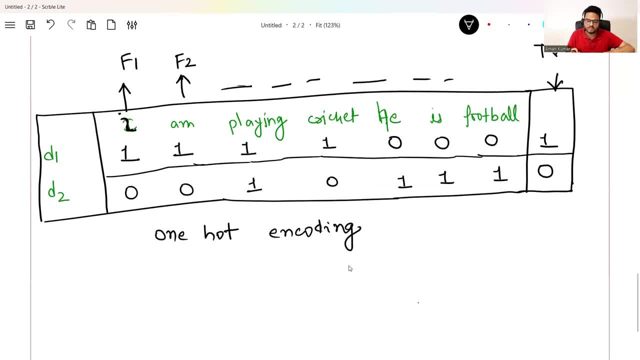 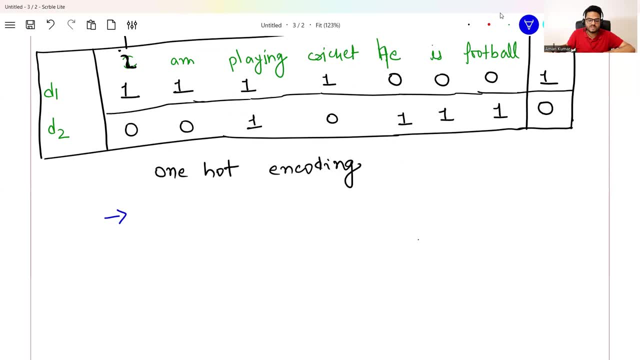 Okay, So now we have a one hot encoded document in front of us, but there are some problems with this approach. What is the first problem? First problem is this document will be unnecessary, very, very large because- understand here, here- we have limited number of words. 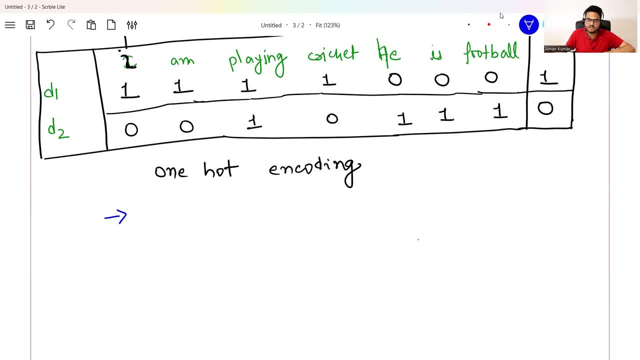 What if there are large number of words? This document will be very, very large and most of the entries will be zero. So that is a problem of something known as sparse matrix. Okay, sparse matrix. So it will be very, very large matrix and lot of zeros. 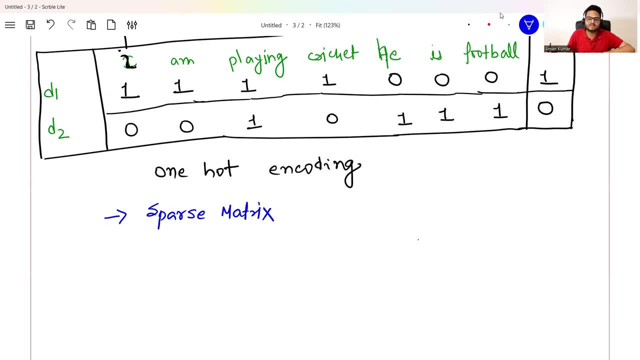 Hence it will take a lot of processing time. and second problem with this is these words. right, These words are treated individually. Okay, so words are Treated individually. individually means there is no capturing of relation between the words. I will give you examples going forward, but you have to understand all these words are. 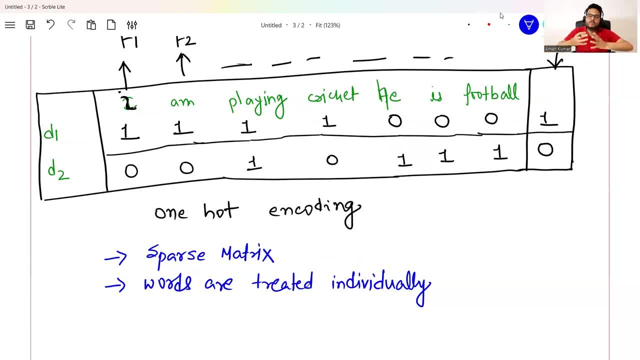 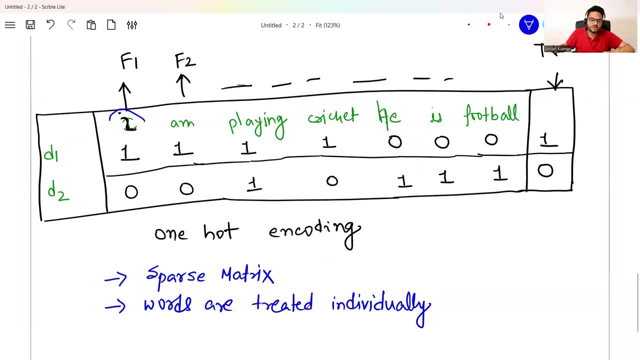 simply put in a bag. So there is a concept of bag of words. So this is very simple. like you, have broken all the words in tokens. So what are the tokens? I is one token, M is another token, playing is another token. So what you have done is: 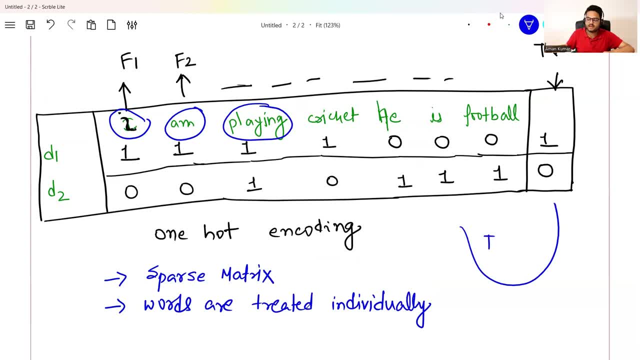 You have created a bag like this and you have put all your words like t1, t2, t3, like tokens. There is no order, maintained, There is no meaning, maintained, right. So all these words are treated separate, separate. That is one problem. 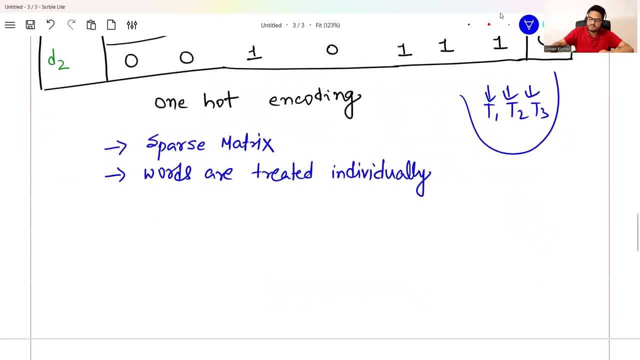 So what was the next thing that people did? people, what they did is they came to the world of something known as world of n grams. So I will write two here and I will say the world of the world of n grams. I'm explaining you all these techniques, guys, so that you will be very confident when you. 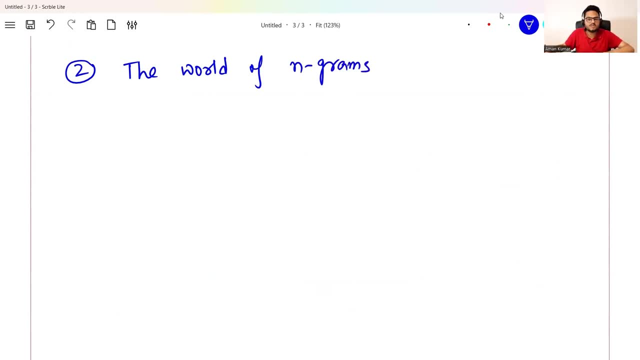 speak to someone, Okay, so remember those two words. I am playing cricket, He is playing football- Okay, so I will write here again so that we can take reference. I am playing cricket, Okay, and he is playing football, So these two words are there in front of you. 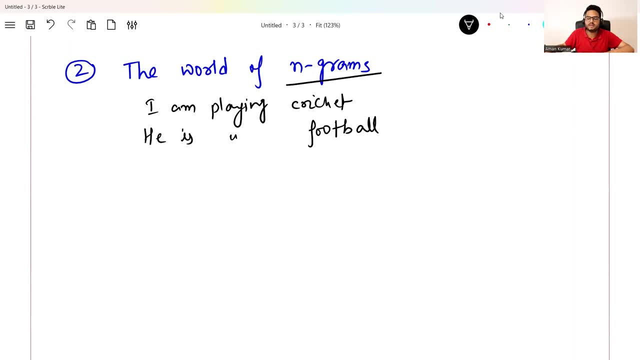 Okay, So these two words are there in front of us Now. what happened in the world of n grams is the meaning of n gram is we will create token of multiple words together, not a single single word. Okay, so n gram can be one gram also, and n gram can be two gram also, and n gram can be. 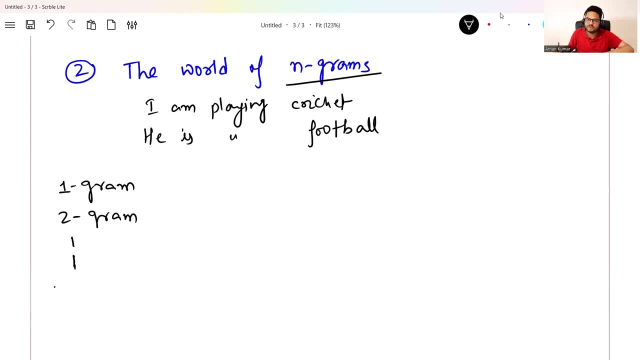 many grams, Okay, it can be four gram, five gram, six grams, and in the end it can be n gram, Okay. so what is the meaning of this? if I have to take one gram tokens from this right, then my tokens will be. I am playing all those things that was there in the previous example. 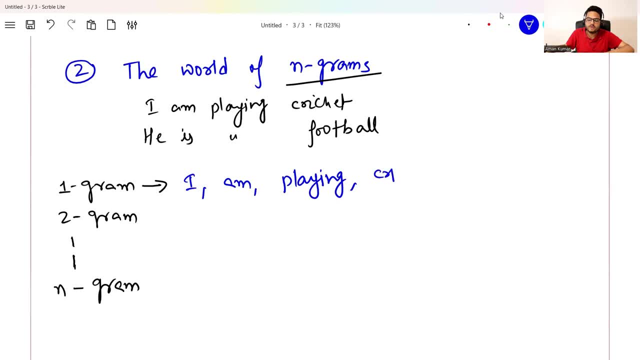 So one gram is nothing different than one hot encoding. Okay, so what will be your one gram tokens? cricket, then he then is, and then football. These are your one gram tokens. Okay, very similar to your one hot encoding in two gram tokens. 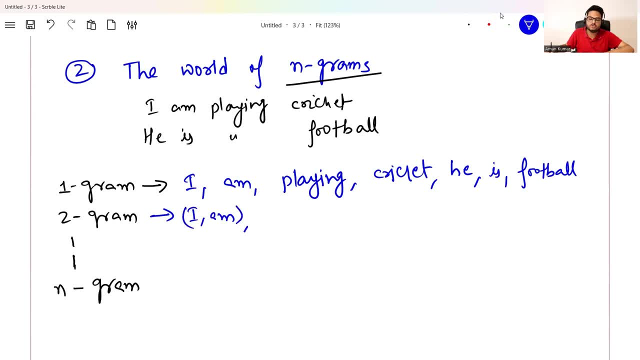 You will take two words together. For example, I am- this is your one token. I am playing, This is your another token. Okay, and then playing cricket, This is your third token. two gram token. understand, guys, What people were trying to do is they were trying to understand which two words, or three. 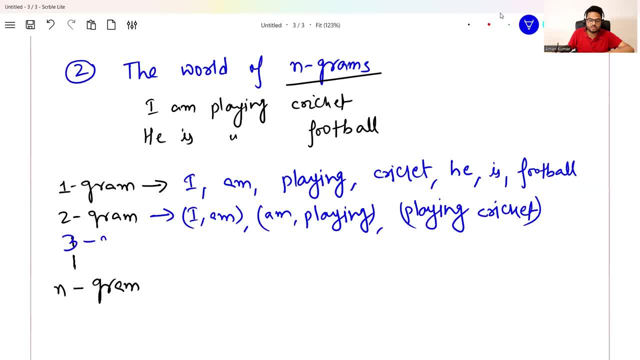 words come together. Suppose I write here three gram token, right? So in three gram token, how it will be created. I am playing. This is one token. Okay, and then another token will be: m playing cricket. I am playing cricket. 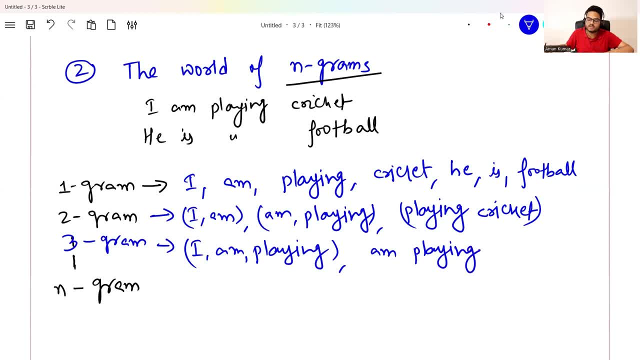 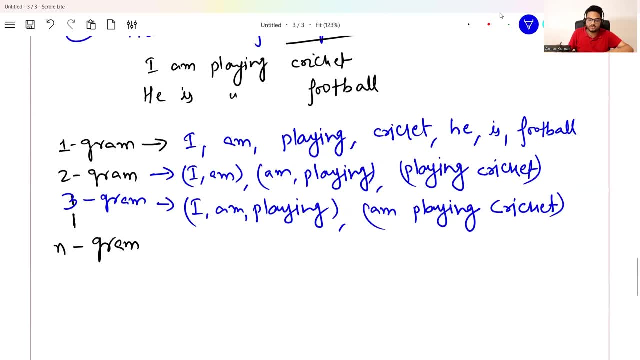 So understand this will not be taken from one document, only from the entire corpus. This will be taken. Okay, this is three gram token and similarly you can create a n gram tokens from this, as many as words you want to take. What is the advantage? 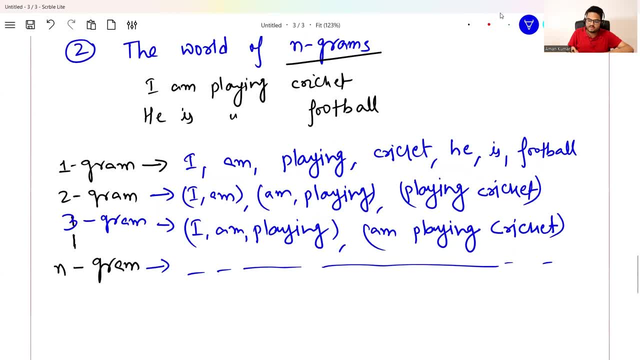 The advantage is, suppose playing cricket is coming here, So playing football will also come, So it will at least capture some meaning. So how do you create your your data training data? So the advantage is Your data training data. So, for example, this is your document one. 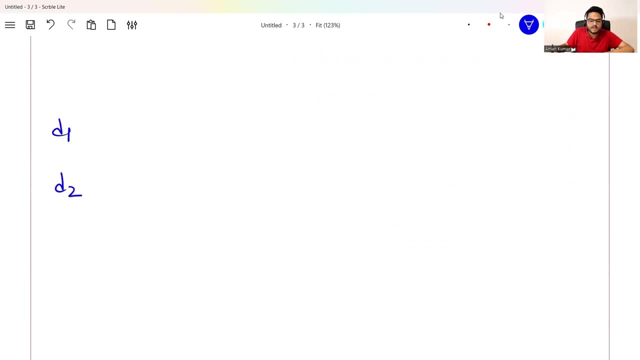 This is your document. two: So you will write your n gram tokens here. So n gram tokens, This will be your one set of features. This will be your one set of features. Then you- sorry, I'm sorry- one gram tokens, you can say: and then here you can say two gram tokens, two. 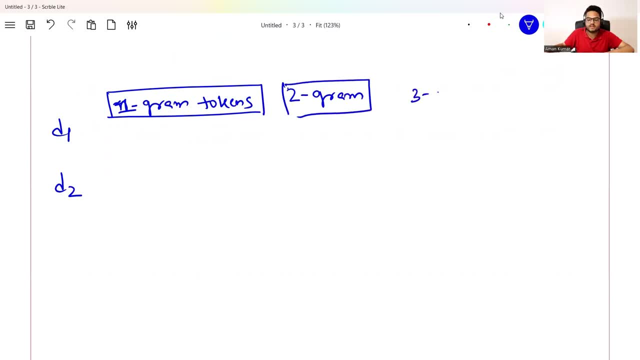 gram tokens will be your other set of features, and then three gram tokens and so on and so forth. So how many ever you want to take. So if I want to take one gram token, is I present? Yes, is M present? Yes, Two gram token: 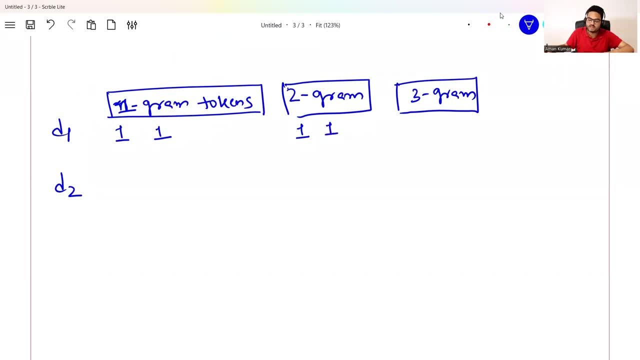 I am is present: Yes, M playing is present: Yes, Playing cricket is present: Yes, Playing football is present: No. Similarly for this and similarly for document two. Now, what is happening here? You are trying to capture some context. 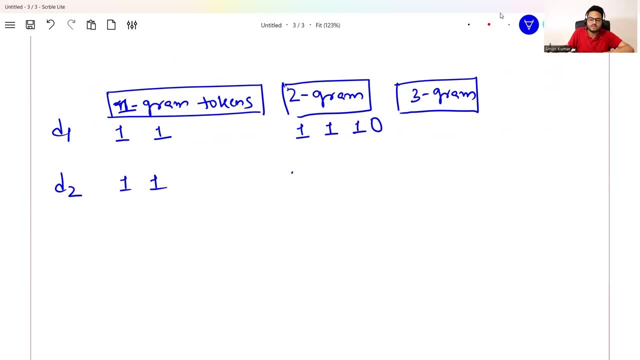 So for document two, also maybe one one, some zero, some one, some zero, some one, Okay, And then here in the end your target variable will be there, one or zero. So now the prediction can happen on this. So this becomes your training data. 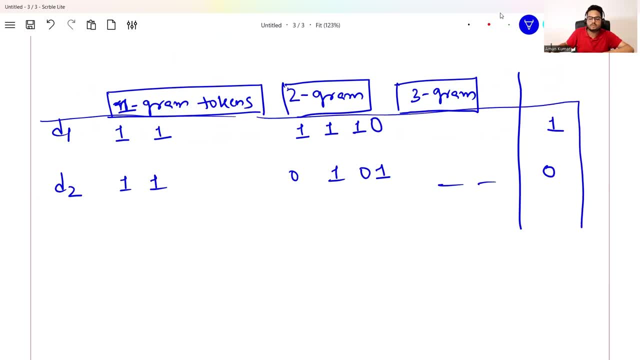 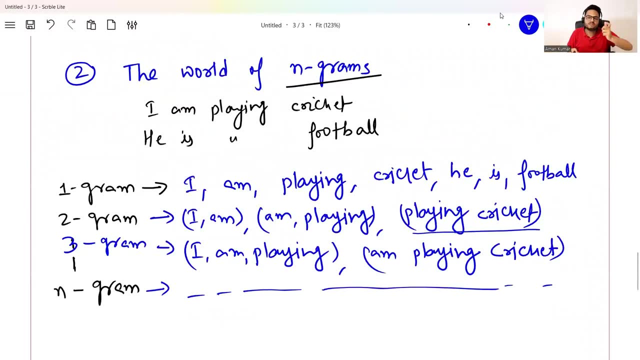 You have a lot of features now and then your you know you can train your model based on this. So how this model is different from basic one, hot encoding at least some meaning of the word and some more context We are trying to understand. this is the world of n grams. 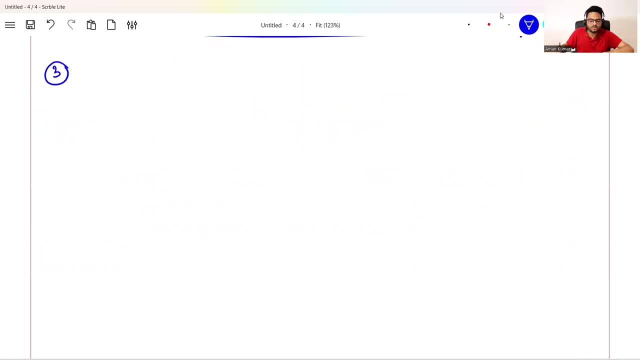 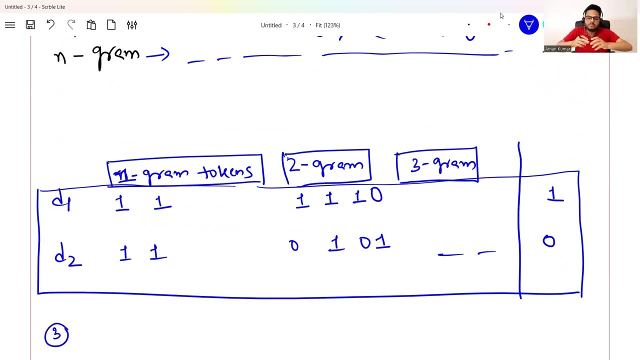 Okay, Now let's move to the third. What is the problem with n grams? again, sparse, metric problem, and You know it is not very efficient. how many tokens you will create, how many grams you will create, right. So one gram itself will be very too many tokens. 2 grams will be too many tokens. 3 grams will. 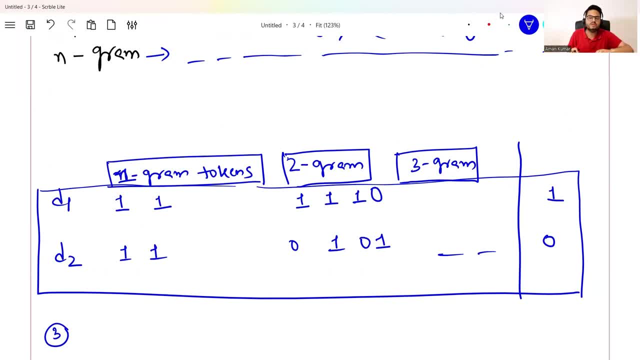 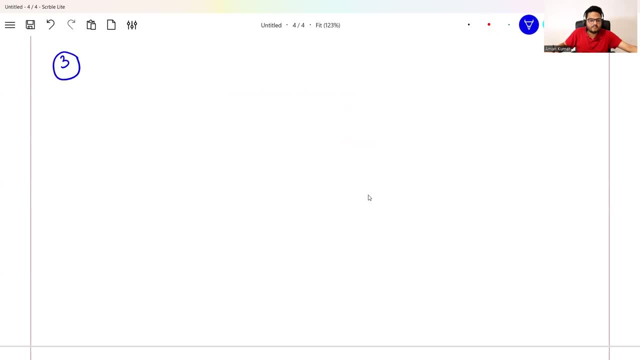 be too many tokens, right, many tokens will be there. So how many you can keep creating, right? So this is again a sparse metric problem. computation problem as the third technique, people move to something known as TF, IDF. Okay, TF stands for term frequency and IDF stands for inverse frequency. 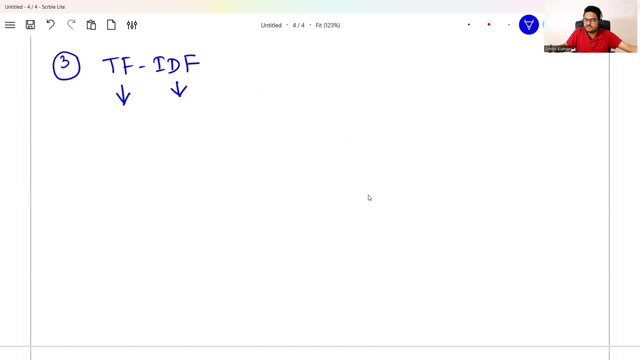 Okay, TF stands for inverse document frequency. What is the purpose of this particular mechanism? is suppose there are two words in front of you, the two sentences that I just mentioned, for example. just to understand simply, I will write it here again: I am playing cricket, Okay, and then he is playing football. 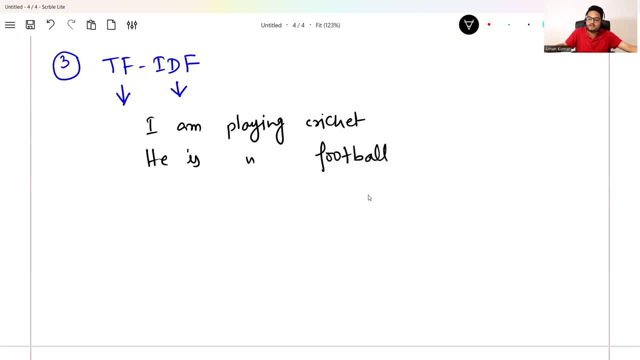 If you notice here in these two sentences, guys playing word is common in both These sentences. Okay, but what differentiates these two sentences? the presence of cricket and football. So in TF IDF the prime agenda is to not look sentences individually. Okay. 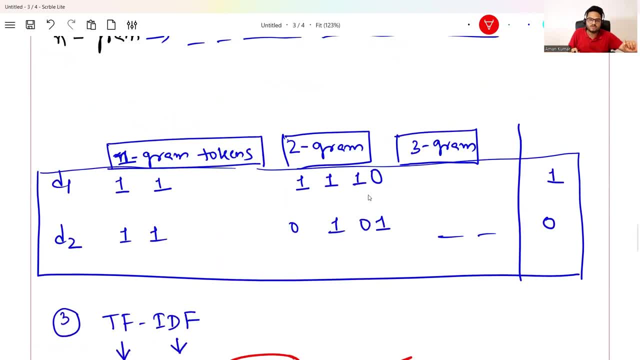 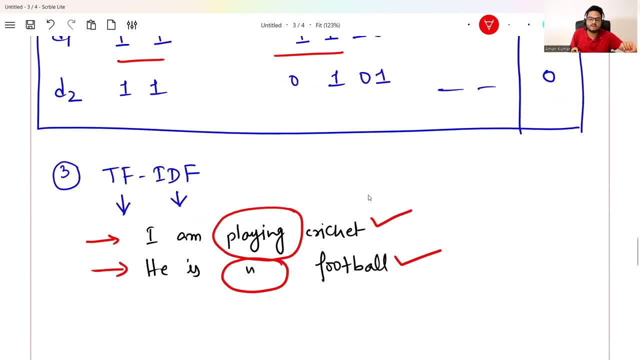 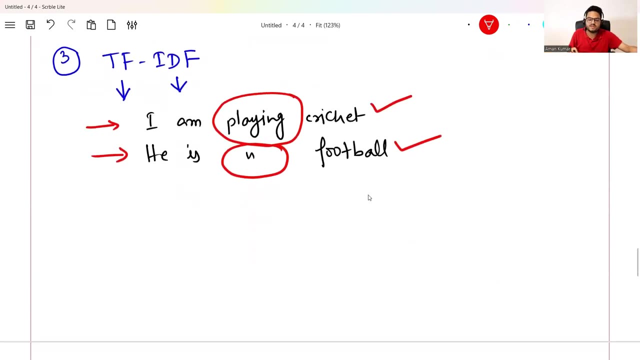 So in all these techniques till now you might be noticing, sentences or documents are looked individually and these numbers are computed in TF, IDF, sentences and corpus is looked together and a differentiator is tried to create here. So how the differentiator will be created is words which are common across all the documents. 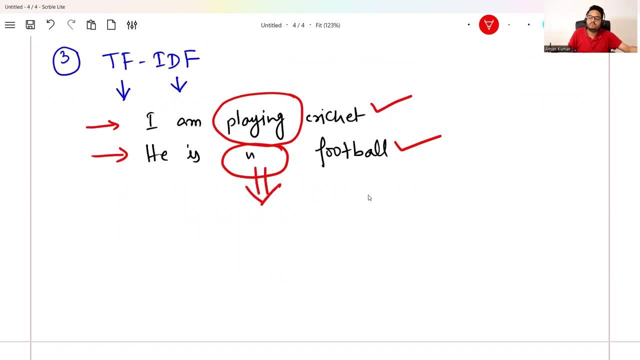 these will be given. low weight is okay, and words which is present in only one documents. these will be given how it is a high weight is for that particular document. There is a complete mathematics behind it. For example, if I write here cricket, okay, and if I write here football, okay, and if 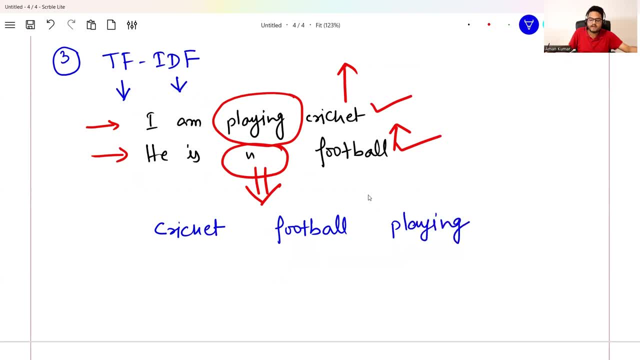 I write here playing Okay and I want to compute TF IDF score of document one and document to then. in document one, the TF IDF score for cricket will be high. in document to, the TF IDF score for football will be high. the playing score in both these documents will be very, very low or zero. 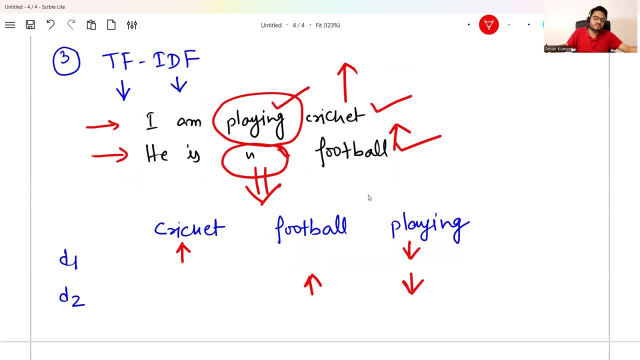 The reason for that is playing is a common word in both these documents and the differentiator is cricket and football, So their numbers will be high. There is a Complete mathematics behind it. if you want to go in more detail, guys, again I will refer. 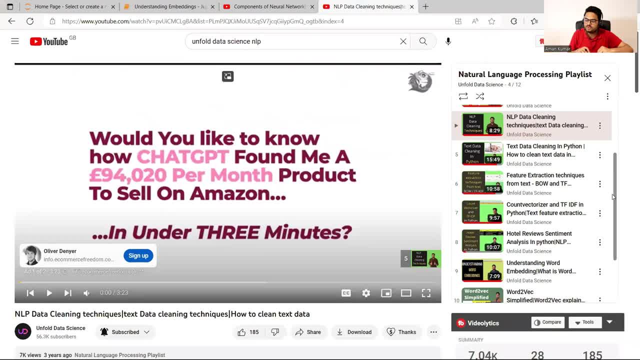 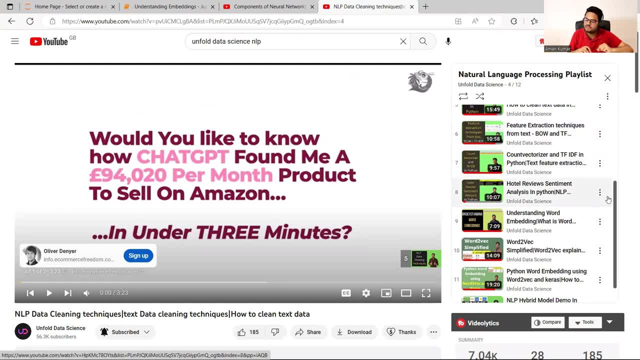 you to the same playlist that I was mentioning and here you can go and see feature extraction techniques from bag of words to TF IDF, count vectorizer and TF IDF, and I have done one use case, also using TF IDF, So it will be very easy for you to understand from here all the mathematics I have explained. 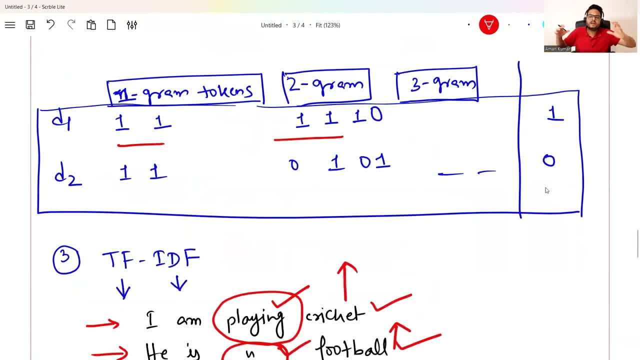 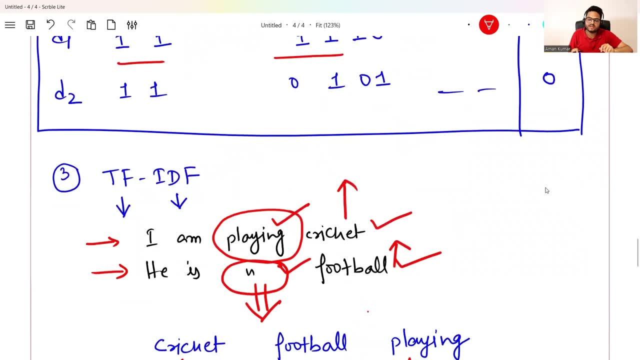 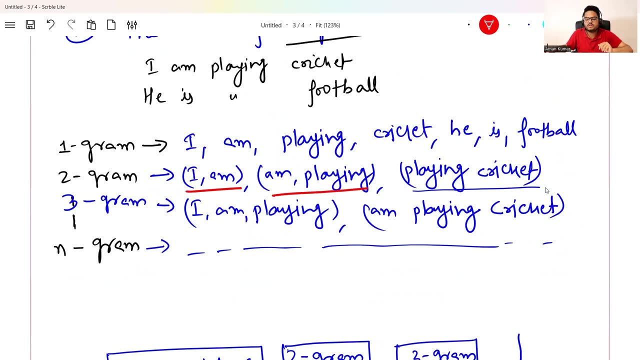 there. Okay, So now what is happening now? entire corpus, people, people started looking together, try to understand the meaning, Meaning of words and compute TF IDF. TF IDF can be computed for n-gram tokens, also not individual token. suppose I want to compute TF IDF for this or this or this? I can very well do that. 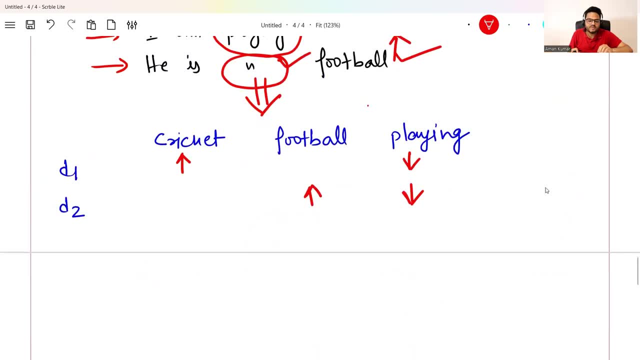 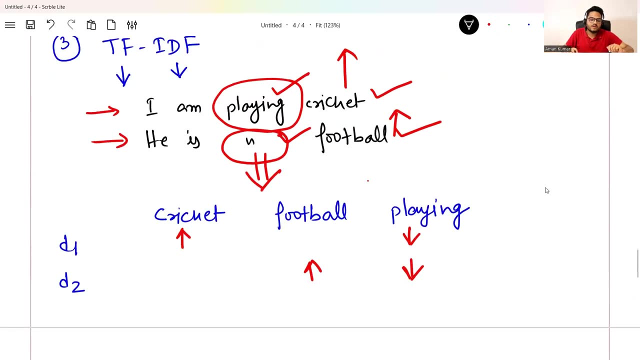 that is doable. Okay, so up to TF IDF. at least some some meaning started coming in the world of NLP, some, some things we are able to capture right now. TF IDF was number three. I was just checking which number I am in, and then I will go to number four. 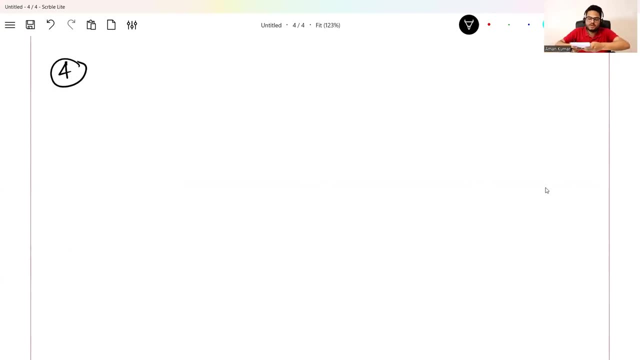 Now, what is number four? As it moves forward it becomes little more interesting. Let me see my notes here once, which I have noted at number four. at number four, We will learn something about the world of word embedding, the world of word embedding. Now one thing to notice here, guys. till now we are processing document by document. 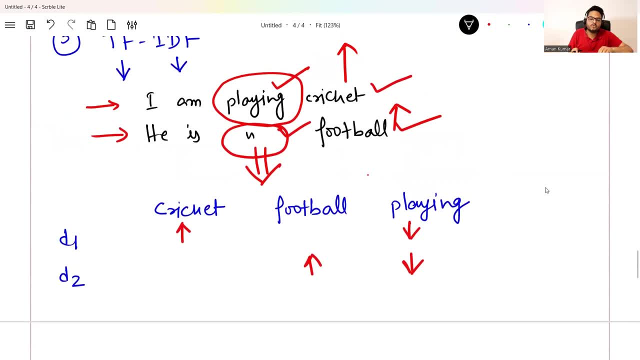 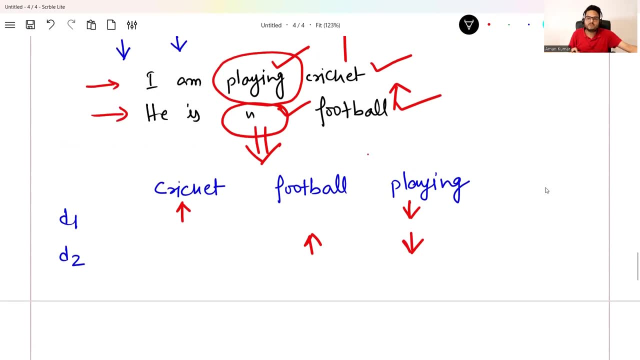 If you notice here all these techniques will go and look for word occurrence in a document and create a matrix based on that. What if I want to process my document word by word? What if I want to process my machine learning engine word by word? 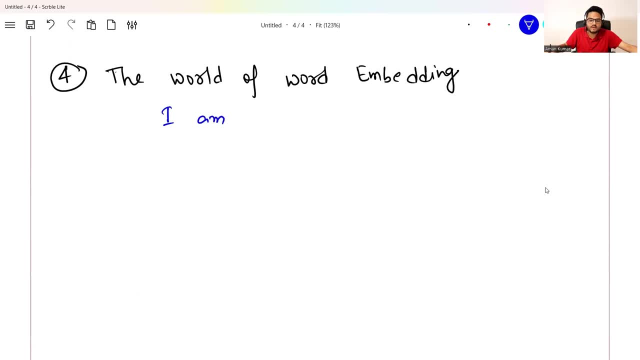 For example, here I have a sentence: I am playing cricket. okay, so I do not want to process this sentence as a whole, rather I want to learn from word by word. So I will treat I first, then I will treat M, then I will treat playing. 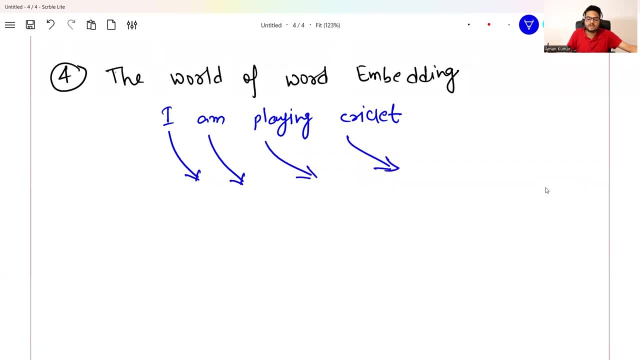 Then I will treat, Then I will treat cricket. So how do you do that? How do you? you know, treat word, So word needs to be converted to numbers and those are called word vectors. Okay, remember these terminology, guys: word vectors. word vectors means what if I create? 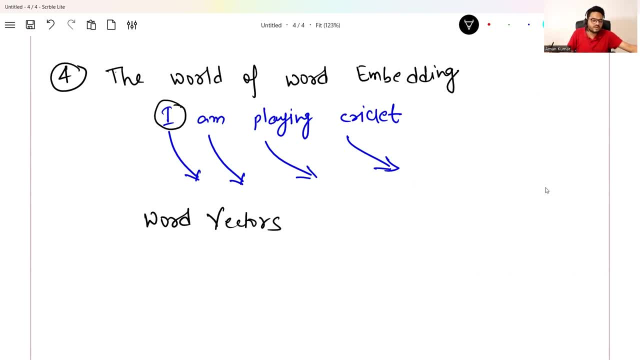 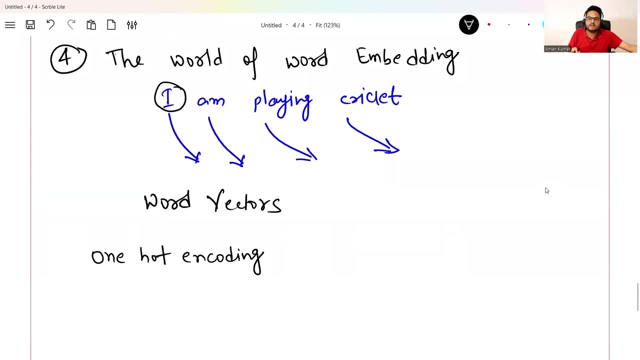 a vector from this word. How will you create a vector from this word? One famous technique is known as again one hot encoding. one hot encoding. Okay, One hot encoding. what it will do is it will simply assign a number to all the words in 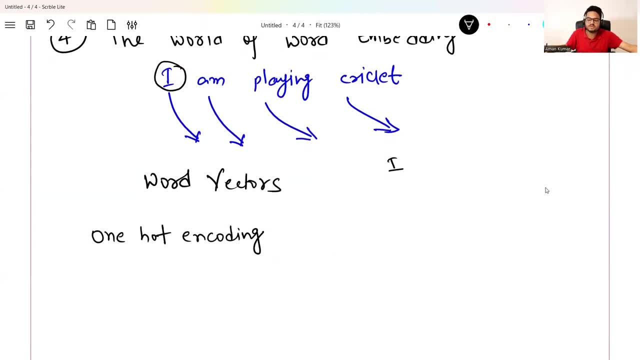 your corpus. For example, how many words are there in my corpus? I am playing, playing cricket. Let's take first sentence. only just to make you understand. I'm not taking the second sentence. now. suppose I is your word number one. aim is your word number two, playing is your word. 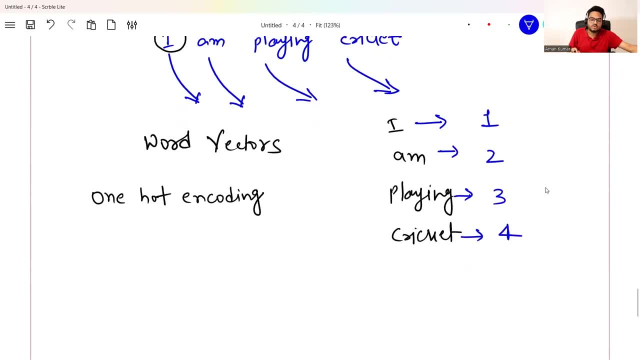 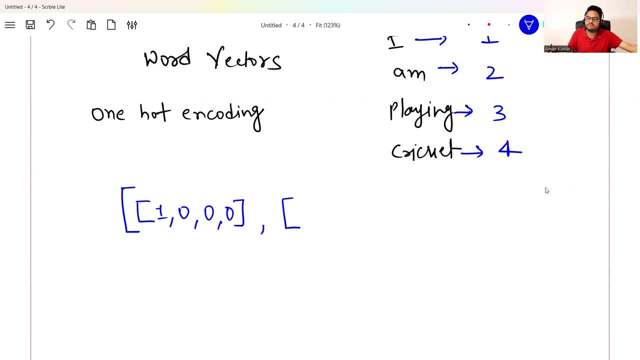 number three: Cricket is your word, Aim is number four. So if you do a one hot encoding right, then this is how your same sentence will look like one zero, zero, zero. This is your first word. try to understand this guy. This is the base for everything in RN and LSTM and large language models. 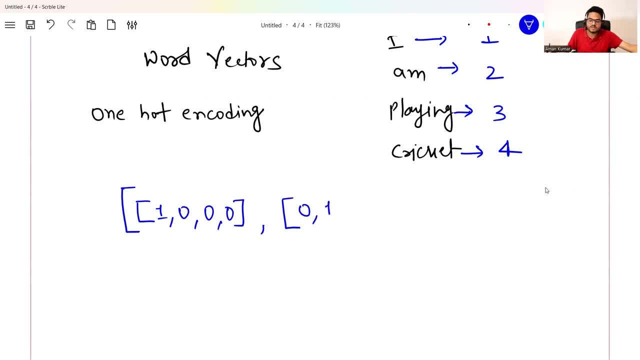 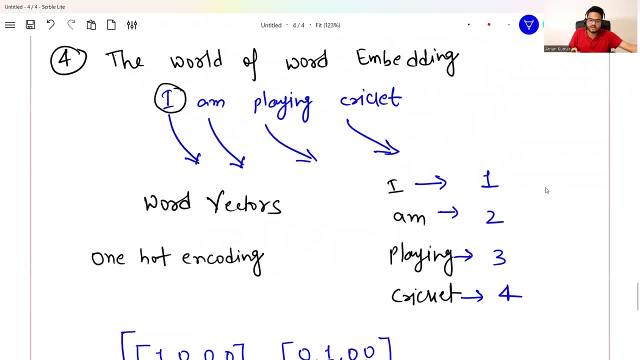 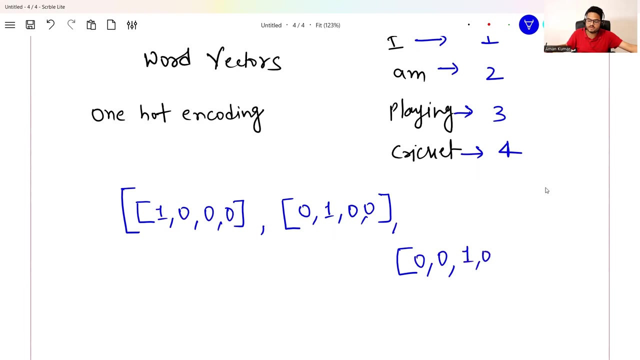 Okay, one zero, zero, zero is your first word. then zero, one, zero, zero is your second word. okay, because aim is number two. aim is number two, right? So second word, One third word becomes zero, zero, one, zero. third word. fourth word: zero, zero, zero one. 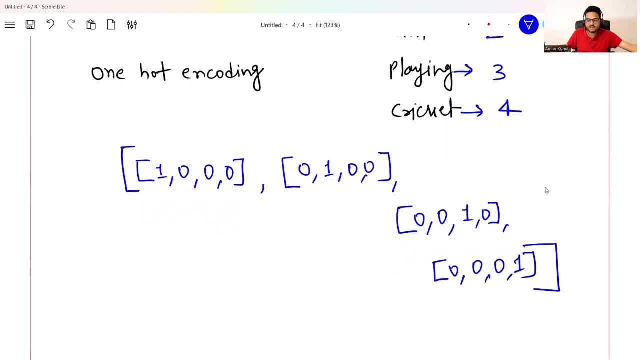 So try to understand, don't confuse. this entire thing is your first sentence. this entire thing is your first sentence, okay, and this is your word one, this is your word two, this is your word three and this is your word four. And this is called this one: zero, zero. this thing is word vector. 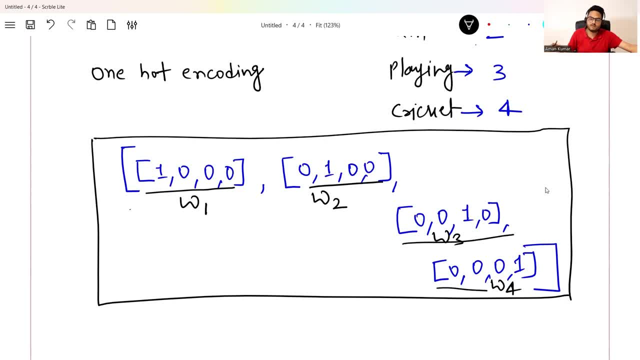 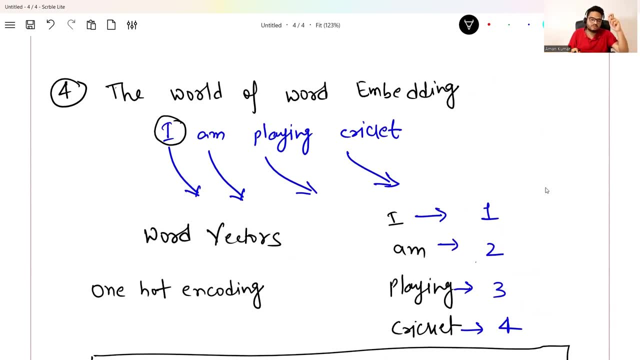 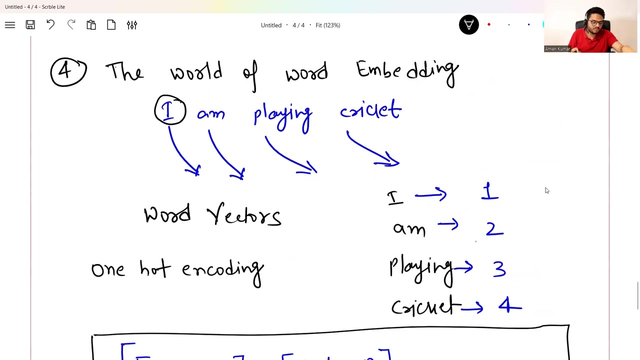 This is word vector, This is word vector and this is word vector. So I told you one technique of one hot encoding to encode your numbers word into word vectors, and from this only the advanced techniques of word embedding came into picture. Okay, I'm going to show you in Python how the advanced word embeddings are working, but one. 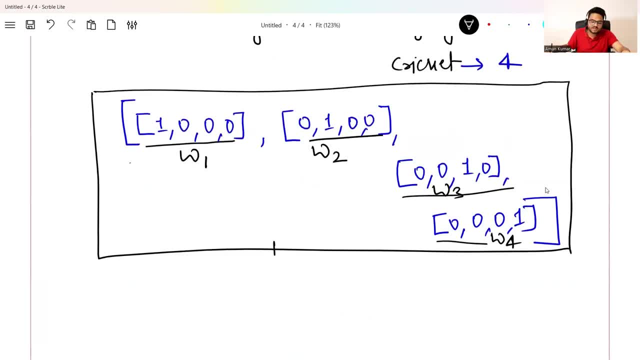 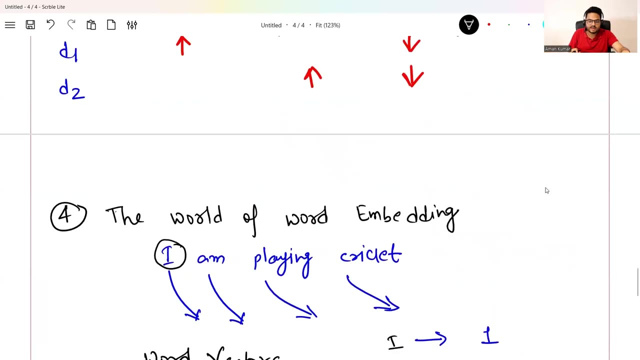 thing I want to tell you here: when word embeddings came into into the picture, then artificial neural networks started gaining a lot of attention in the industry. artificial neural networks why? because it needs a lot of processing power. now understand, guys. this looks much simpler if I talk from processing point of view, right from machine point of view. processing point: 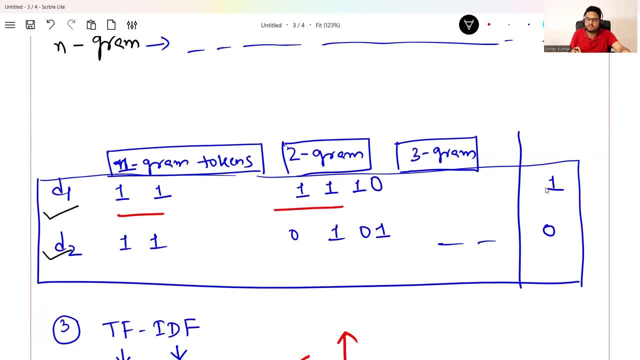 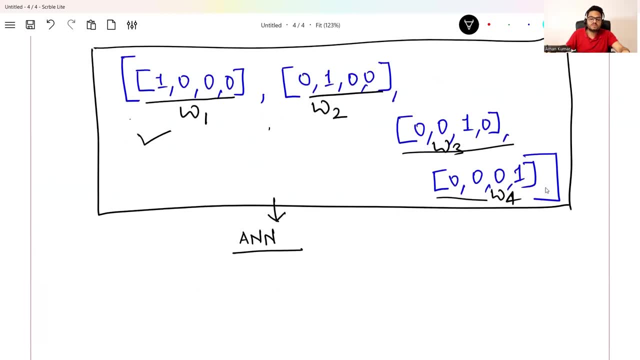 of view. if I go document by document, it looks a little simpler, right, but if I go word by word, right then my input itself is becoming very, very huge. so processing will become huge and it will need need more memory and more complex network. and that is when the artificial 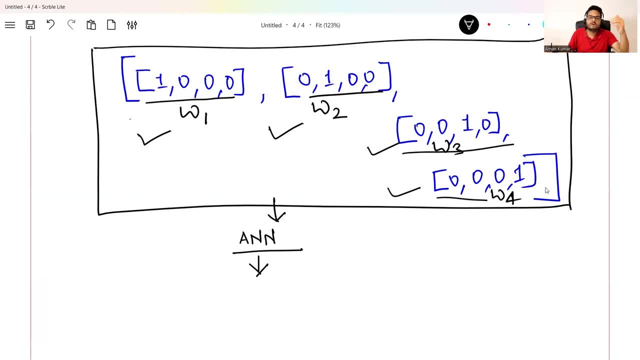 neural networks became popular, then word embeddings and all these things started taking picture, started taking, you know, front seat in the world of NLP. so what is the problem with word embedding? again, this is computationally expensive. as I told you, the input will go all together in different way. 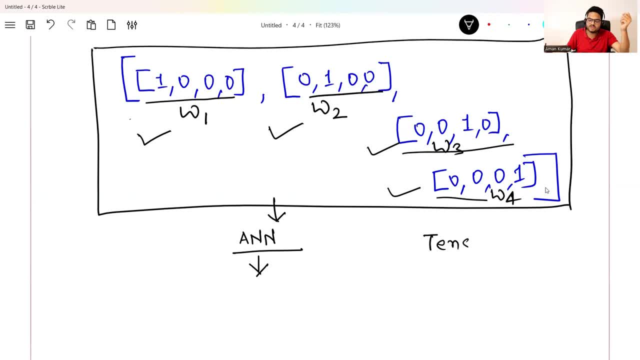 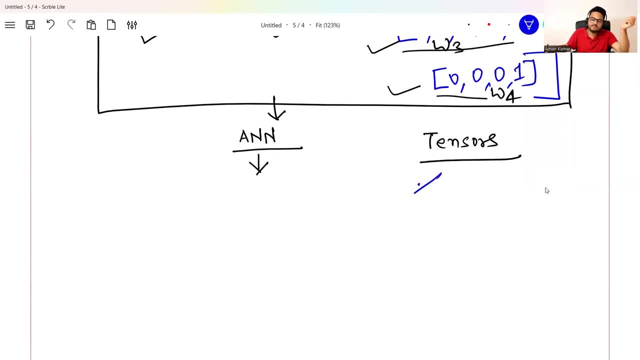 So if you don't know the concept of tensors, guys, please read about it. it's a very, very simple topic to understand. you can simply, you know, if you are a python guy, you can simply think it like: n dimensional array, okay, and the array in python. so if there is one value, 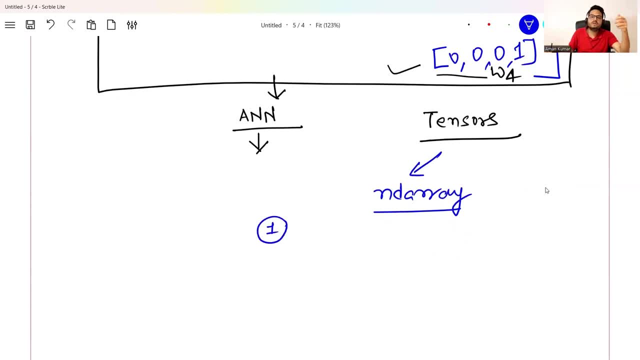 one single value, then this is like one, one scalar value. if I write like one, two, three, four, this is one kind of vector value, and I can write a 2D vector, I can write a 3D vector, I can write a n dimensional vector, right? so in the world of machine learning, tensors are 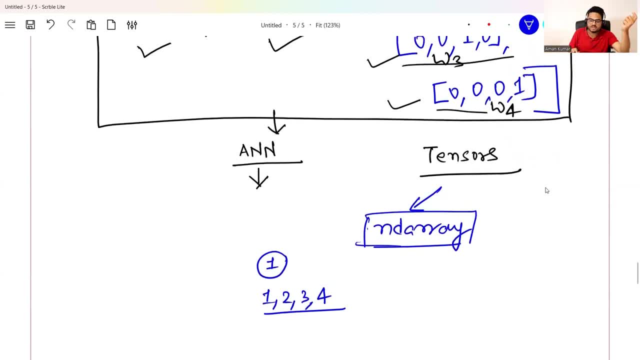 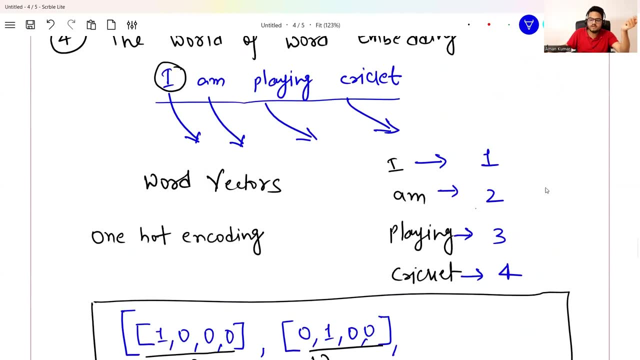 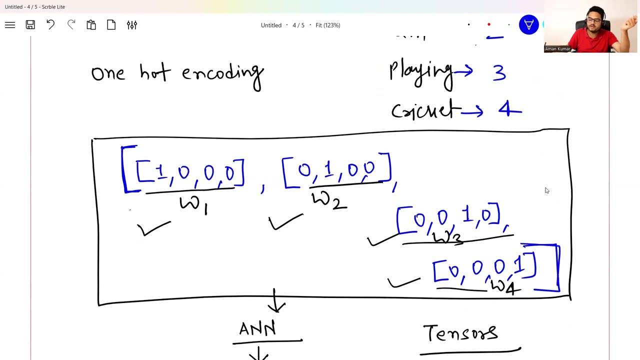 nothing, but you can think of n dimensional array and where that is used is now, suppose this, this sentence: you have to give input to your training, right, this sentence? so this sentence itself has become a n dimensional array, if you see this right. so this has become a n dimensional array, so this will be called as a tensor. okay, so it will go in input as: 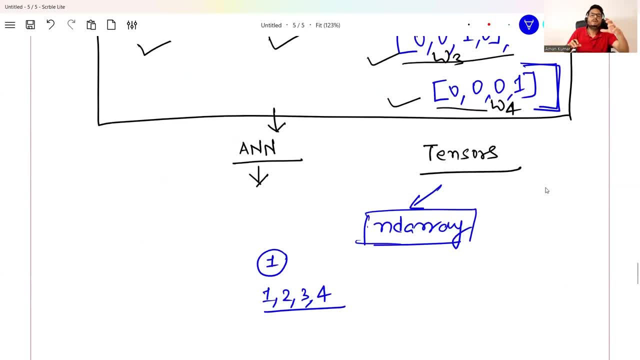 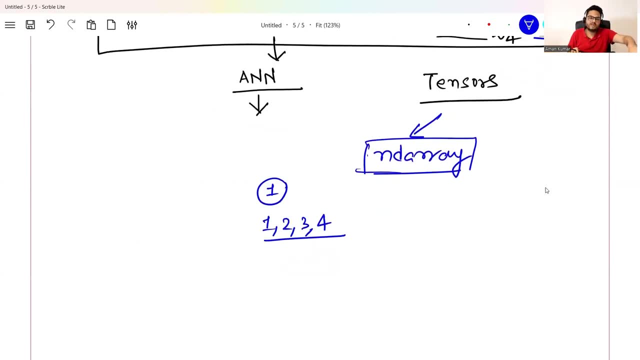 a tensor. so nothing to confuse. their tensor means input is going to be a tensor and the word embedding technique is going in n dimensional array. you have to understand. and since artificial neural network came, so these computations became possible. now, if I go one level from here, then there are different types of word embedding. I explained you a simple word: embedding. 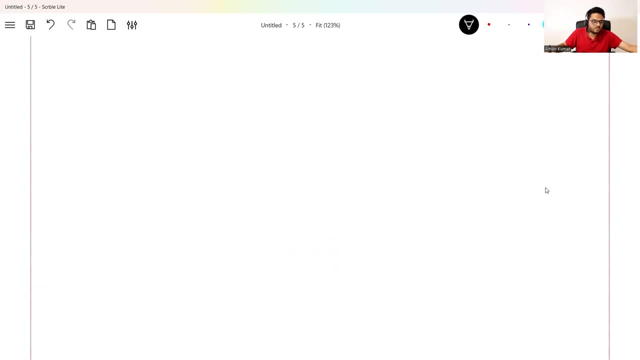 technique. that is one hot, but there are different types of word embedding techniques. for example, what to wake is a word embedding technique. okay, glove is another one word embedding technique. so what these will do is this will give you more meaning, like on trying to dive level of integration, top peurn on where we have our word embedding, International Word embedding. 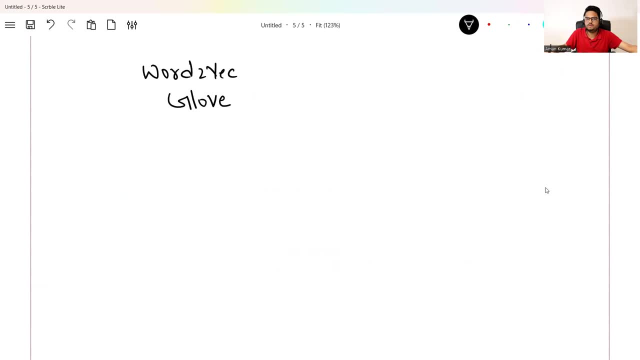 full embedding to your words. for example, if I take what to wake as an example, right, and if I take cricket as a word- so in normal- what one hot encoding- it will just be 101010, right, but this is a pre-trained model, what to wake is a pre-trained model, and globe is also a pre-trained model. 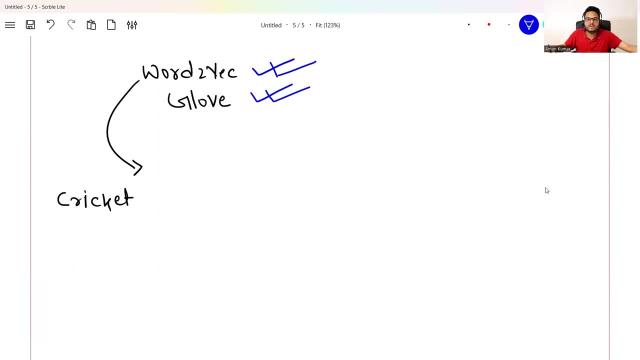 when you take a pre-trained model and when you embed your machine learning model, your data right, so it will be featured on some of the other dimensions. for example, is game is outdoor okay, is outdoor is multiplayer? I am writing here some features on these features. your word will be: 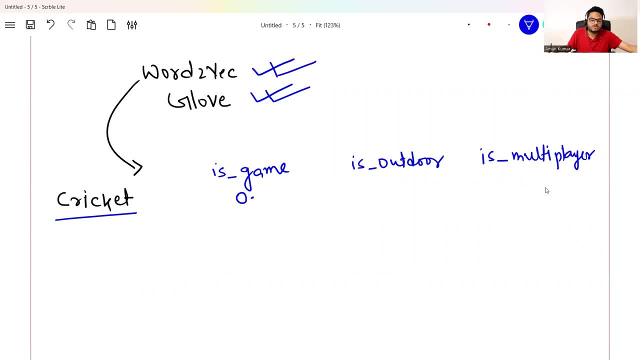 given a score. so cricket is a game. so 0.9 score out of one is an outdoor game. 0.8 score out of one is an outdoor game. 0.9 score out of one is an outdoor game. 0.8 score out of one. 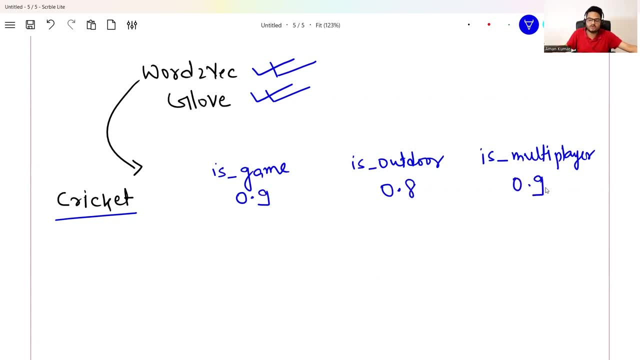 is an outdoor game. 0.9 score out of one is multiplayer game: 0.9 score out of one. so this becomes your vector. I am just writing here three. it can be a 300 or 3000 vector dimension vector. so I am writing here, not dimension objects, you know, presence of elements in the vector. 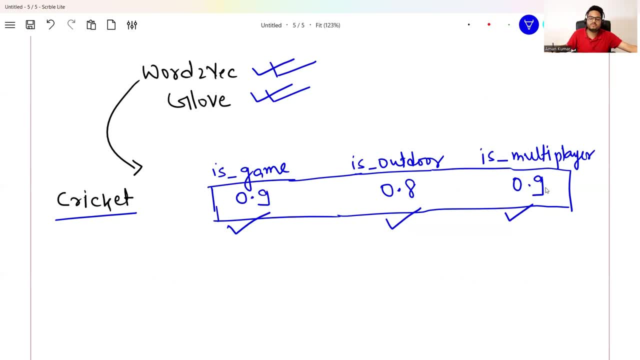 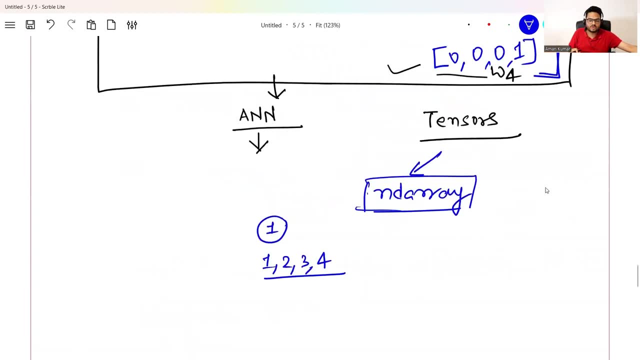 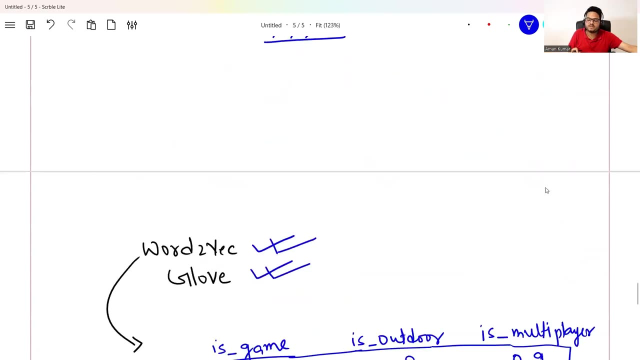 so 0.9, 0.8, 0.9. this is your vector cricket. okay, another word comes, one more vector gets generated. so if you compare from your normal one hot encoding, right, then that that looks little more meaningful. okay, so that is one kind of advance. you can say word. 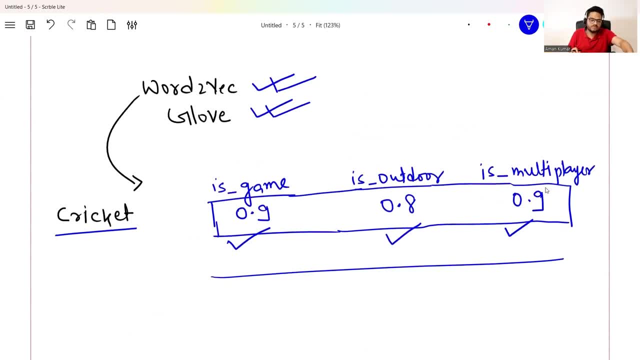 embedding technique, if you compare, like you know, some time back, but I am going to show you in python, in Keras, right in Keras, which is, which is a deep learning framework, it gives you its own embedding layer. okay, it gives you its own embedding layer in Keras. so what you? 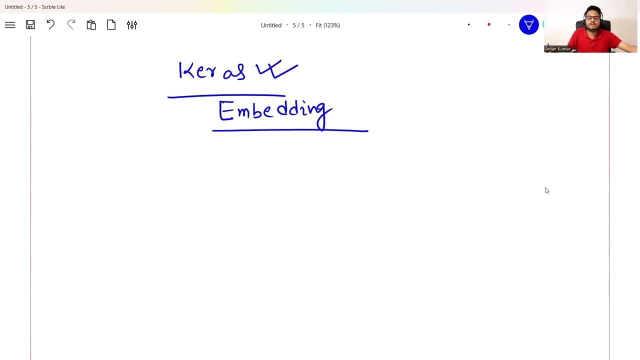 can do is: this is a famous deep learning framework in keras. you can simply say that this is my vector, this is my document, embed my document and you can just get your embedding done. and there is one more embedding that i will show you. in python now, that is known as integer based encoding. that is very 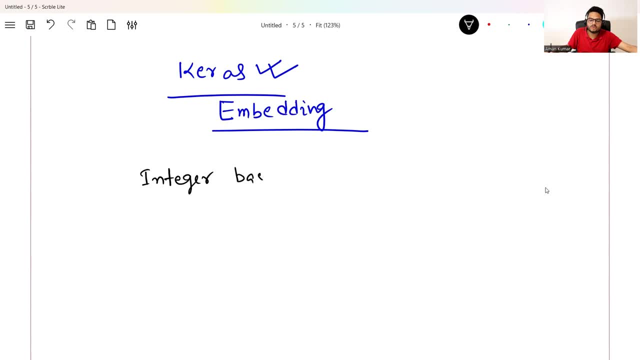 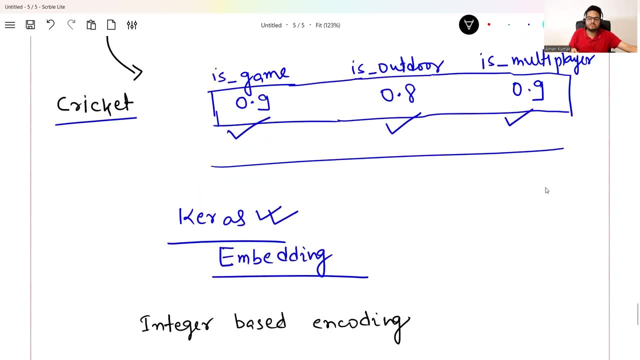 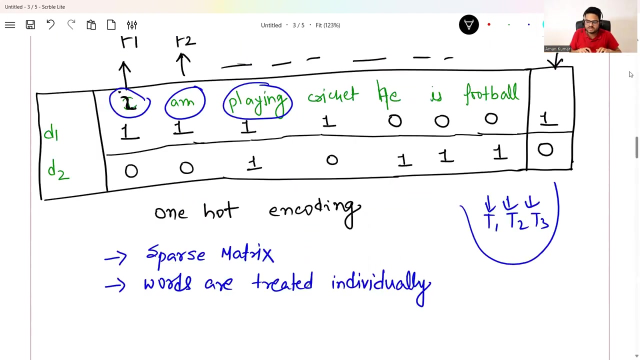 similar to what we saw in one hot encoding- okay, integer based encoding. so try to understand, guys, how things are improving in the world of nlp. i am going to python now and show you how these things are working together. just a quick revision. all these things we have understood how the nlp 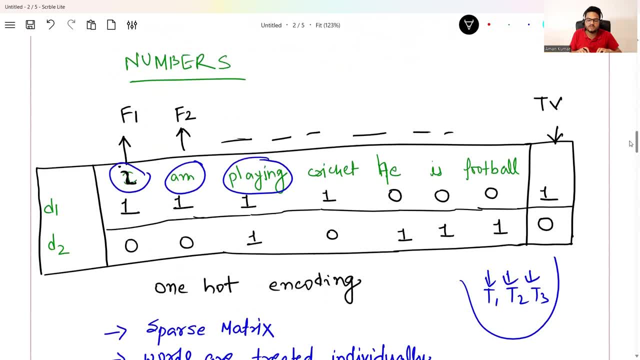 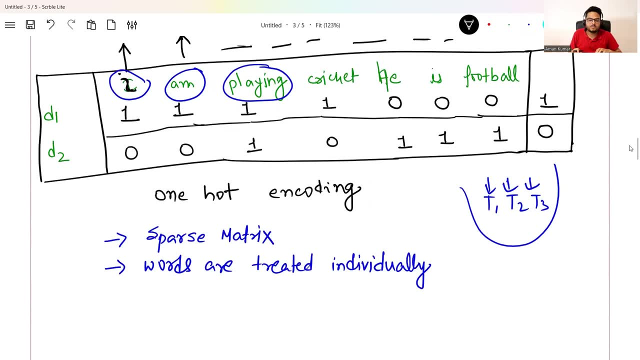 has improved right from count vectorizer counting the number of words. here, in place of one zero, you can also write count of the word. okay, that is counting the number of words, then problems with this, then the world of n grams, then how what happened in tf, idf, and then how the word. 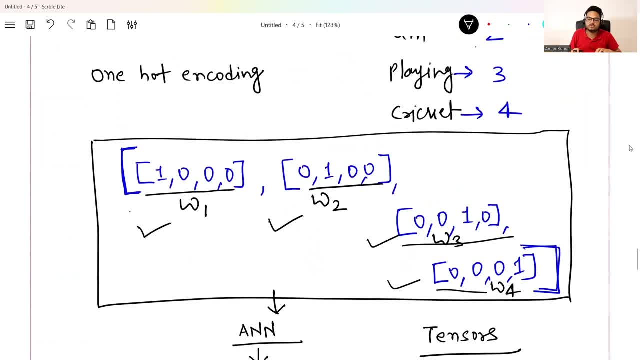 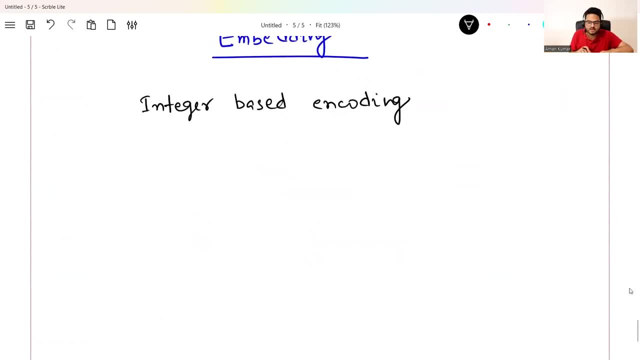 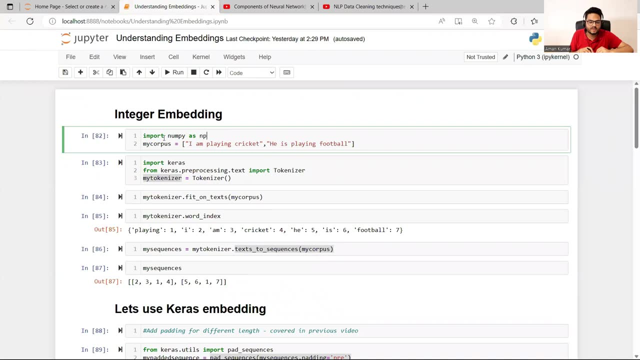 embedding came into picture. so converting word to vectors came into picture, some sophisticated way of converting what two vectors came into picture. and then let's go to python and see what are different embedding techniques that i want to show you. so here, guys, i have taken these two lines as 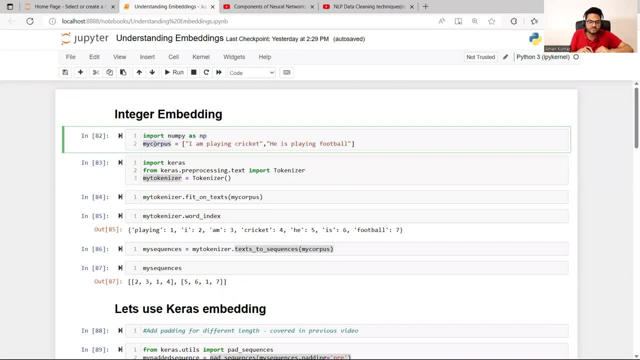 you can see import numpy as np my corpus. so what is my corpus? my corpus is simply combination of those two sentences that i am writing: i am playing cricket, he is playing football. this is my corpus: two documents or two sentences that you can see here. i will say: enter from keraspreprocessing. 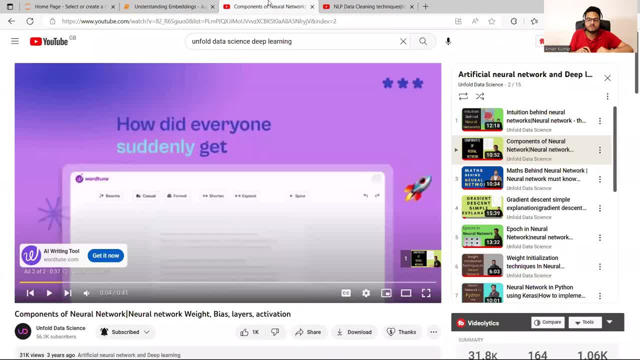 i am importing tokenizer. now some of you who is not aware of any concept of deep learning or neural network, you have to go to unfold data science, deep learning and right from intuition behind neural network. you will find all the video till optimizers in neural network. okay, 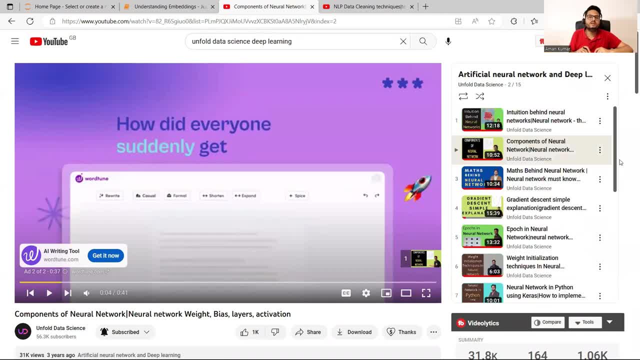 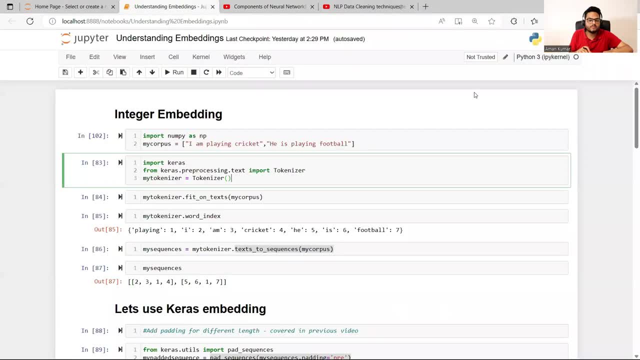 so everything that i will speak from here on. if you have any confusions, please go and see this playlist: 15 videos. all these are very, very useful for you. okay, so going back to keras is a famous deep learning framework. i will say here, from keras, i am importing preprocessingtext and i am saying i am initializing a tokenizer. 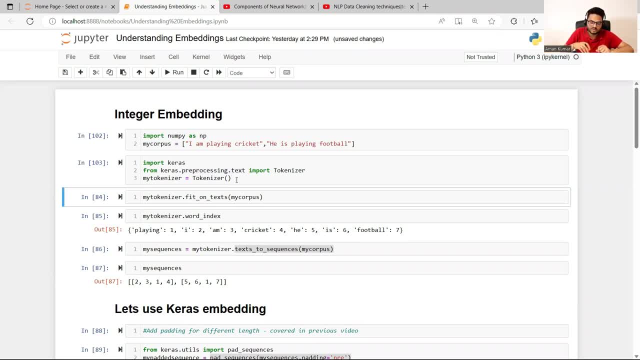 object tokenizer. object means it will tokenize my, my corpus, and then i am calling a method called fit on text. and then, if you see here, guys, whatever i am highlighting, right, the, the fit on text has given one number to all the words in my corpus. so playing is my word number one. 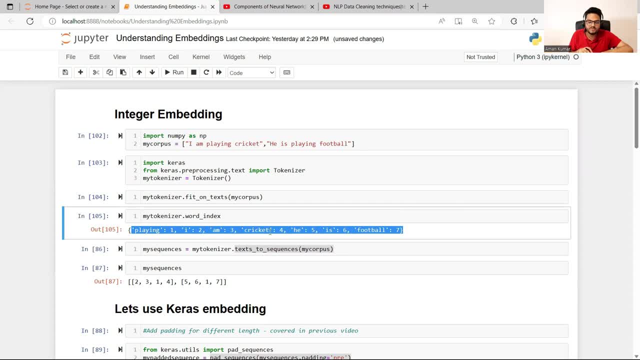 i is my word number two, m is my word number three, cricket is my word number four. he is my word number five is six, football seven. so as i was telling you in a theory, right, if you see here he is, h is capital here, but in the token h is small. how that becomes small. 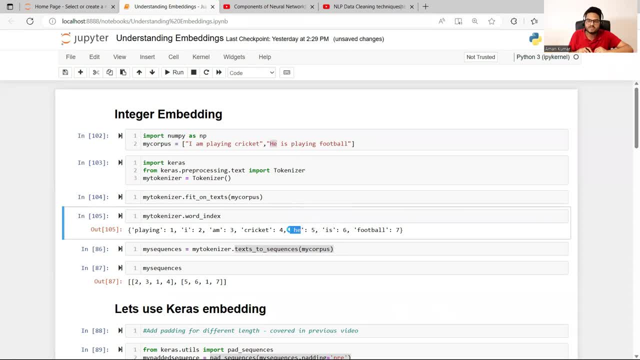 because keras itself did some pre-processing on my text. try to understand this. keras itself did some processing on my text and converted everything to lowercase and assigned a number. at the moment my words are assigned 11, number right, and then if I run text to, sequences, right. 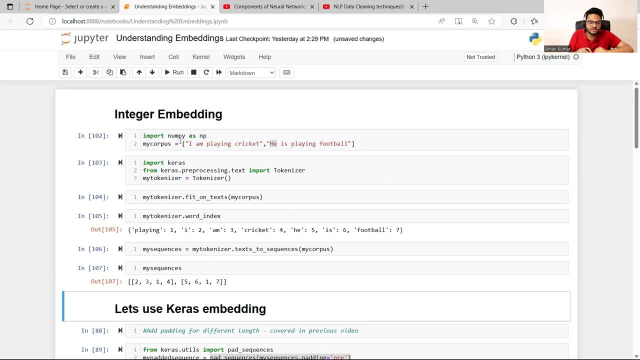 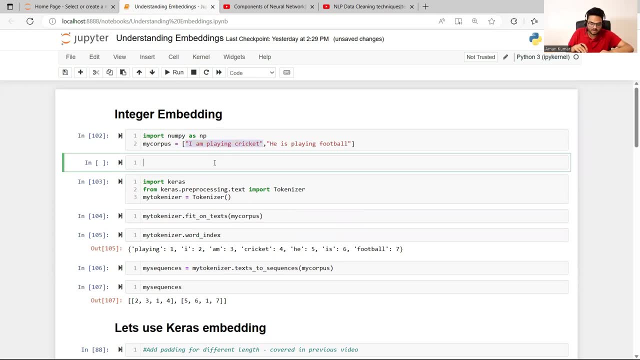 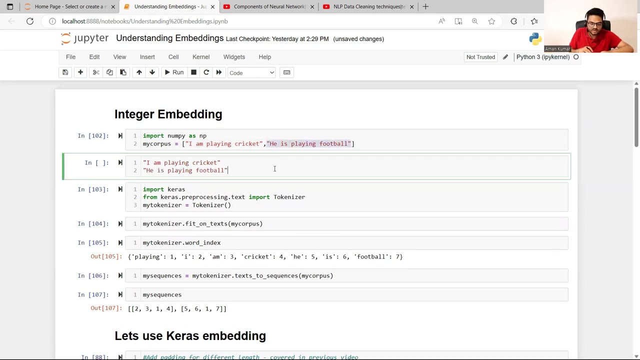 then you will see that my, my original document are these two. okay, so my first, my first document is: I am playing cricket and my second document is: he is playing football. okay, so I is which number word? I each second number word, so two. okay, you can see here these two words are: 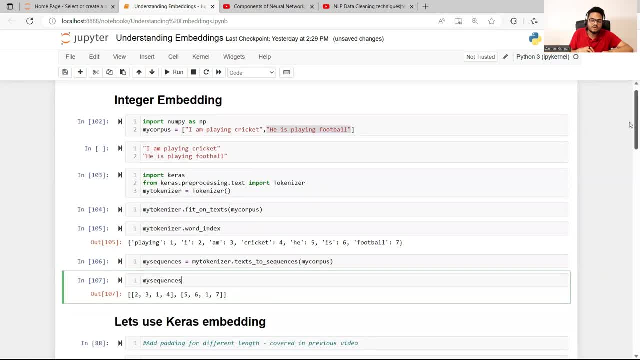 represented in terms of integers. now these two sentences. so two, three, one, four means I am playing cricket, two is I am is three, playing is one, cricket is four. so two, three, one, four is my four, is my first sentence. okay, five, six, one, seven. same way is my second sentence. he is playing football. 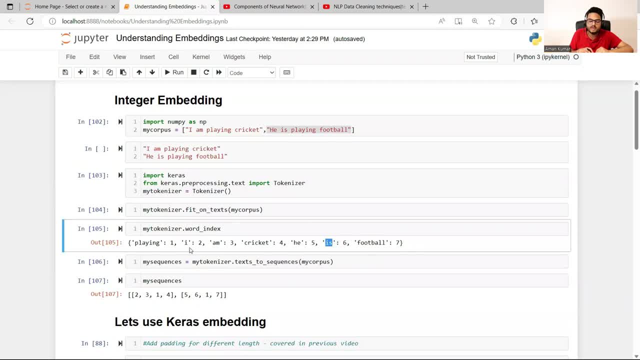 he is five, is six playing one and football seven. so what I have done here is I have imported a python package from Keras and I have converted my text to numbers using something known as integer embedding. this is called as a integer embedding: all your words will be given one. 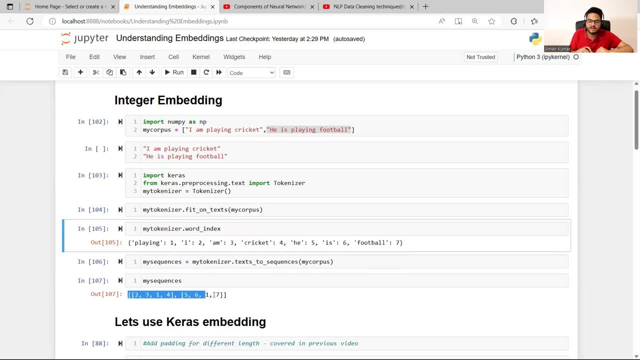 one integer number and your sentence will be converted like this, very similar to one hot encoding, just that numbers are here, integer numbers are here. okay, so if we move from here, the other technique, the other word embedding technique that I want to show you comes directly from Keras. Keras will embed it for you. so if I 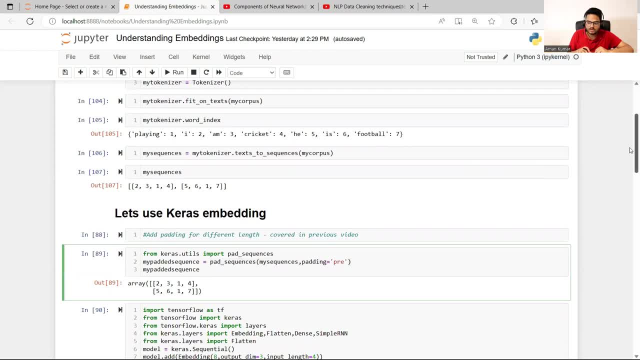 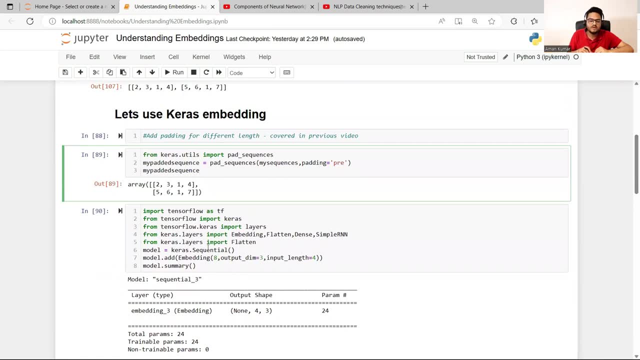 go here and I am just creating a pad sequence which which I am creating for for some purpose. I will come back to this later, but before that, guys, here, as you can see, import tensorflow. I am importing embedding layer and then flatten and dense and simple and n I am not using. don't worry about all this. if you see, most of these things, I am. 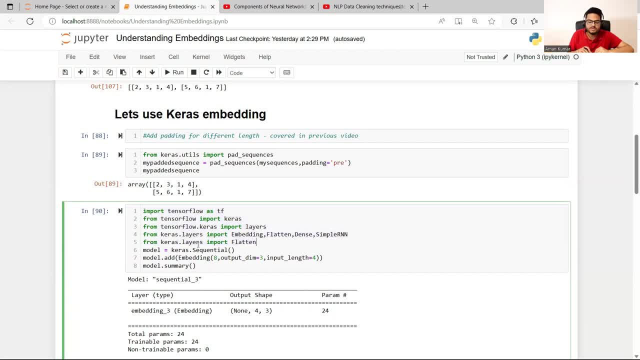 not using whatever I am highlighting, okay, just, I am using sequential model and I am using embedding layer. so, as you can see, just focus on line number six, seven and eight. whatever I am highlighting here from Keras, I am taking a sequential layer and then I am adding embedding. 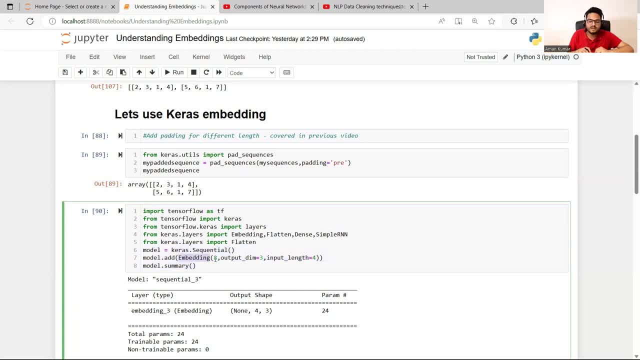 embedding, want to embed my input and then I'm saying it. why I'm saying it? because there are seven unique words in my vocab. how many unique words are there in my vocab? seven unique words in my vocab. so in Keras embedding you have to give n plus one, so eight output dimension. 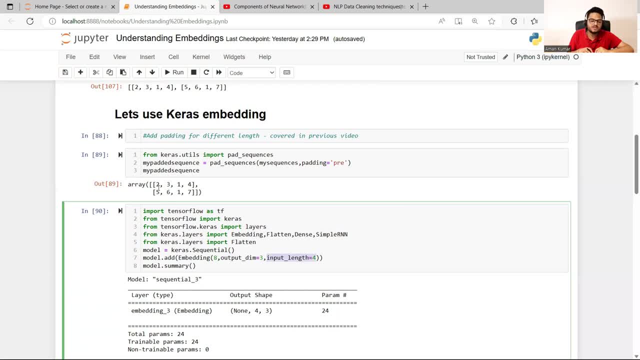 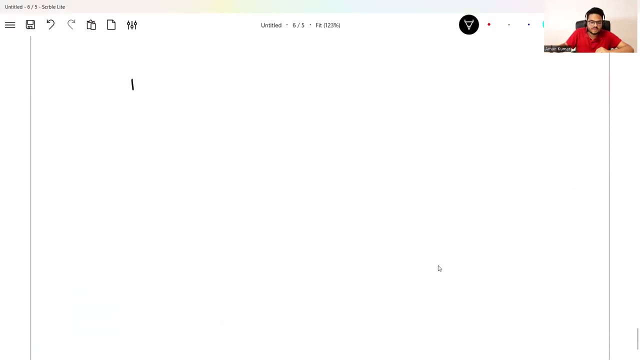 I want three, and input length is four. input length is what is the length of my, my each sentence. so here in this box, what I'm doing is I'm just padding. so what is the concept of padding? I will tell you, suppose. suppose there are two sentences, one is I M and other 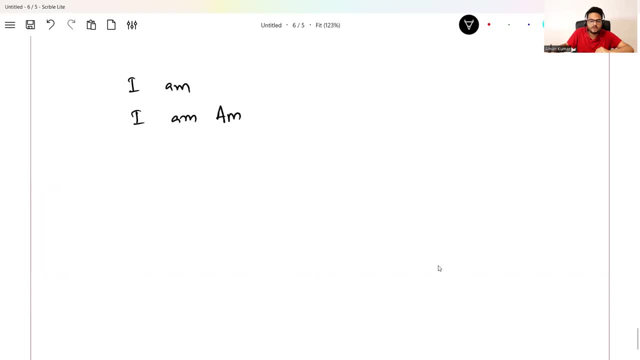 is I M Aman. okay, so when you send, when you convert this sentence to integer encoding or any kind of encoding right, suppose this will have 15 and image, let's say 16 number word. so this is the integer encoding for this right, and here suppose 15, and then I'm. 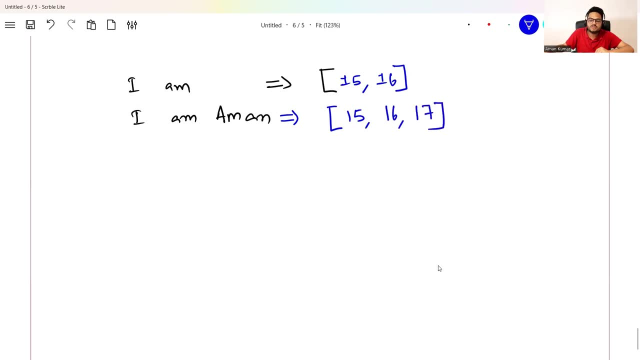 then 16 and then a manage, let's say 17. so this vector is of size 3 and this vector is of size. sorry, this vector is of size 2 and this is of size 3. I don't want that to happen because that will create problem in my machine learning. so I want both these vectors to be. 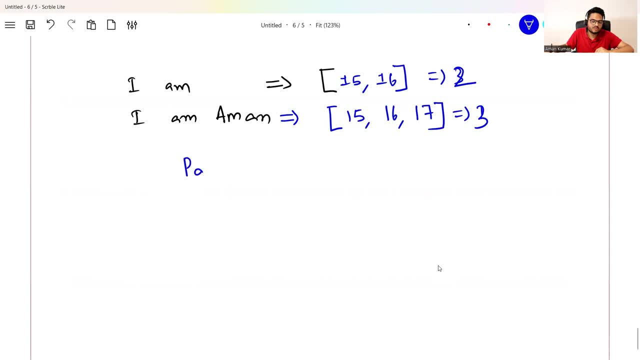 same size. for making it same size, there is a concept of padding. so what padding will do is it will add 0, just to make it a fixed number. for example, I say: make it padding is equal to 0 and add 0 in pre. pre means before this or post means after this. so then I will. 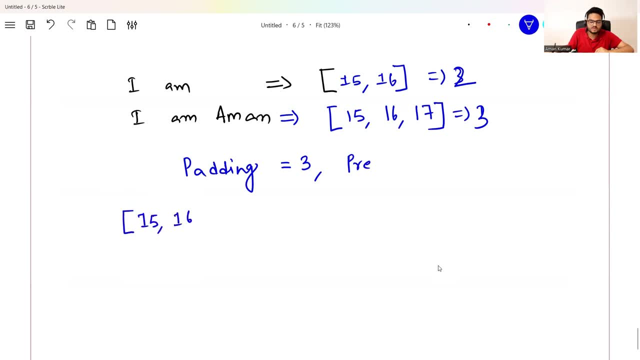 get two vectors: 15, 16, 0- this is my first sentence, and 15, 16 and 17- this is my second sentence. okay, so this is padding. what padding does? it makes your vectors equal size by adding zeros in front or in the back. so that is what I am doing here. from Keras utils import. 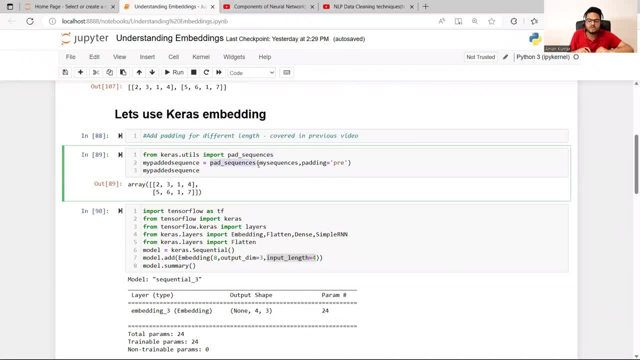 pad sequences. and I am saying: if some word is not in the same word, if some is not in the same you know length, then convert that to same length. but in this case both my words are for four numbers only. so this is fine. this will not do anything. now what I am doing, 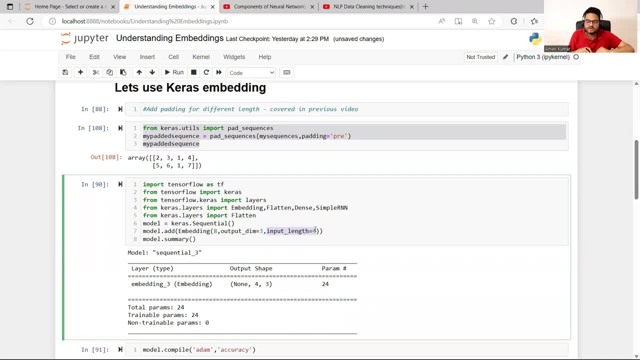 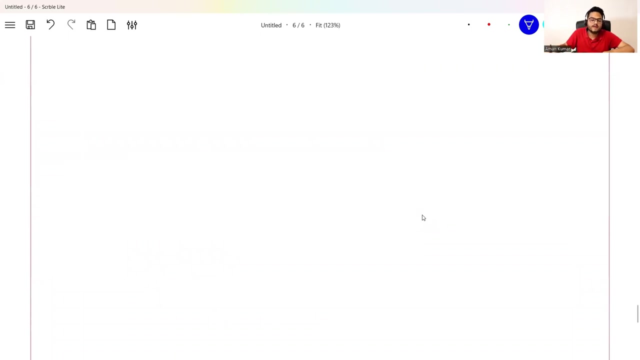 I am the same thing I am giving here input. length is equal to 4. so what I am asking to Keras is: take these input, okay, Take these input and give me an output of three dimensions. so let's come back to our our here again. so now what we have is: we have words, okay, and in our words we have how many? 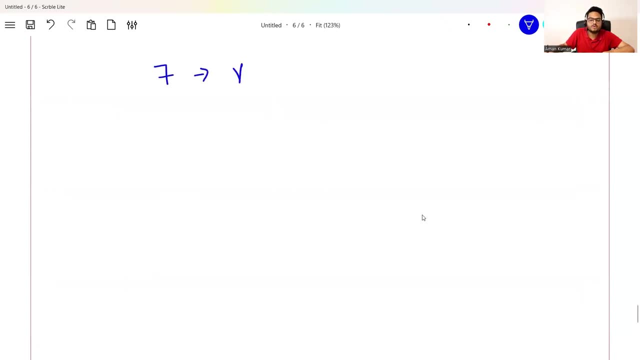 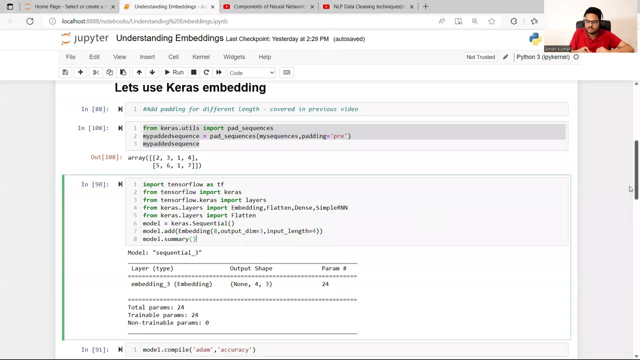 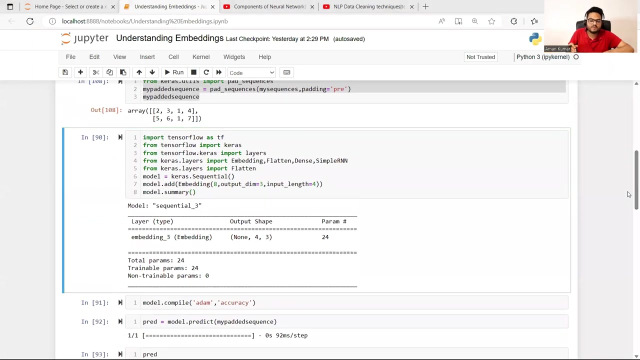 how many vocab seven. vocab seven is my vocab size. vocab size means how many unique words are there in your vocab. So if you come here right, One, two, three, four, five, six, seven, seven unique words in my vocab. so when the vector will be created, one. 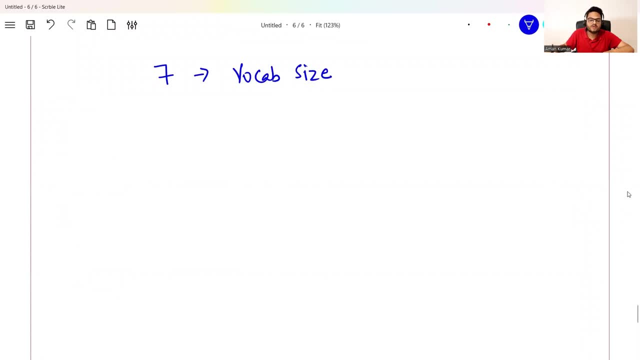 hot encoded vector will be created. then it will be created. how many entries will be there? for example, suppose, for cricket word i want to create a one hot encoded vector. so how many elements will be here? there will be seven elements, right, seven elements. so first element will represent, i second. 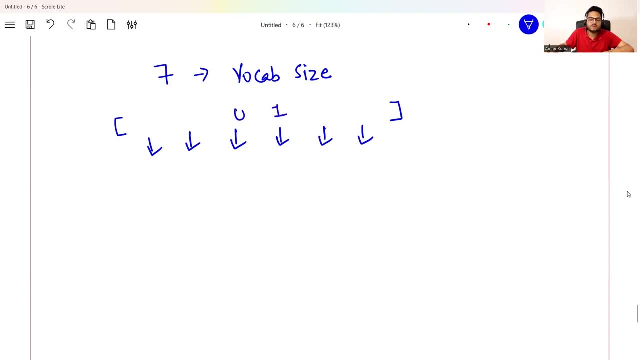 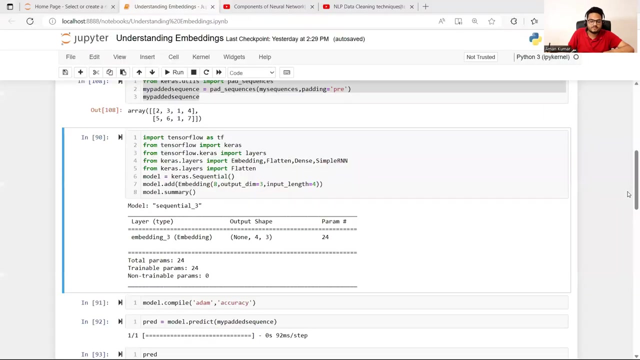 m like that. okay, so only cricket will be one, rest, all will be zero. so what i'm saying is: seven is my vocab size. so when my model will get created, the embedding model, it will look like this: one, two, three, four, five, six, seven, okay. and then i'm saying output dimension will be three output. 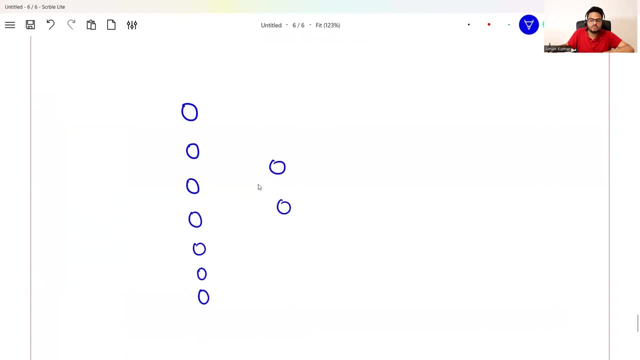 dimension will be three means one, two and three will be my output. so what i want to do, i want to create a one hot encoded vector and i want to create a one hot encoded vector and i want to create a fully connected neural network here. fully connected neural network here, where i am. 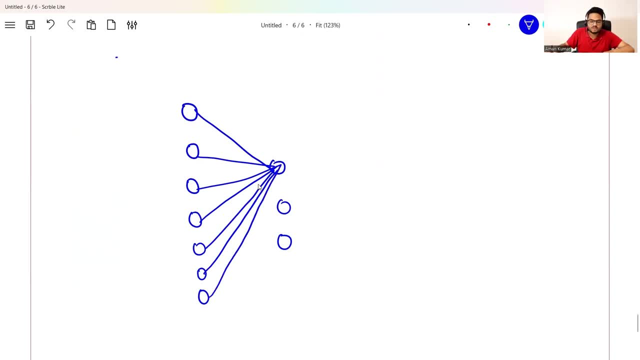 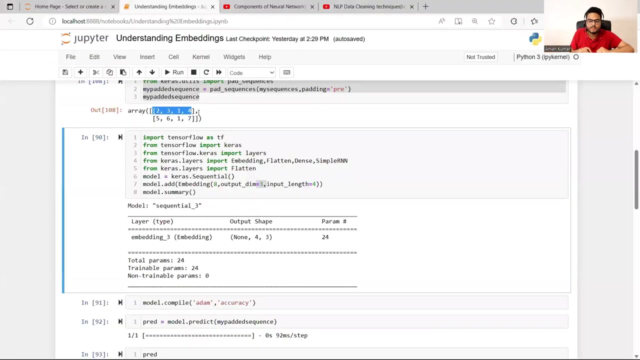 saying to keras embedding that take my word. suppose my cricket word looks like this: one zero, zero, zero, zero, zero, zero, seven. one, two, three, four, five, six, seven. so suppose my cricket word looks like this: now do not confuse between these numbers, numbers and this encoded number. so this is word number two. for example, my is word number two. so 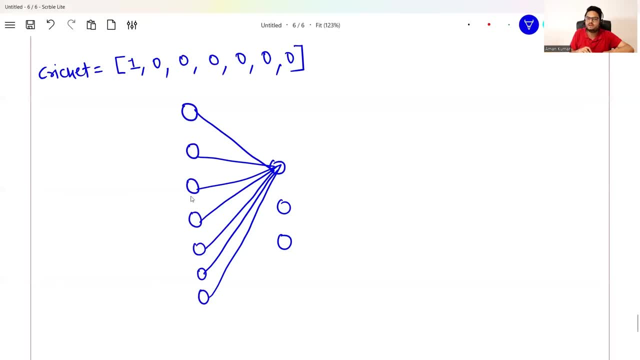 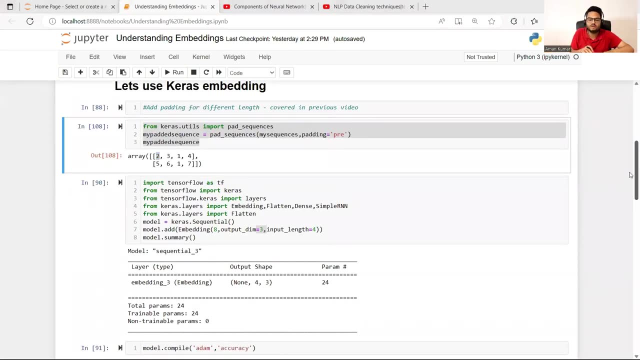 this encoding will happen internally, otherwise it cannot send it to the vector space. okay, so this encoding will happen internally. what you have here is one number for each word, okay, so one, two, three, four, five, six, seven. suppose we are talking about two word number two, right so? 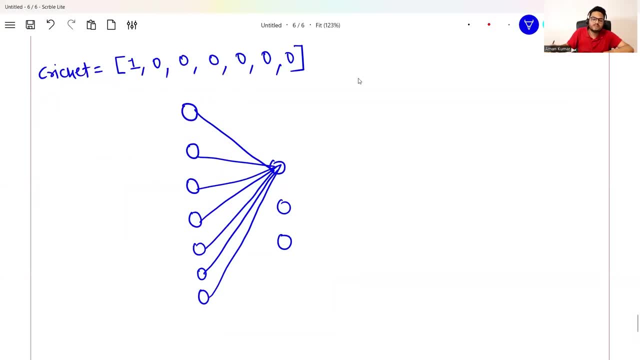 that word. number two will become one, rest will become zero. this goes as input to your embedding layer or this model in this case. and what i'm saying to keras is: give me a three dimension output. three dimension output is encode my word in a three dimension space, so three. 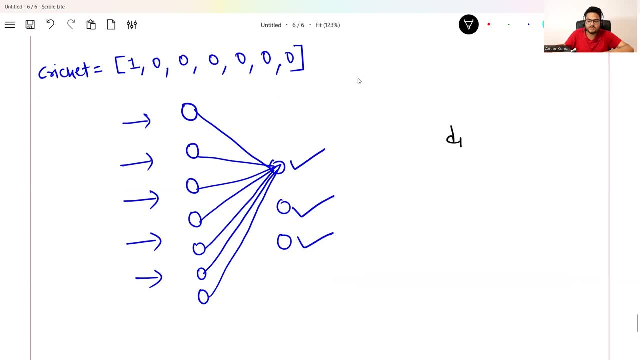 dimension space means it will be a d1 and d2 and d3. so my word cricket, my word cricket, will have some score on these three. so this score can be, let's say, 0.6 minus 0.4 and 0.2. 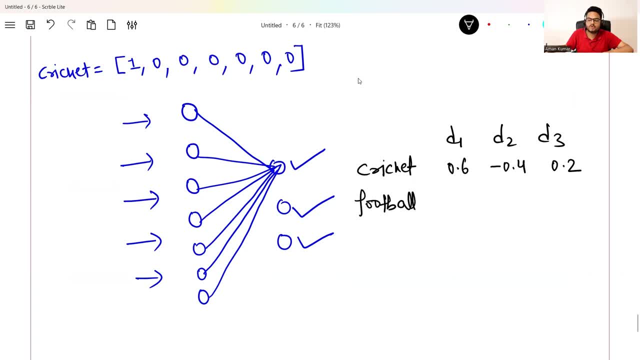 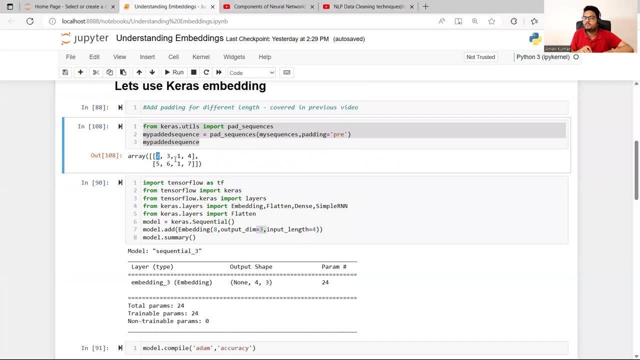 similarly, my word football, my word football, can have a score of 0.5 on this. 0.2 and 0.1, something like this. what i'm saying to keras is: take all my words, one by one, words which are encoded in integer format. remember this integer format words will be converted to one hot vectors before. 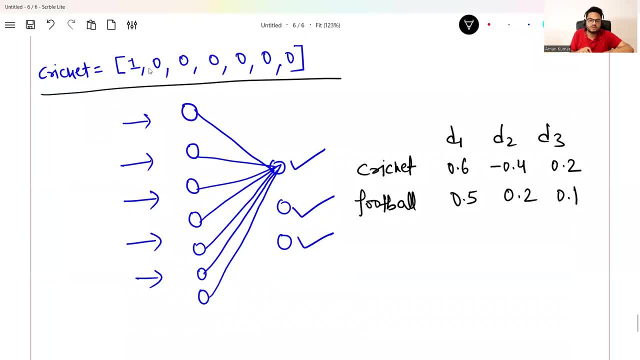 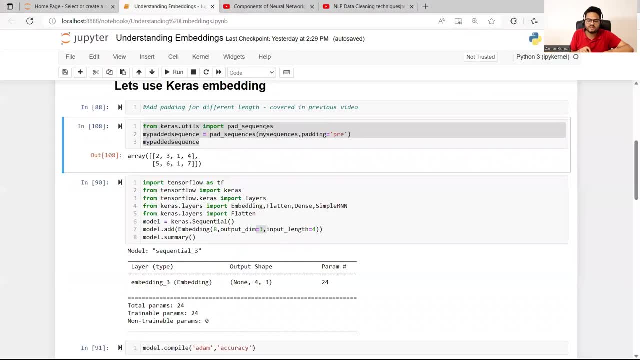 sending it to the model. so two number word only. this place will become one rest, all will become zero. that will be the result of this encoding. so this is the result of this encoding. so this is will be sent and the output. what you get is a three dimension output. okay, so if i run this, 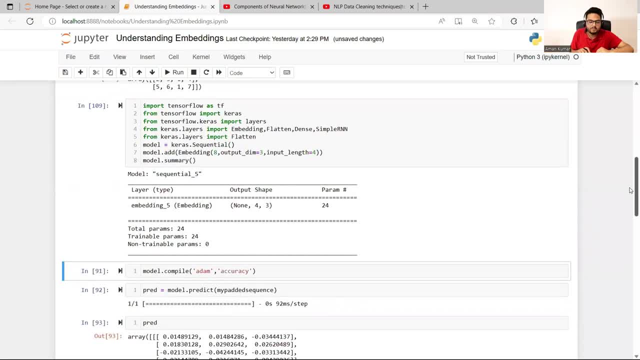 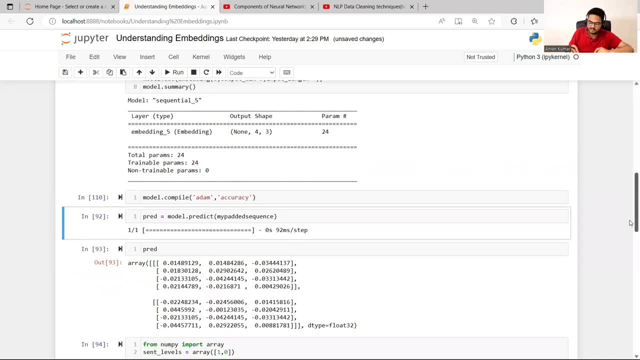 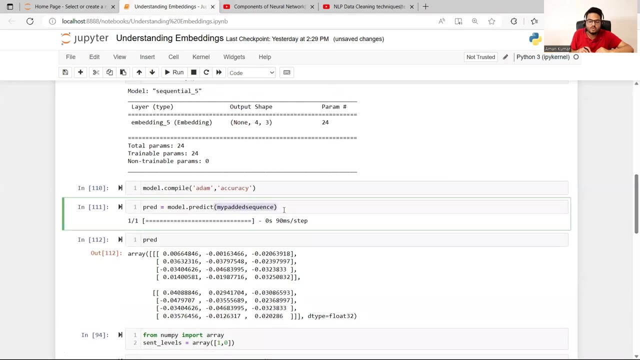 model here and if i predict- for example, i'm compiling this model and i'm predicting on my padded sequence- my padded sequence in same input data i'm predicting on. okay, if i'm predicting on my padded sequence, that is same input data. what you will notice. here is now my word number two. 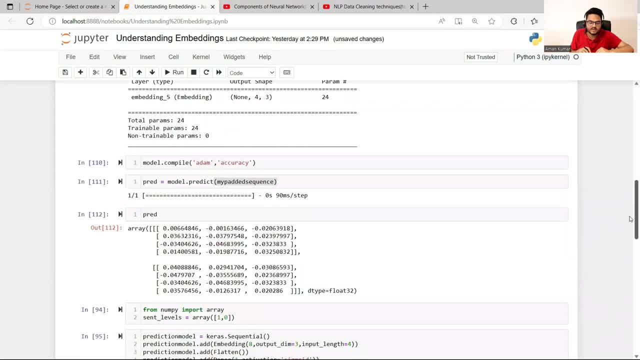 my word number two is represented by this. this is my word number two. okay, please pay attention here, guys. my word number two went to the model, learned the embedding, and when it came back after embedding, it is represented like this: okay, similarly, the next word is represented like this. so all the. 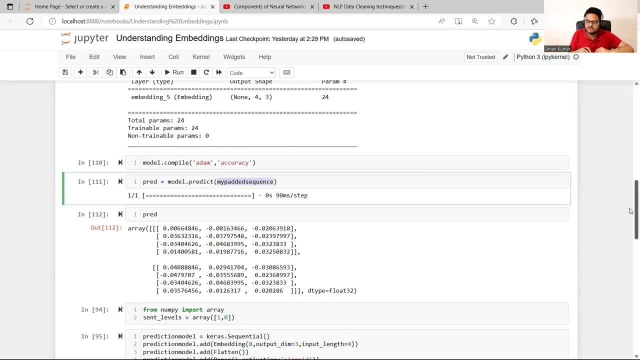 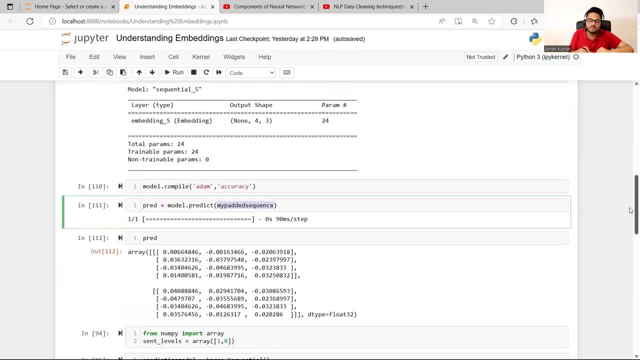 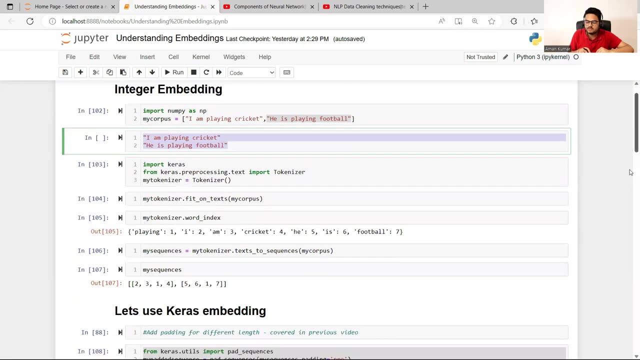 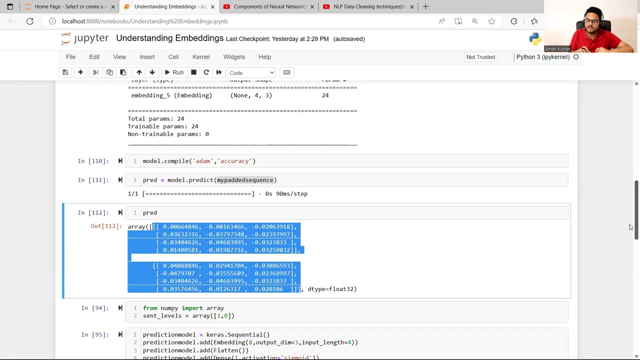 words in my padded sequence, which was there, on which model was trained only okay, has been converted into a three-dimensional numbers. now, your original sentence, your original sentence, these two sentences are these three-dimensional numbers. now, now you can take these numbers, you can train your model and do whatever you want. okay, before i train my model, i will explain you one more. 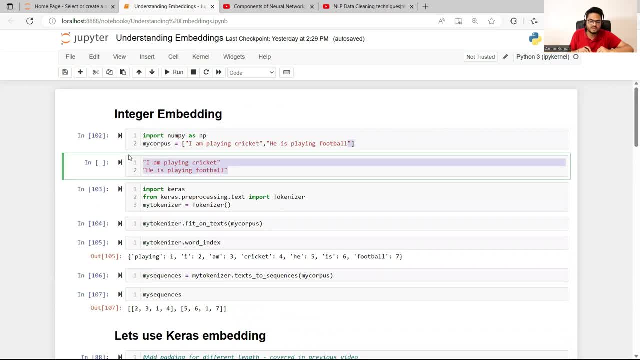 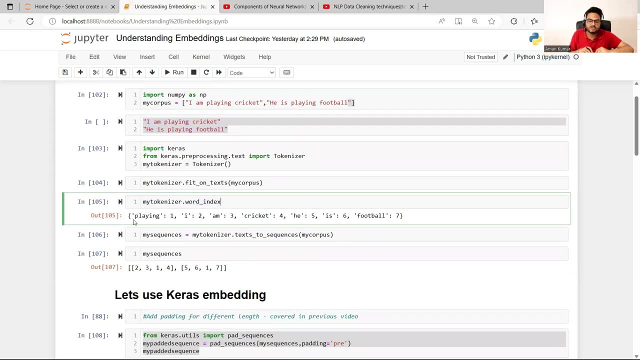 time. what has been done here? this is your original sentence. from your original sentence, what you did? you created tokens. tokens means individual words. you created tokens. tokens means individual words, words in those individual words, you assigned a number. for example, playing is first word, i is second word, m is third word, and so on and so forth. once this happened, then you said: okay, create a. 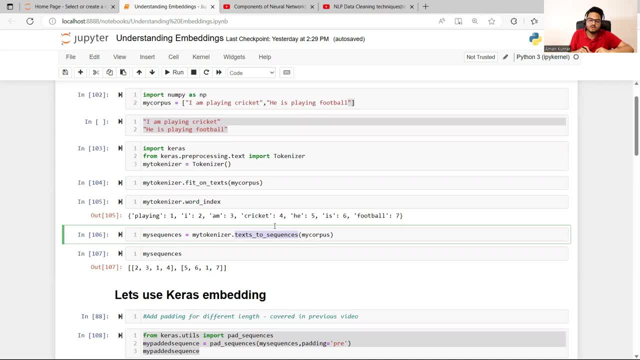 sequence from my corpus. now, the first sentence has been converted to a series of numbers because, you know, now system identifies that as a number. so i is number two, m is number three, playing is number one and cricket is number four. okay, now what i want to do is i want to. 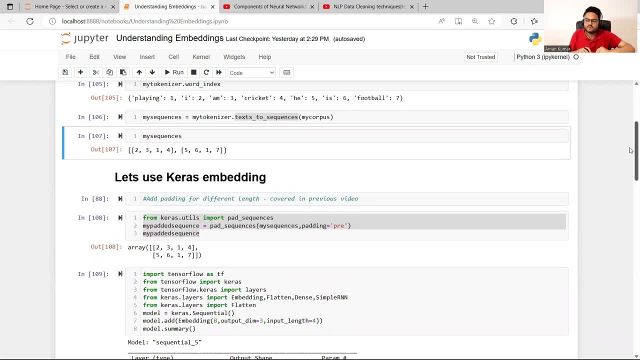 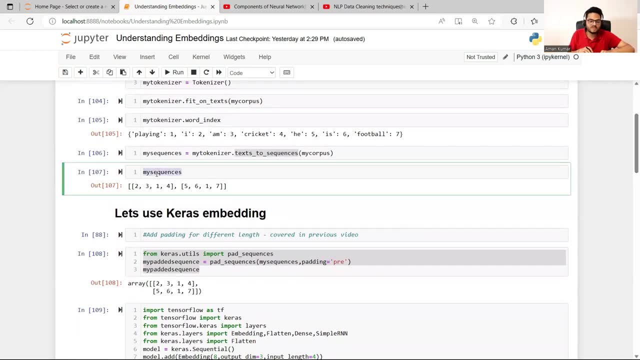 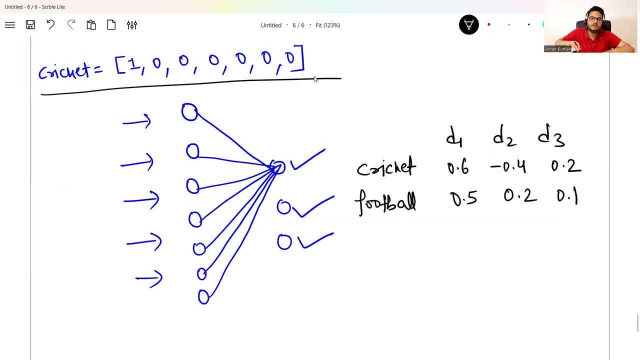 take advantage of keras embedding layer. so when i want to send this to keras embedding for one more layer of embedding, then if i send this, my sequence is right- then it will get converted into a one hot vector. all these words will be converted into one hot vector and those 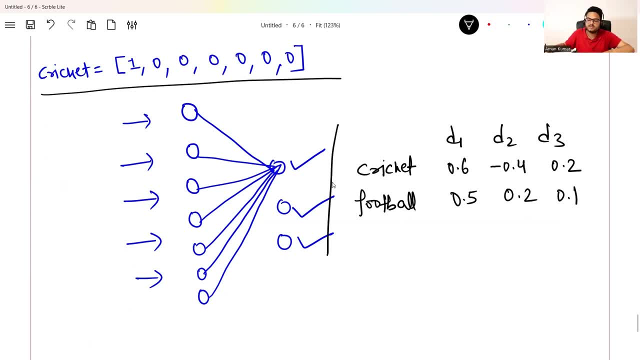 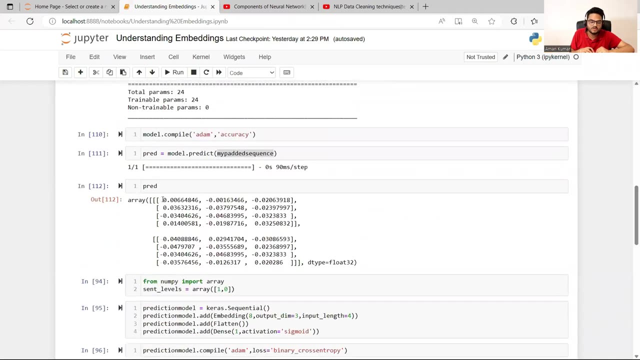 will be predicted based on keras embedding. so when the embedding results comes out, for all the word, i will have three, three numbers that i am trying to show you there. for all the words, i have three words, three, three numbers. okay, for all the words: three, three numbers. one, two, three, number for first. 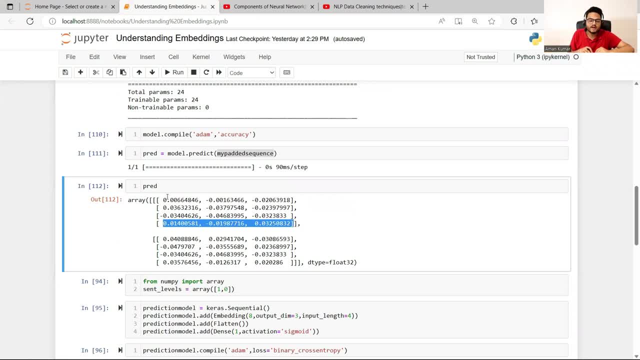 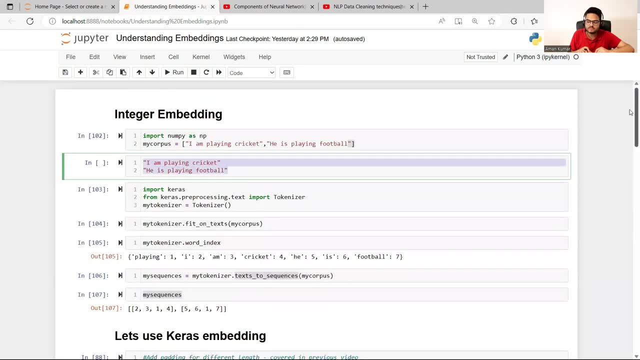 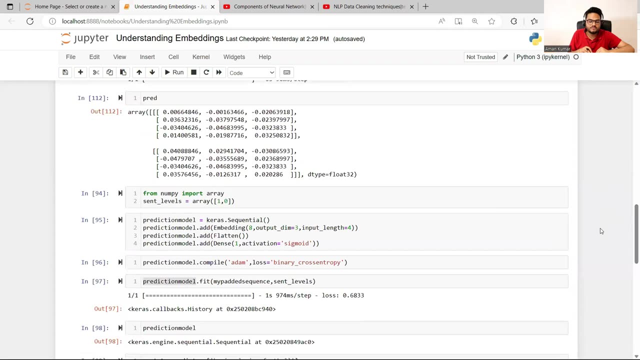 word, one, two, three, number for fourth word, and so on and so forth. i can take this data and train a model. let's do that. so till now, if you notice, i have not defined my target variable. i i'm solving this as a classification problem, okay, so here what i'm trying to do. i am trying to from numpy. 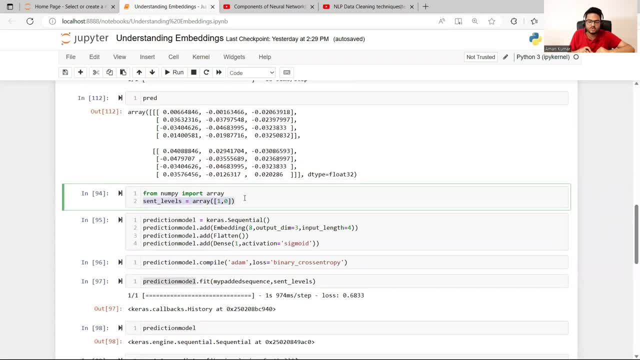 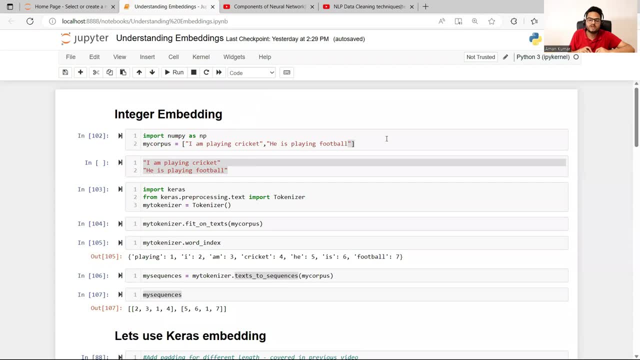 import. i'm importing an array and i'm calling sentence. level is equal to array one zero. array one zero means i'm trying to predict if a given sentence falls in the category of cricket. so one means cricket, zero means no cricket. okay, so i'm giving one zero. i will call this as is my sentence. 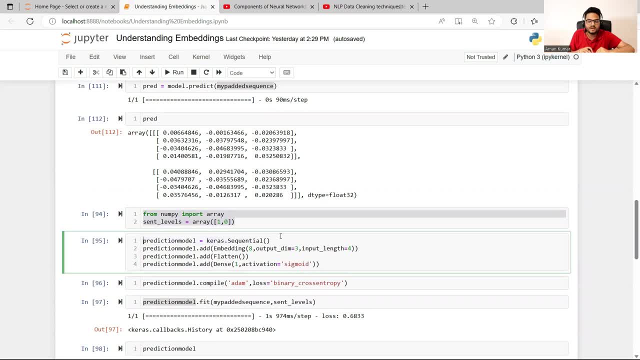 models. okay, now, if you see, here i'm again taking sequential. i am adding same way, the embedding layer that that i was doing above, and then i'm adding a flattened layer and this is a very simple basic neural network. if you have confusions, you can watch, you know. components of neural network video. 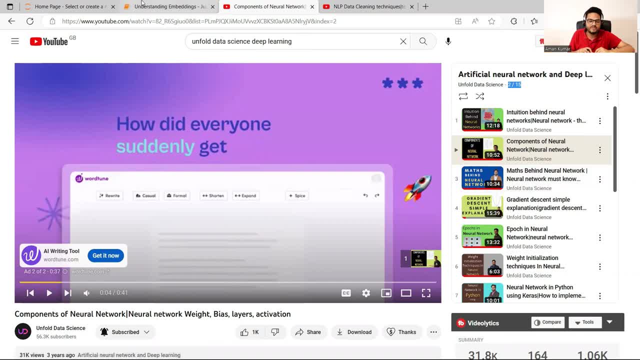 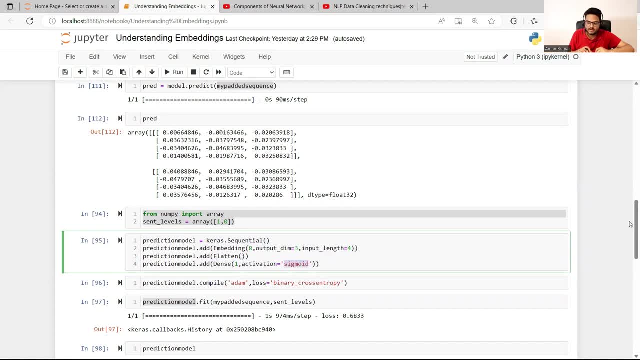 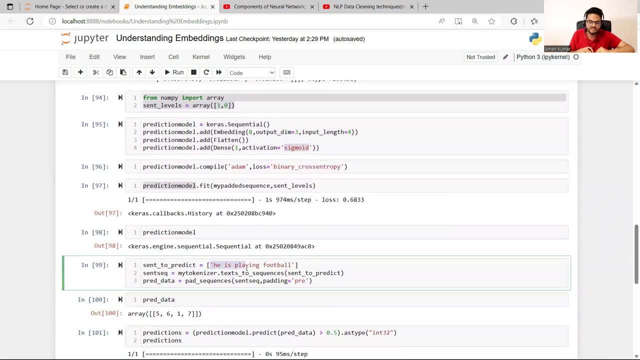 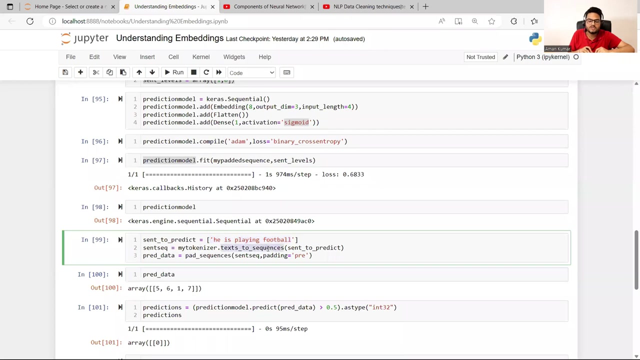 it will be very, very clear to you what i'm doing here. very simple: neural network and sigmoid, because this is a classification problem, so training this neural network. and then here, if you see, i am taking a new sentence. he is playing football, okay, and this new sentence has been converted into a sequence using same tokenizer. 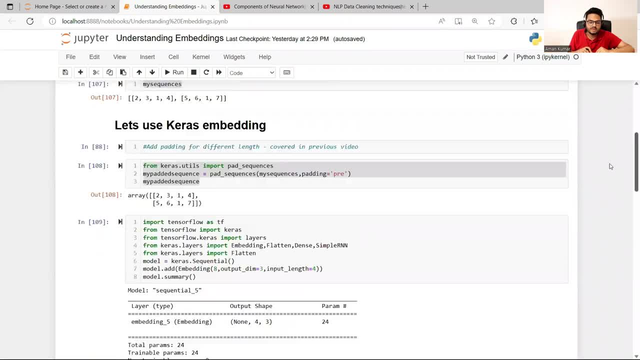 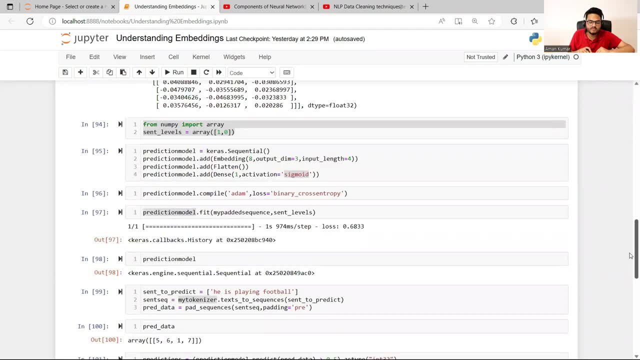 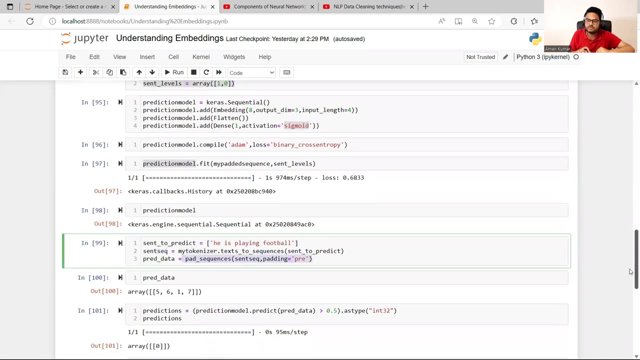 that we did above. so if you see here the same tokenizer that we used above, my tokenizer right, using this tokenizer only i have converted my sentence into sentence sequence and then i have padded because i want to ensure it's a free uh for four thing, for character thing, and then i have 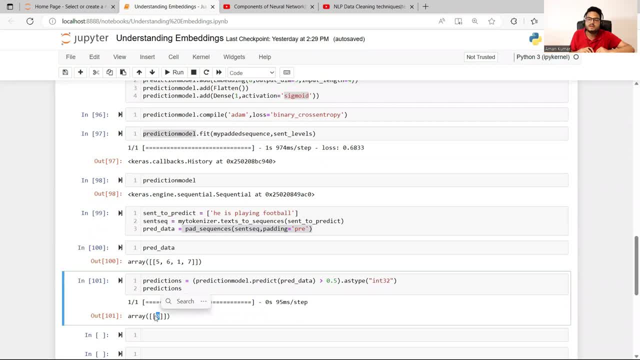 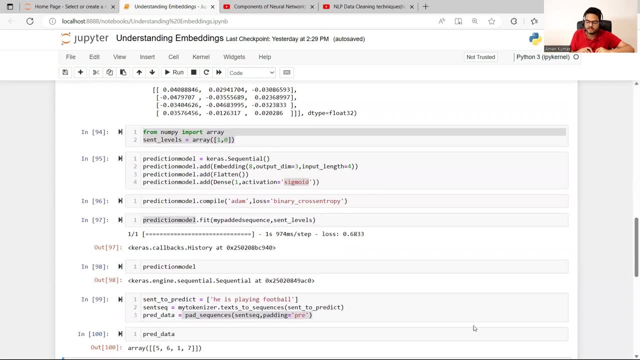 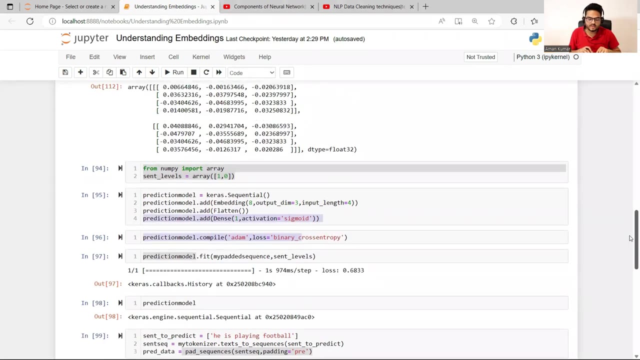 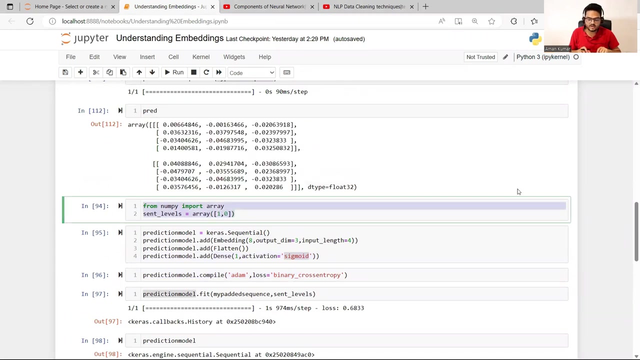 predicted and if you can see here, my prediction is zero. zero means it is not cricket, because my input line here is: what is my input line here? my input line here is: it is football. okay, so what i did in this model up to here, i created my text into numbers, then i added a label because i did not had in the beginning. 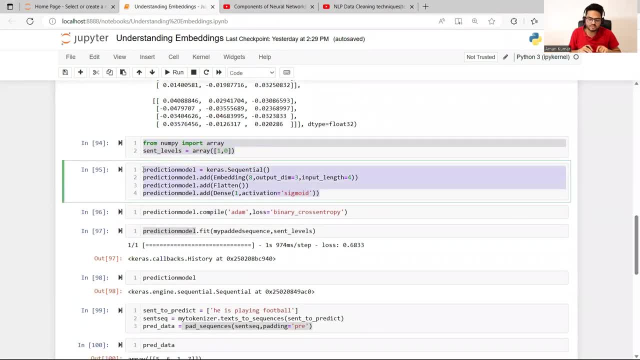 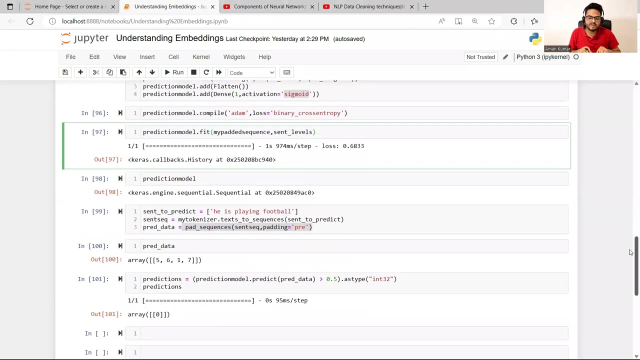 and then i defined a neural network model with one, just one embedding layer, one flattened layer, and target is dense. because this is a sigmoid, because this is a binary classification problem, i compiled my model and i just fit my model and i am predicting with a new sentence. my new sentence is: he's playing football. 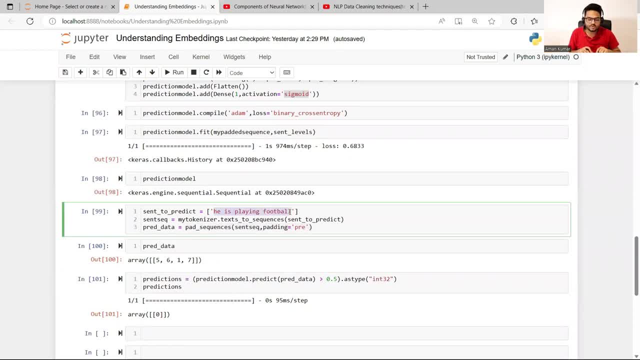 on this new sentence: i am predicting. when i am predicting, i am getting my prediction as zero. zero, because this is not a cricket related word. okay, and here all the pre-processing that i am doing, it is based on the pre-processing what i did in the training data. so what is this is a simple. 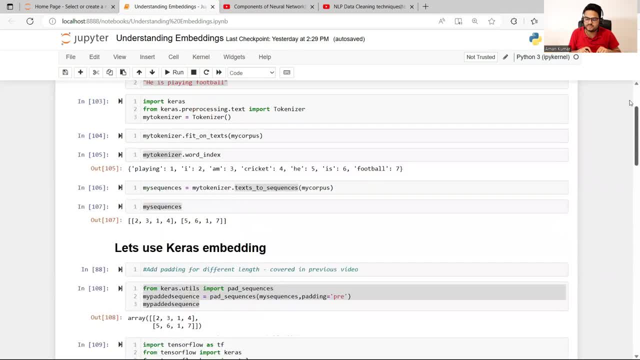 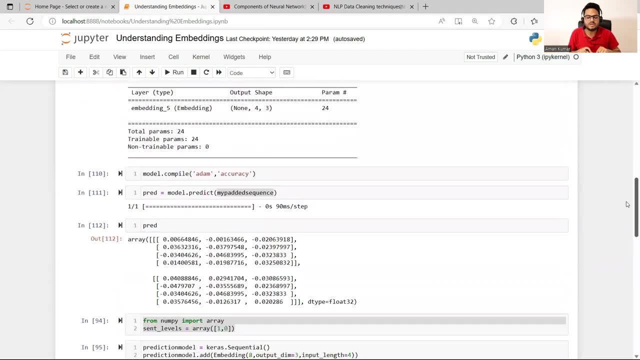 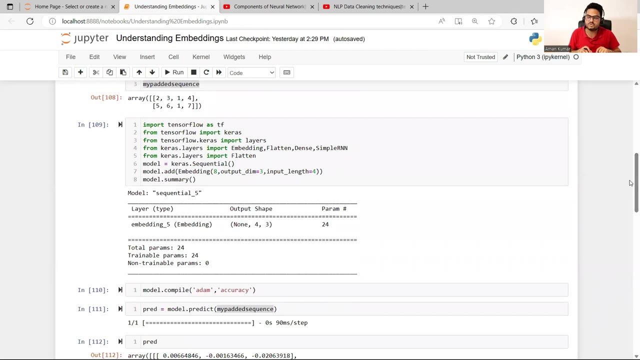 classification problem that i solved in four days, front of you, using simple, most basic neural network. okay, most basic neural network. using that, i solved a simple classification problem. now my question to you, first question to you, which i want you to write me in comment, is why total number of parameters and total number of trainable? 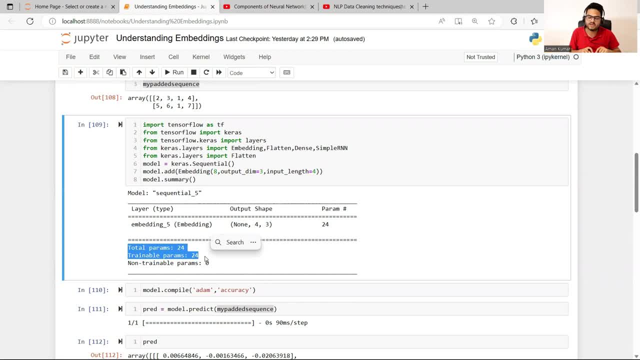 parameters is 24 here. that is the first thing that you have to write me in comment. okay, think on that and write me. if you understand the neural network architecture, you will be easily able to explain me why that is 24 only why not something else? okay, you have to explain me in the comment. 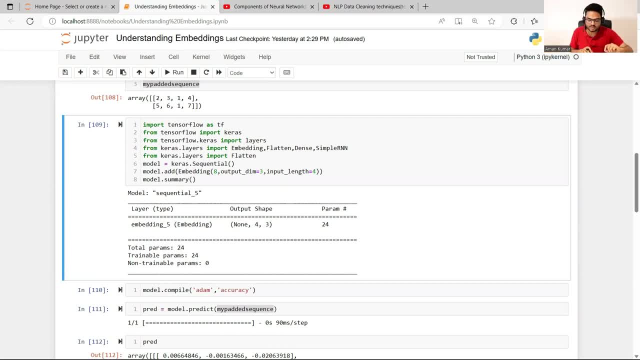 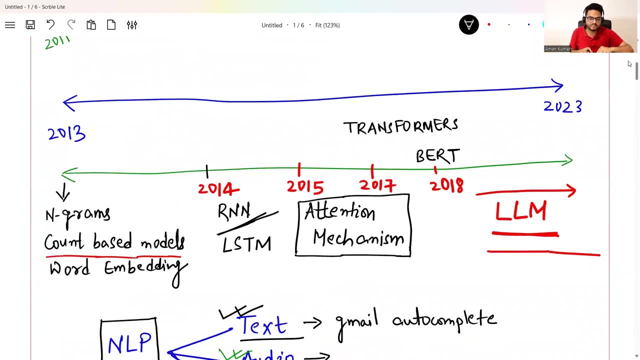 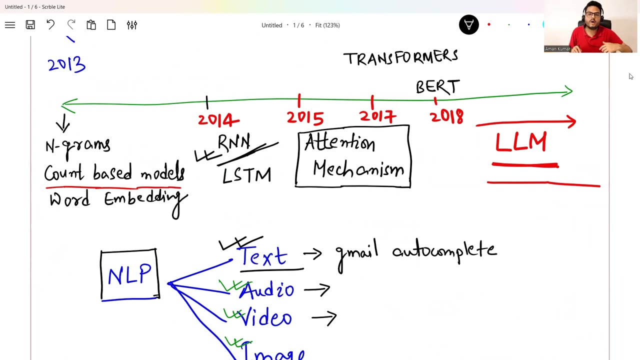 then, second thing that i want to capture here: i want to go back there and try to explain you that we have covered everything up to word embedding, okay, so, which means that we have covered everything up to whatever happened before the world of rnn. so why rnn came into picture, what is the use of rnn- we have all these techniques. then why rnn has come into. 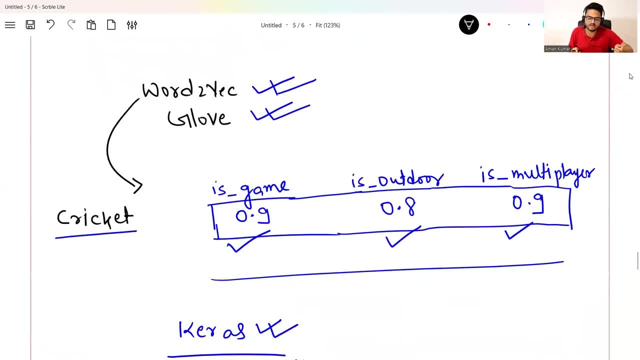 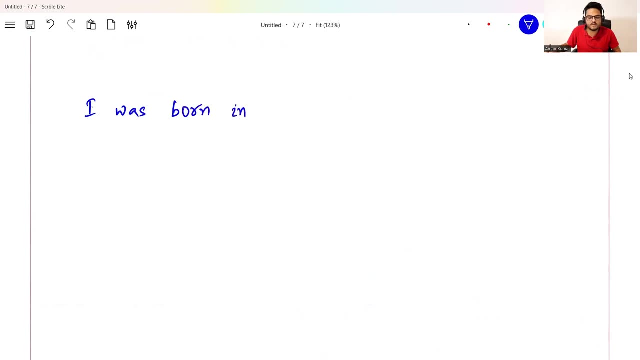 picture. so i will write here one word, okay, one sentence, and then we will think together. for example, i write here: i was, i was born in germany. i was born in germany and hence and hence can speak blank. so what do you think will be here in the blank? 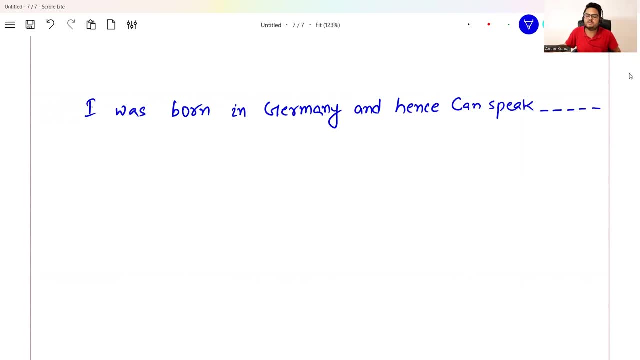 obviously you and me are human, so we can simply think it will be german. okay, because somebody is born in germany, so he or she can speak german. how did you come to that conclusion? because whatever was written before this, but if you are using this memory, right, you went backwards and you understood what was said before. 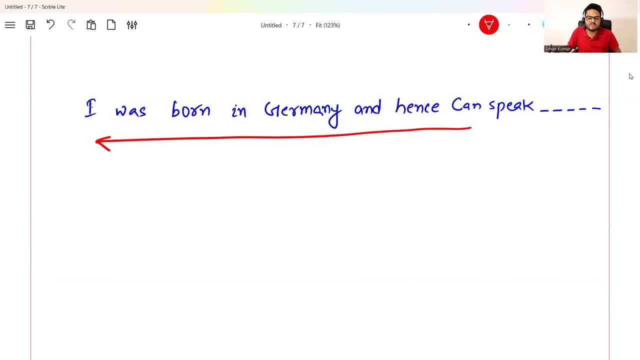 what was said before is: i was born in germany. okay, and this information- i was born in germany- was useful in determining what will be the next word or, in other way you can say in useful in understanding the context of a given line or sentence. okay, in none of these models. 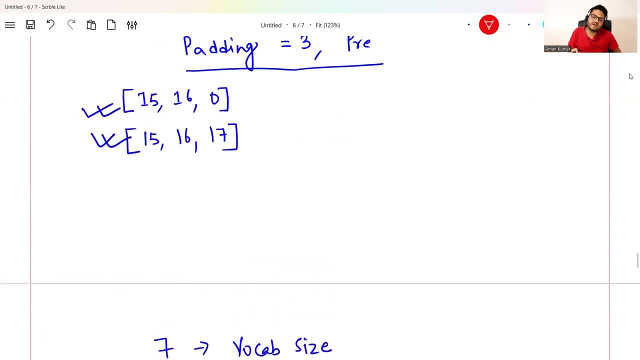 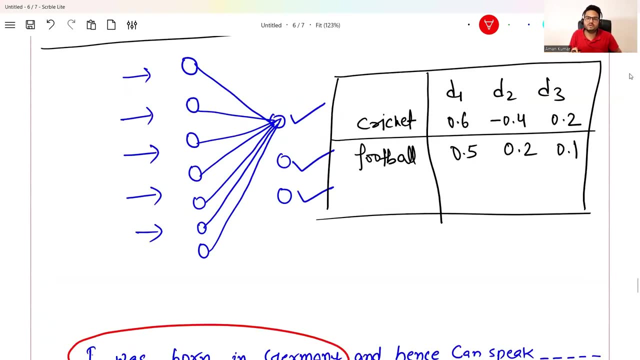 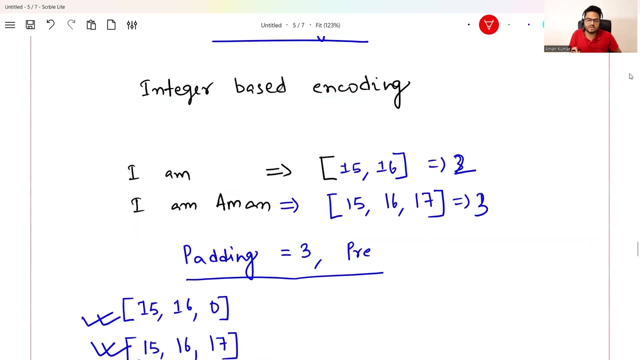 in none of these models- there are several we have discussed till now. whatever kind of word embedding we have done, whatever kind of advancement we have done till now, we don't have capacity and capability of remembering what happened before. for example, in this sentence there are four words: okay in integer based encoding or any encoding you. 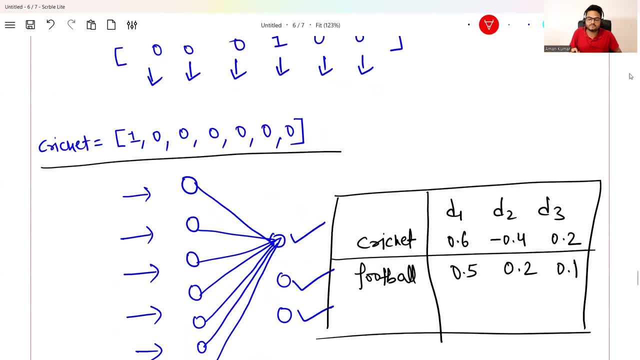 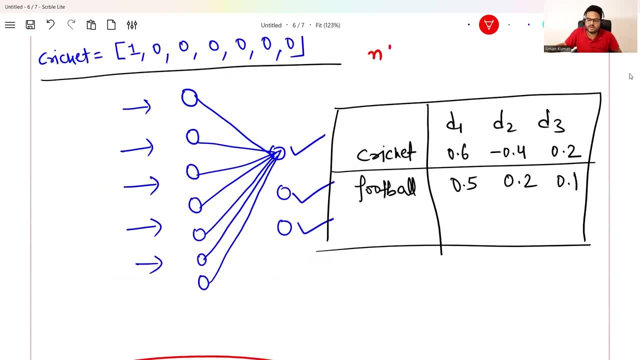 do right. all these words will go and all these words will, you know, prediction will happen. so one n-dimensional array will get created. one n-dimensional array will get created, which we call tensors also, that will go as the input in any neural network and output will come and then 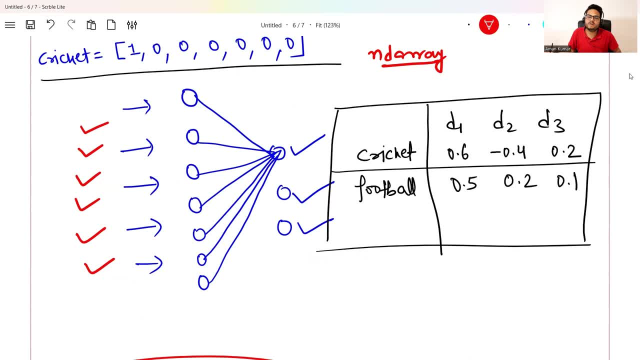 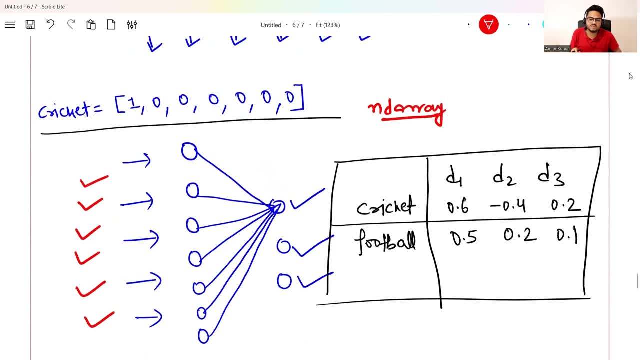 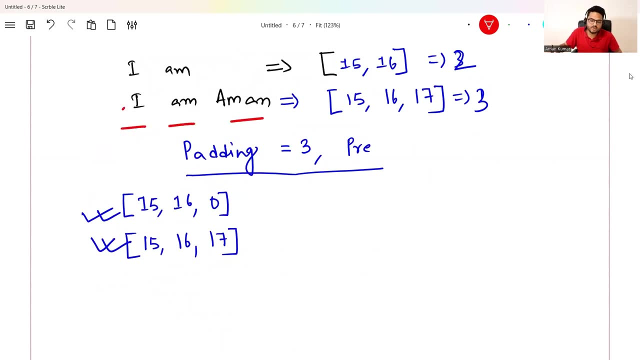 the loss will be optimized. that is how it will work, but there is no way the previous information can be captured or stored or memorized. what is meant by previous information is, in this case, suppose, the. the sentence is: i am aman. i goes a as a word vector. aim goes as another word vector. aman goes as another word vector. 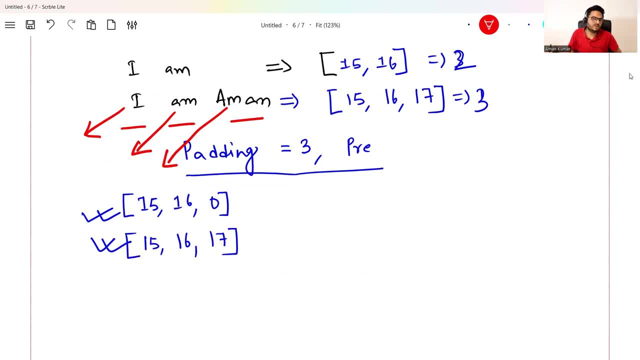 but there is no way in a normal artificial neural network that i can remember when i, when i reach aman, first of all, all these things will be processed together only so there is no, no time to reach something. okay, but suppose when i reach aman i don't have any information about what was. 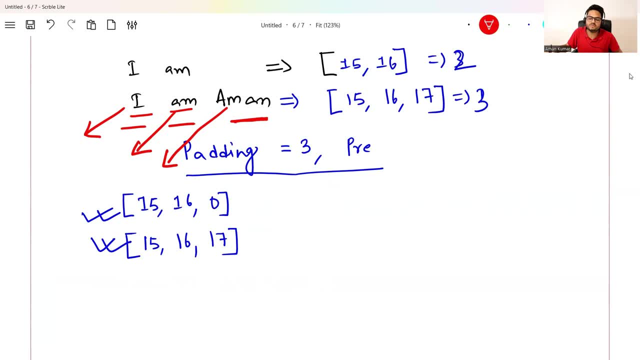 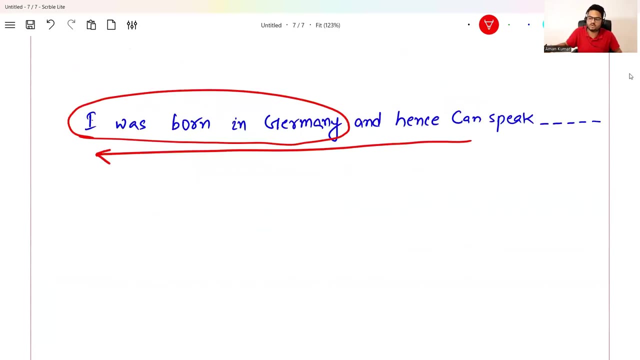 before aman, and if you don't have this information, what was before amon among then you know, understanding what can happen after that or understand the complete context of that, becomes very, very difficult. that is one problem with all these approaches that we have done till now. what is the other problem? so I'm writing another word here for 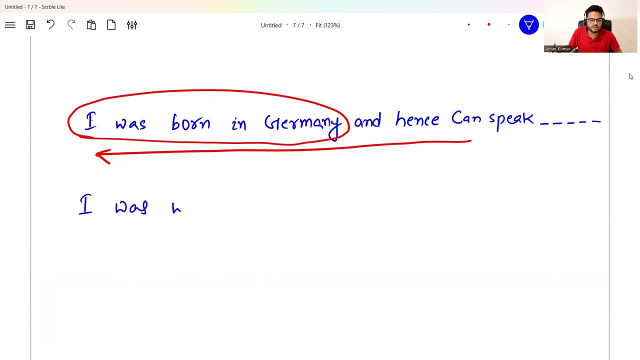 example, I say I was, I was walking, I was working on Bank of the River- okay, or this is one my favorite I will take: okay. so, for example, I can say I work at Apple- okay. and here I say a I eat Apple. now, based on the context right, the meaning of what Apple is changing a lot. 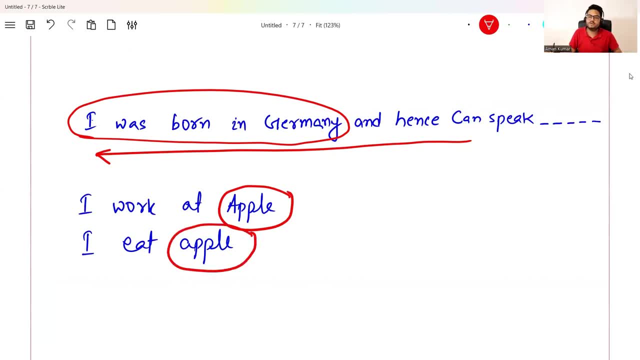 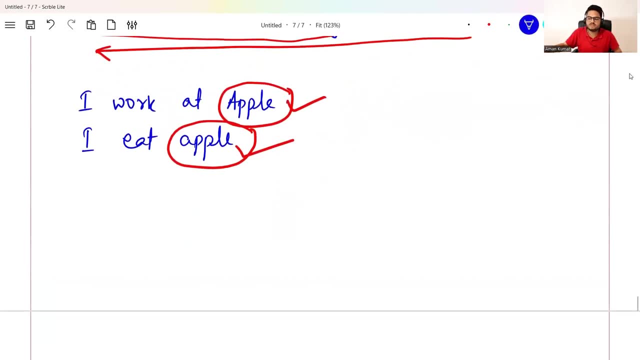 so another example of how the context, based on the context, the meaning of the sentence and word changes. and then there are some sentences where there is confusion, there is a differential ambiguity. you don't understand what this sentence is. for example, chicken. chicken is ready to eat now. whether chicken is ready to eat something or chicken is cooked to eat, we don't know. 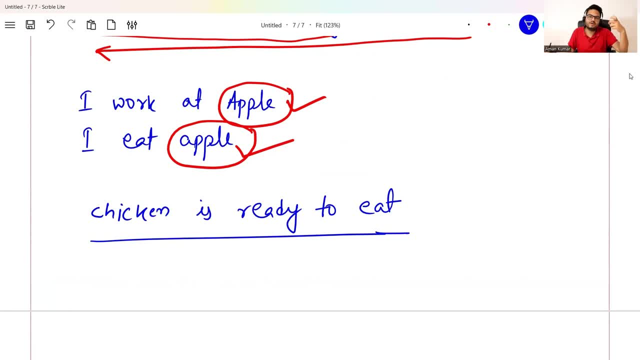 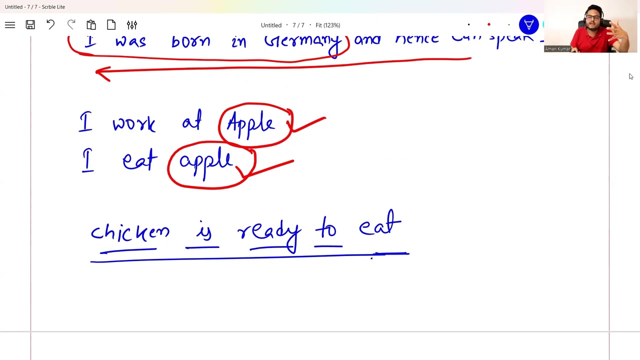 that. so understanding the sarcasm, understanding the, the context of a saying sentence in a given given scenario, right. all these things can be possible only when you remember the previous words in the network. so scientists and researchers had to find out a way to remember what happened before, remember what was said before and keep that information in the network. 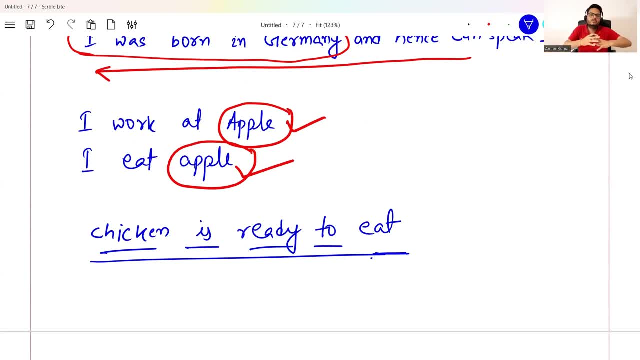 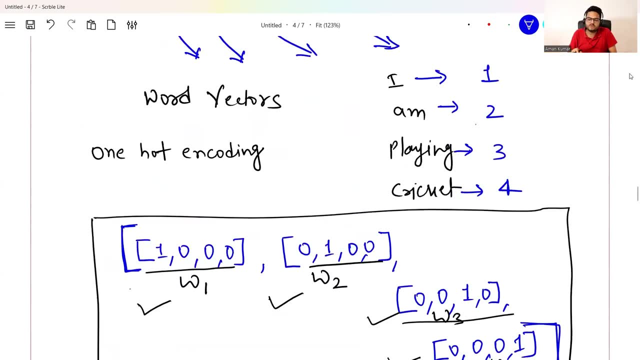 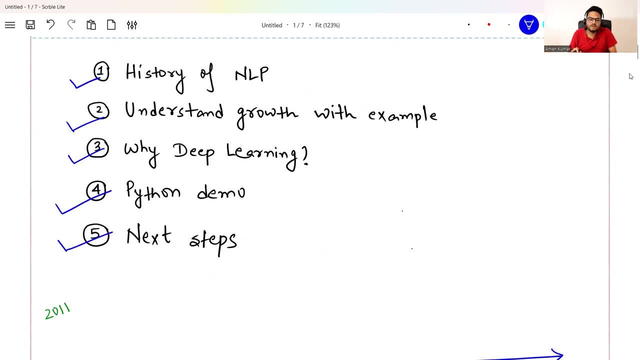 so that by looking at that information you know, the better predictions can be made. and that is where the born, you know, the new type of neural networks was born, and that is known as recurrent neural network or Rn. And and okay, so that is where the new type of neural network was born in 2014, especially. 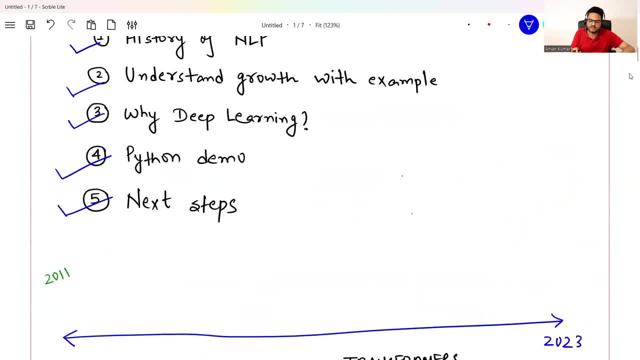 for sequential data. so whatever data I kept I discussed now came into the category of sequential data. for example, a sentence: right, I am Amman, okay, living living in this justice. so if somebody knows where Amman lives, they can fill this sentence. so this is a kind of sequential data where next thing depends on previous thing and Next thing. 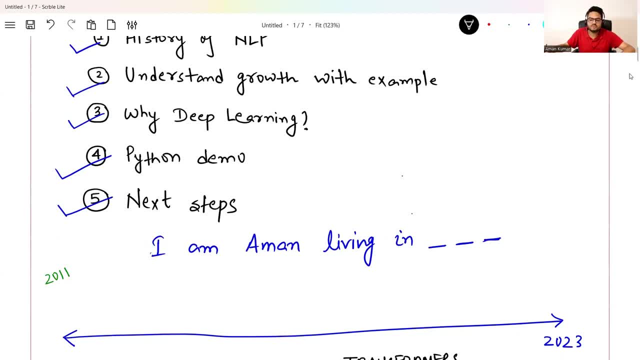 has a relation from the previous thing. okay, and suppose you want to predict stock market data, so maybe maybe some stock prices, let's say 12, 120, 12, 15, 12, 30 and then 11, 18 and then 11, 20 and then 12, 15. so what will be the next prediction? it will depend on the previous. value. so this, this kind of data, is called sequential data. so you can use a sentence or you. you can use many different numbers for this type of equation. for example, if you have a period of time which will last long, you want to go and calculate it. if you have, 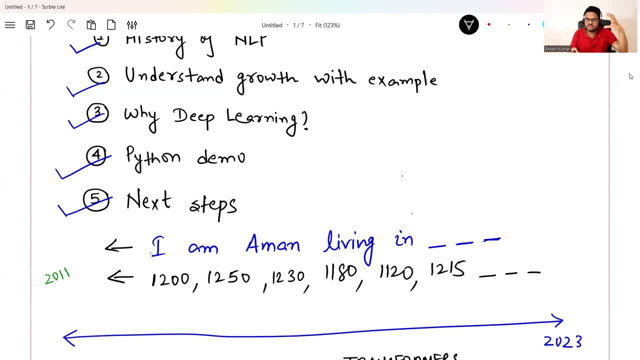 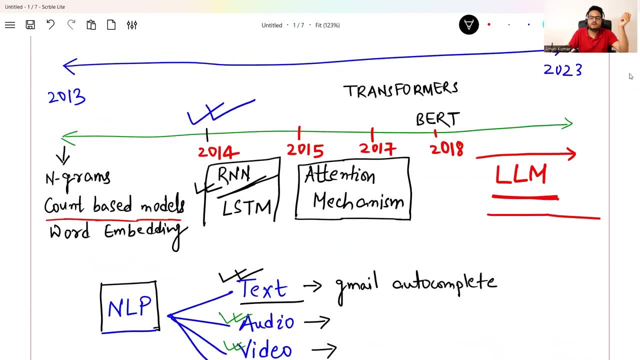 the previous value, you know what's going on in that period. you can do it with the previous. so to solve the problem of sequential data and to memorize the information there was. this architecture born RNN, and another variant of RNN is LSTM, so I am going to cover in my next video. 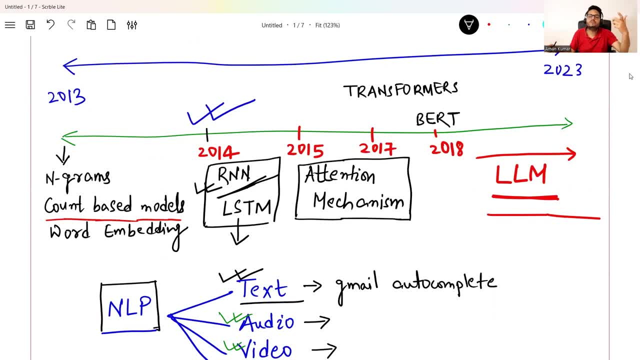 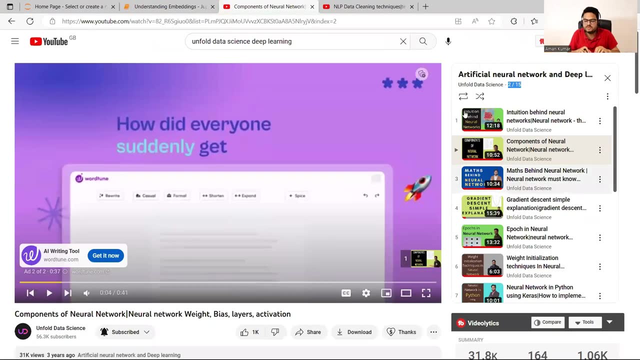 the architecture of RNN and how RNN works and how it is used in the deep learning and in sequence models, and then we will go on to the advanced topics. okay, so what you have to do, guys? I showed you two playlists here. one is artificial neural network basics. if you don't know basics, it will. 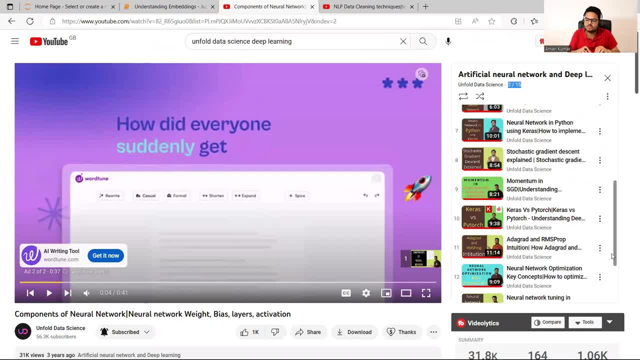 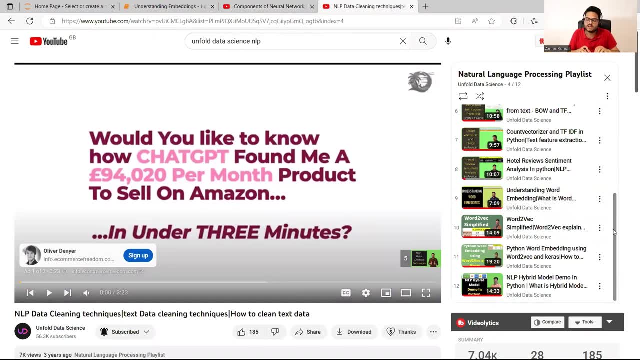 not be easy for you to understand advanced topics. okay, so just go through this and understand the basics well, and NLP basics like data cleaning or word embedding or word vectors and these things I covered. but again, go here and see which videos you want to see and which videos make sense for. 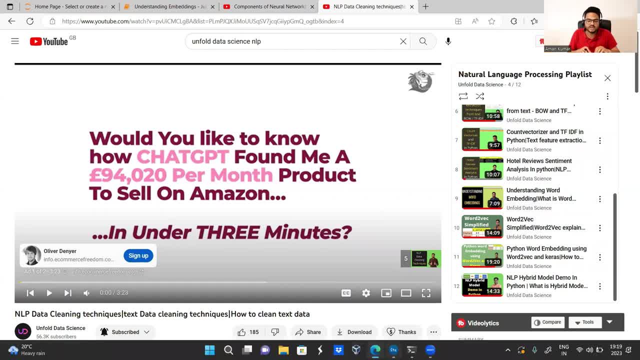 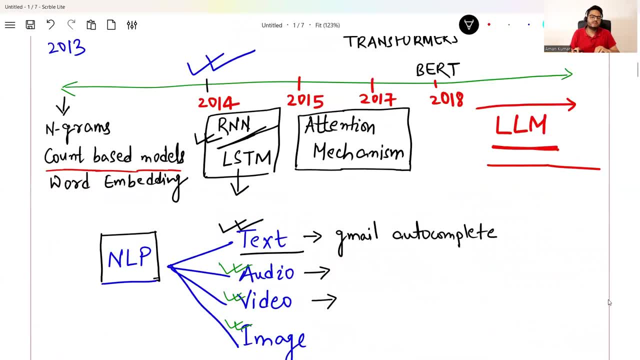 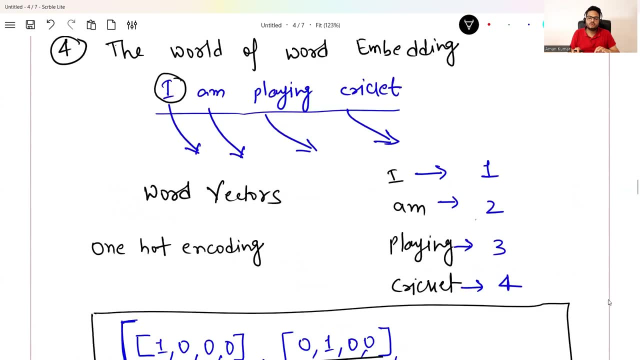 you watch those videos? okay, just to recap, what all we covered today is a brief history of NLP till RNN. okay, different techniques from the beginning, what from wordcon to TFIDF to ngram by grams, right to word embeddings, to different types of word embedding, and then why word embedding is not that great. 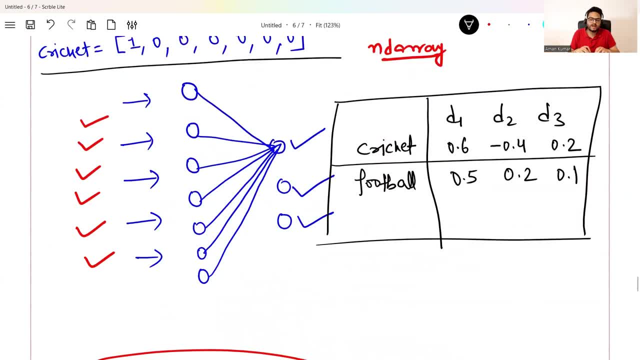 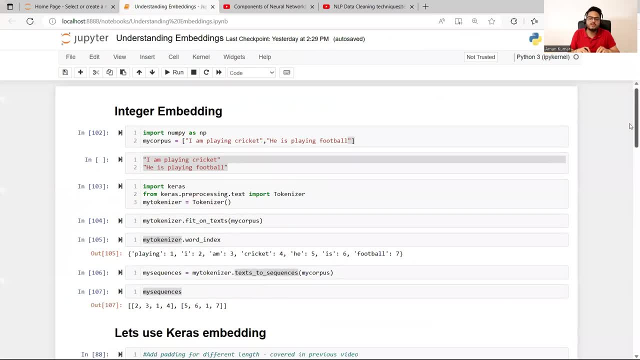 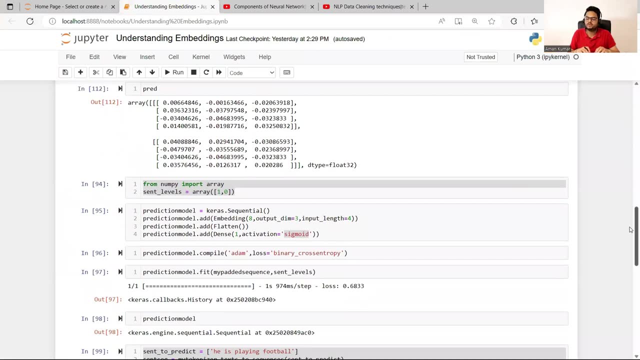 and what is? what are the problems with word embedding? what is padding? and I showed you a sentiment analysis use case of word embedding using very, very simple sentiment analysis use case using integer embedding, keras embedding. we solve that use case. so please let me know what are your questions and how did you like this video, guys? as always, your comments. 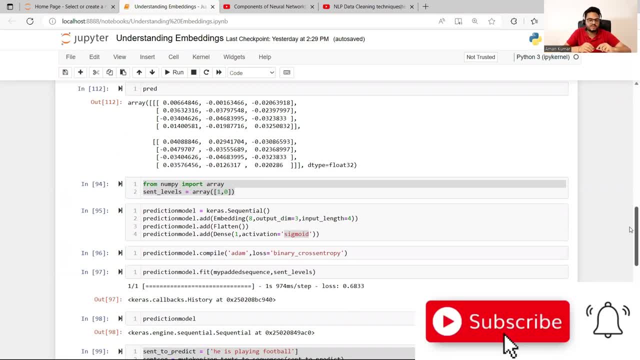 are my motivation, so please keep commenting and, you know, press like if you like this video. see you all in the next video. guys, wherever you are, stay safe and take care.